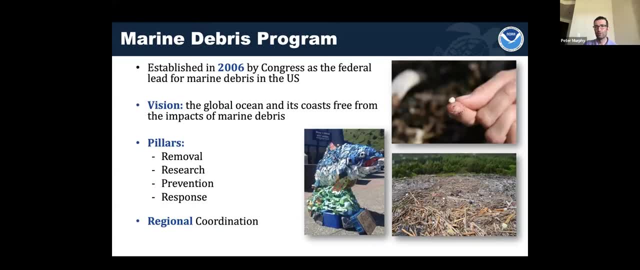 And then drilling a little bit more into the Arctic. So first a little bit about the marine debris program. So we're the- we were established in 2006 by Congress as the federal lead for marine debris in the United States. So we're a relatively young program, you know, coming up on 16 years. So I guess we can. we can drive, but in the US but only with a graduated license, depending on the state. 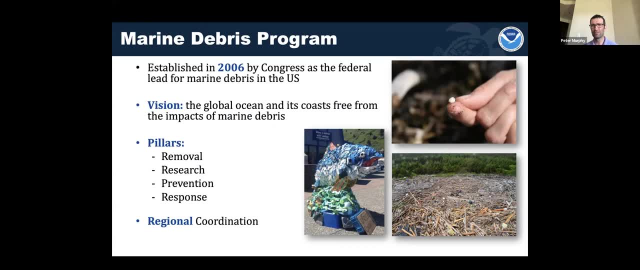 But anyway, I think that one of the things I note is that, while we're designated as the lead, what we see our role as- both me personally and I think us as an office- is to really facilitate the overall marine debris community that exists both nationally and internationally. 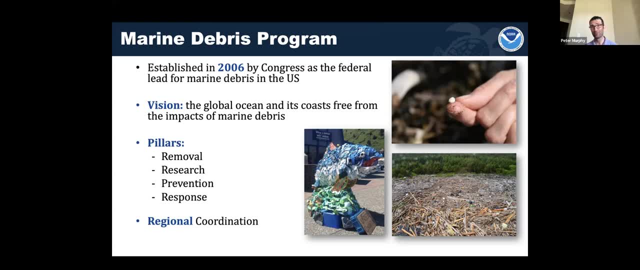 You know, I'm really happy to say that that community has grown a lot over the years. A lot more people are interested in and understand and are engaged with the overall issue of marine debris, or ocean plastics, or marine litter, depending on how you phrase it. 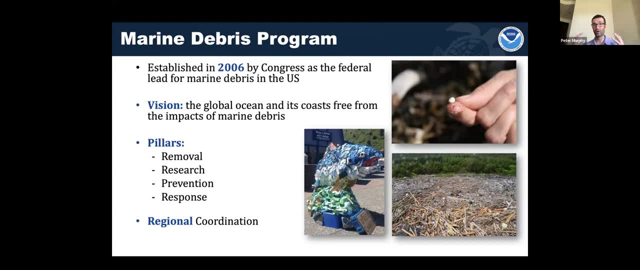 But we view it as our role to help, support, to try to facilitate, And so you know we don't see it as us being in charge of, or we see ourselves as part of, a community, But we just get to have marine debris as our first job. For a lot of people, marine debris is their second, third, fourth job. They have other issues that they're focused on. 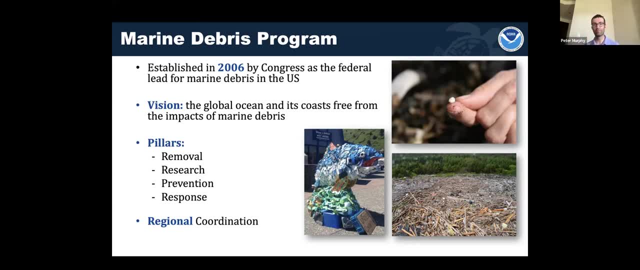 whether those are resources, habitats, other topic areas, whatever it may be- And then they come in and do amazing work on marine debris and then move move on or keep in the community, whatever it may be, But we just get to have it as our primary focus. So obviously the vision is the global ocean and its coast free from the impacts of marine debris. We are a long way from that. 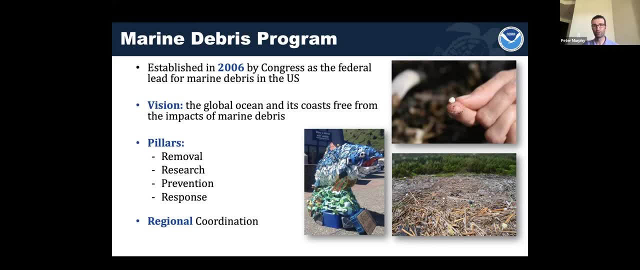 You know, unfortunately that's the reality, But you know it's an aspirational goal And I think that we drive towards in terms of how can we, how do we approach these things. Our key areas of effort are removal, So going out and actually cleaning up debris in the environment. Research, So better understanding the impacts, presence, pathways of debris. 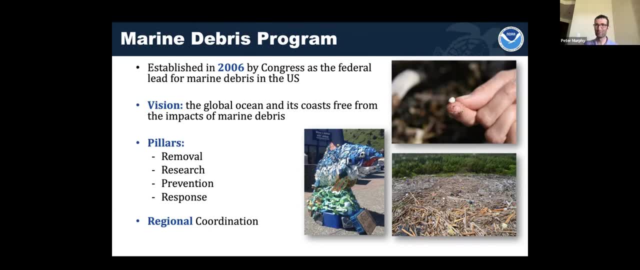 I'm sure you'll hear a lot more from Jennifer about those elements. Obviously she doesn't work for Marine Reprogram but you know an area of overlap obviously Prevention- actually changing behaviors to get to keep debris from getting into the ocean in the first place. You know that's a key area. And then response. 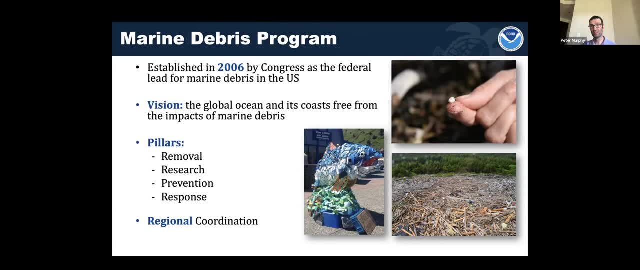 So while a lot of the majority of the debris that goes in the ocean is the result of chronic actions, everyday things that you know- leakage from waste management infrastructure, etc- There also is a significant amount of marine debris that can come into the ocean for individual acute events, And so responding to those is also part of what we work on. 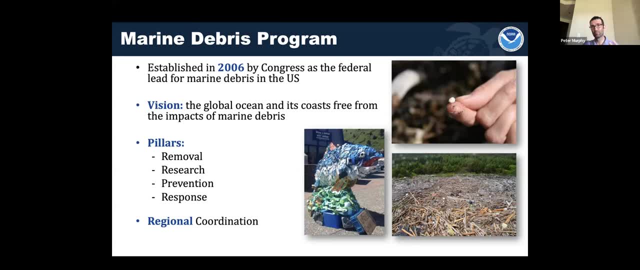 And we do that in a regional structure. So my region of focus is Alaska, which of course includes the Arctic, because you know that's the Alaska is what makes the US an Arctic country, So obviously there's an alignment there. 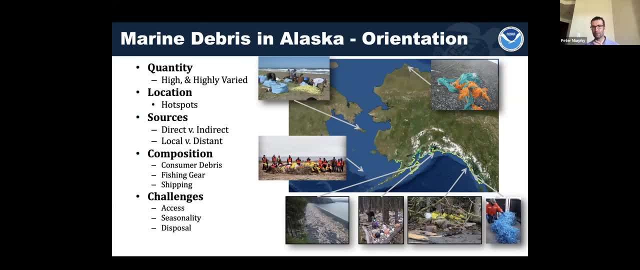 So a little bit of context to the marine debris issue in Alaska. And you know, when we say marine debris, just for context, we're talking about, you know, man-made, person-made objects that exist in the marine environment, whether they were intentionally or unintentionally disposed of. 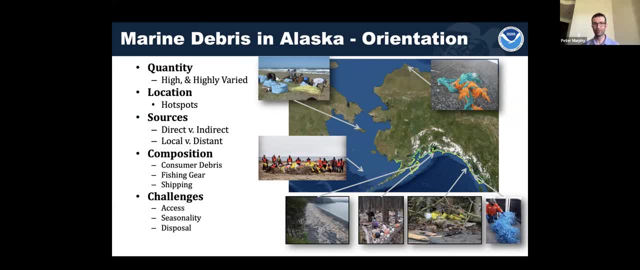 You know that's everything from microplastics to derelict fishing nets, all sorts of items You can see in these images here, examples of those So fishing nets. actually some images from the Pribble Office. I see Veronica online. 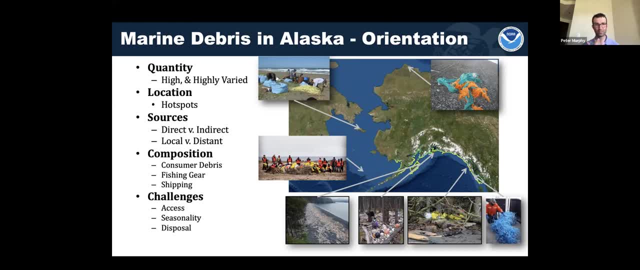 Also images from St Lawrence Island. I see Gay also online, who's done a lot of work out there, And so you can see the diversity of items that exist here. So you have, you know, everything from fishing nets to buoys. 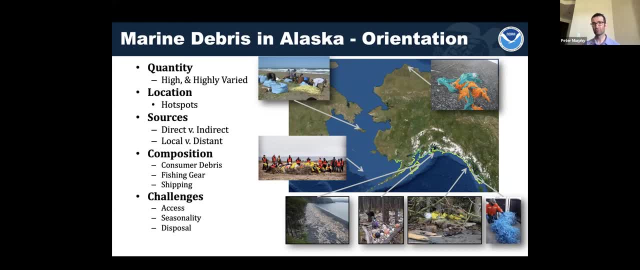 You know a lot of things are associated with the fishing industry and fishing effort. just given that that is such a huge part economic and commercial engine in the state of Alaska. These are very productive waters over the years. But also there's interesting commonalities. 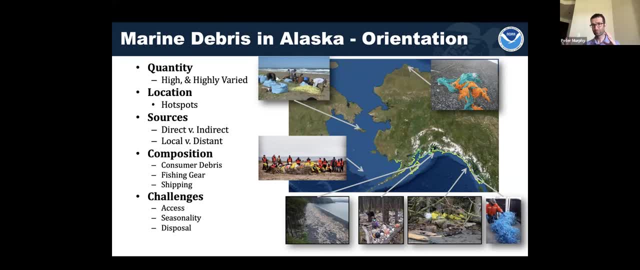 While there's differences across the state in terms of the distribution, there's also commonalities. You can see at the upper left of the images there an image of packing bands on St Lawrence Island, But then at bottom right there's an image of packing bands as well. 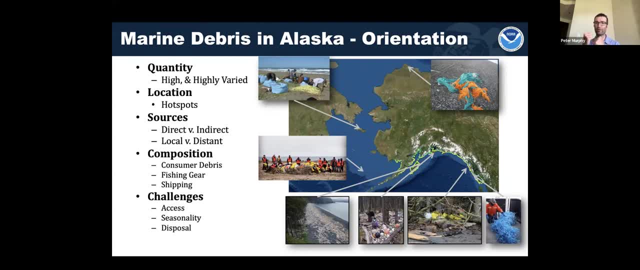 And you know, many of you may be aware of these. These are the heat-sealed bands that go around, often heavy items. You see them in, you know, big box stores like Costco or wherever it may be Best Buy, you know, for washing machines. 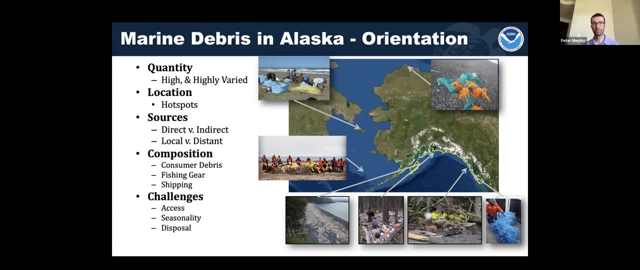 They're also used in the fishing industry, And we'll talk more about that a little bit later, But what the thing is, though, is that they're used in the fishing industry, And we'll talk more about that a little bit later. 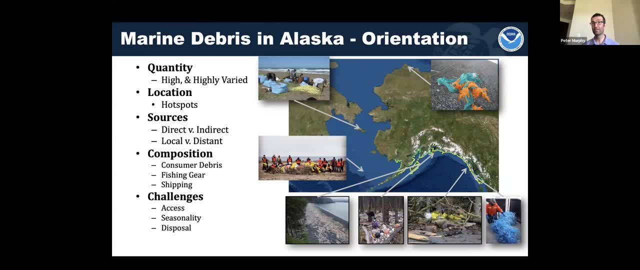 But what the thing is, though, is that they're used in the fishing industry, And what the same thing that makes them really great in their intended use makes them very challenging. They're very. they have high tensile strength. They don't break down easily. 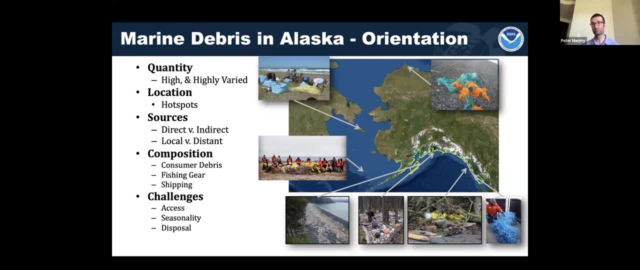 And just when there's an entanglement issue, when an animal gets caught in them, it can cause incredible damage to those animals. So, going back to kind of the content, you know the quantity Alaska has- not only you know- with more shoreline miles than the rest of the United States combined. 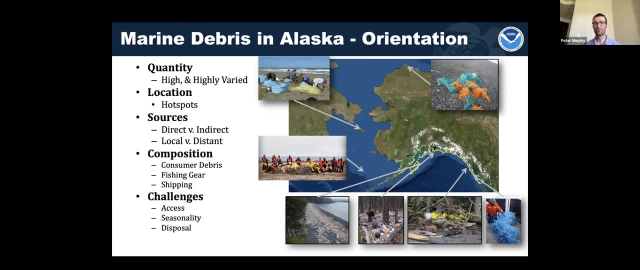 not only that, but also, on a mile-per-mile basis, some of the highest concentrations of marine water. not only that, but also, on a mile-per-mile basis, some of the highest concentrations of marine water And the most common sources of marine debris we see are in the state of Alaska. 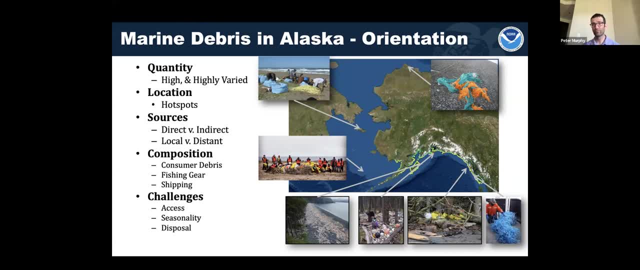 So when we add that up, it's a huge amount of marine debris, And a lot of that is driven by the fact of Alaska's location, as it relates to wind and current patterns, you know, in the North Pacific that bring not only locally derived debris, whether that's from, you know, near shore. 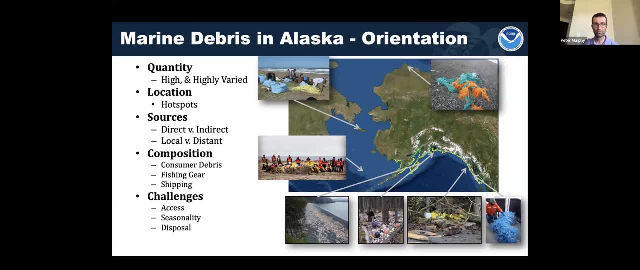 but also distant debris from the open North Pacific that comes to Alaskan shorelines. So that can really drive a lot of that. And that points to the sources, both direct meaning items that go into the ocean, you know immediately, are disposed of into the ocean or lost into the ocean. 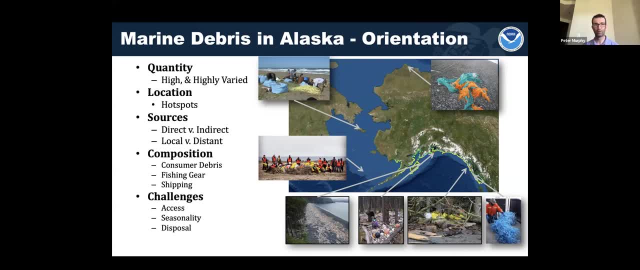 or items that flow from watersheds, which we'll talk about more later, But also local and distant sources. So certainly I think that's an area in which Alaska is different in that a lot other parts of the country or the world you know. 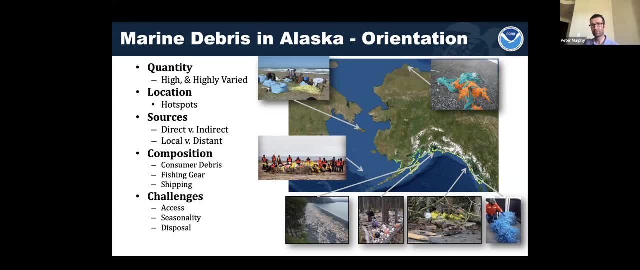 a decent amount of the input of debris is locally driven And certainly there's local introduction in the Alaska waters or near shore. but there's also a lot of distant sources as well And, as we've already talked about, the composition is varied from consumer debris. 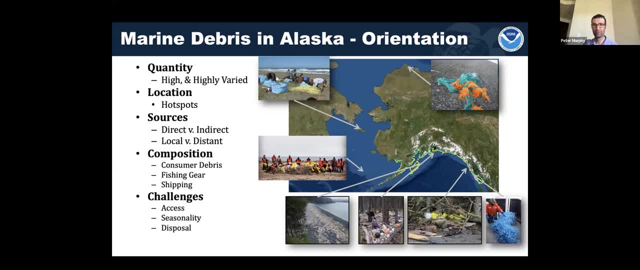 to fishing gear, shipping and many other sources. So challenges, obviously, access. you know many of these places where debris aggregates is far or far from population centers and requires significant logistics- Seasonality of course. anyone who's worked in Alaska knows you know. 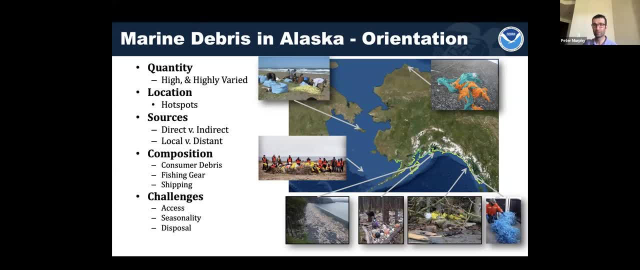 many of these locations are not accessible for significant parts of the year. And also that brings an element of equity, because when you're trying to plan a cleanup, you're competing with the field season for people from a professional standpoint as well as resource gathering standpoint, to the level where they may not be able to volunteer. 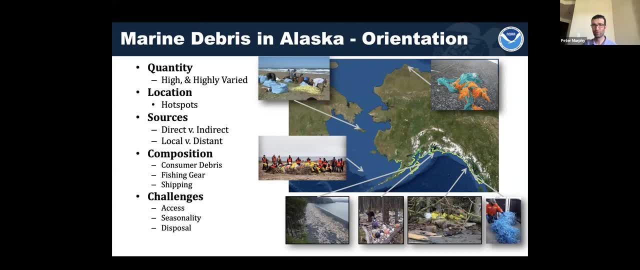 which might be an expectation for cleanups in other parts of the country or the world, And so there's an element of that that needs to be taken into account for equity and for planning. Disposal can also be challenging In Alaska, with many of the landfills or waste management infrastructure was planned. 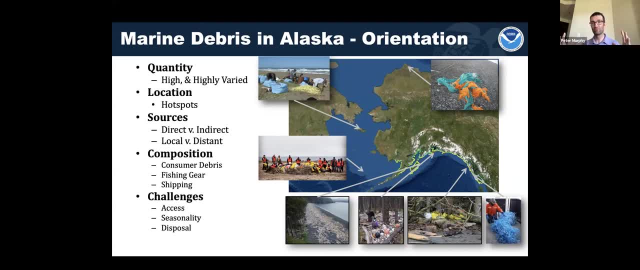 for the size of communities that exist, not for influxes of tons or tens of tons or hundreds of tons of debris from the open ocean. And so many landfills have closed themselves to marine debris. They don't accept it because they don't have the local revenue to accept it. 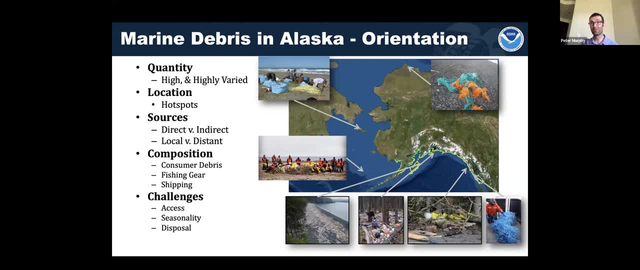 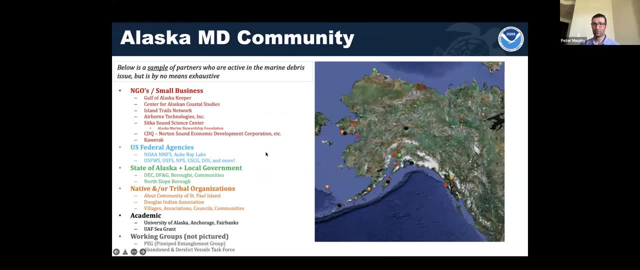 And so that means that you have to find more complicated ways to get rid of the debris. So another note is just as I mentioned earlier that marine debris program, we see ourselves as part of a community. This is a slide that just is a general, it's a sampling. 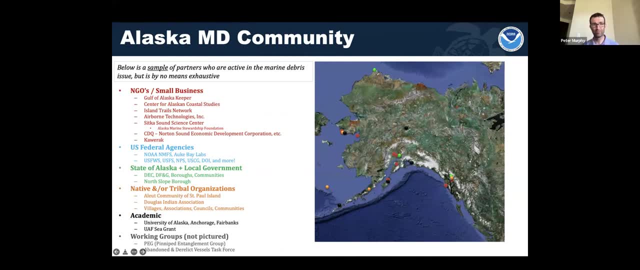 I try to emphasize that At the top it's a sample of partners who are active in the marine debris issue, but it's by no means exhaustive, So I'm not planning on reading this. But the key thing I want to point out is just there's a broad range of innovative, active and dedicated groups who are working on the issue. 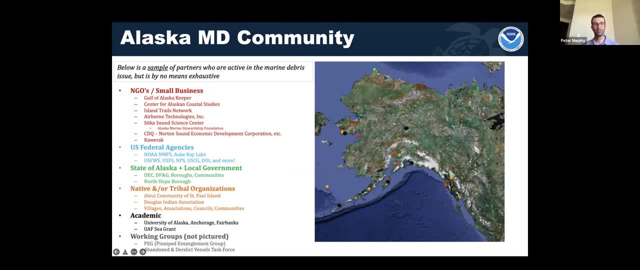 Includes NGOs, federal agencies, state of Alaska, native and tribal organizations, academic groups, working groups, as well as other categories that cross those lines. But I just want to point out- I think that's an important element- is that there's a broad and growing group. 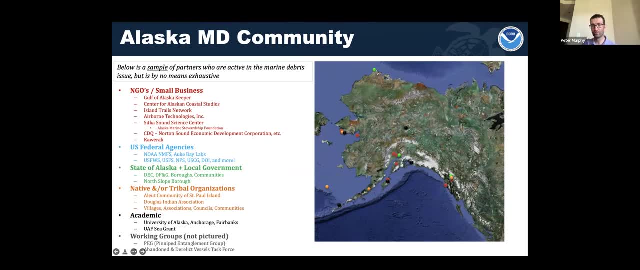 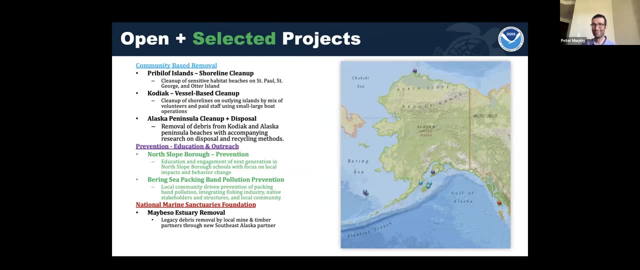 and very interesting list of groups that are very active in the overall issue of marine debris within the state of Alaska. So I want to briefly just highlight a few projects. Actually, for part of this I should have had Veronica should give the talk on the varying sea packing ban pollution prevention project. 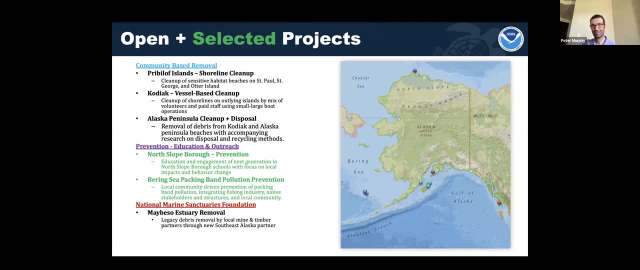 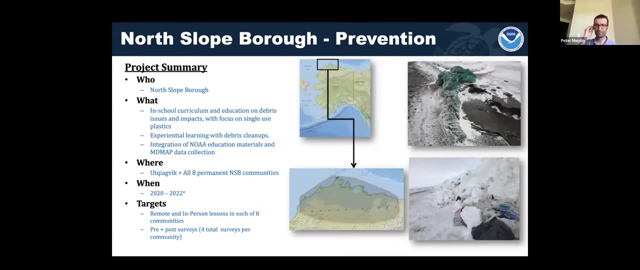 But just highlight. these are active or recent projects in the state of Alaska that I want to highlight or talk through. I'm really focused a little bit on prevention because, realistically, one of the things we've talked about is that you know, can't you're trying to just remove, you can't clean your way out of the marine debris problem. it's like 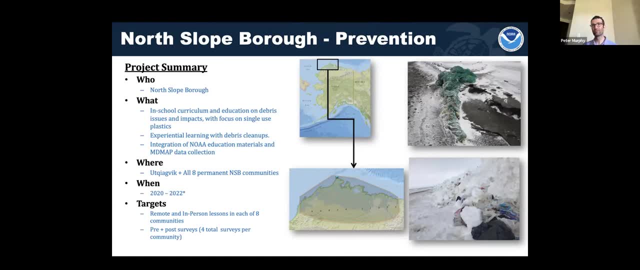 trying to empty a bathtub with a faucet on. so we need to be preventing and changing behaviors, and i think that alaska has a unique power in that, in that, um, while people are accustomed to beach combing and to the concept of things washing up, often that can be more in a friendly or appealing 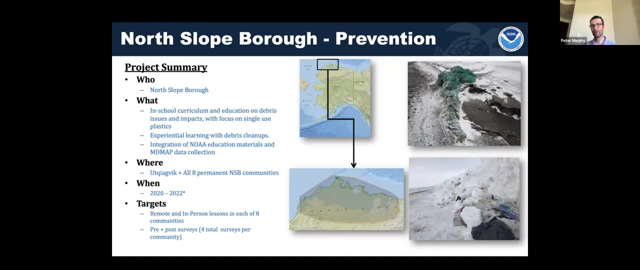 way, whereas the reality can be that you have beaches that are so far away, as we mentioned earlier, from any population center that just have a huge amount of debris. i think that can resonate with people because they think of, you know, pristine wilderness. um, you know why is it there's? 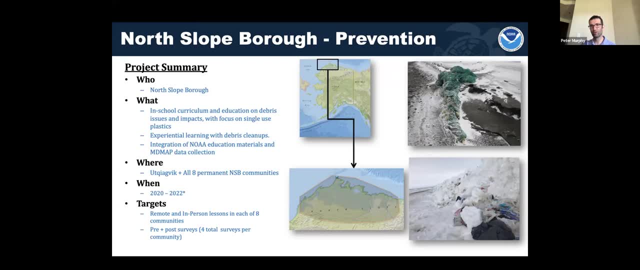 garbage on these beaches, hundreds of miles from um, from the large, large population centers. i think that can really be powerful. anyway, on the specific project, so two that are active right now. um is a north slope borough project, so that's working with the north slope borough government itself. 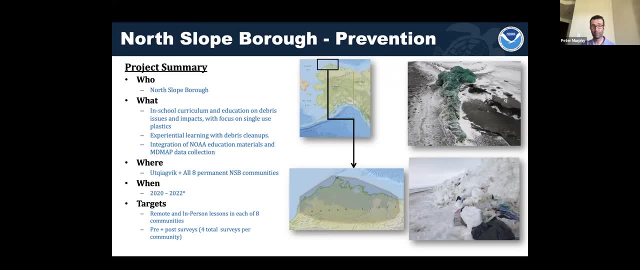 um to conduct in-school curriculum education on debris issues and impacts, with a focus on single-use plastics, so actually choices that can be made locally to drive change um. so that includes ukiyavik and all eight permanent northslope borough communities. there have been some challenges with this, of course, with pandemic requirements and 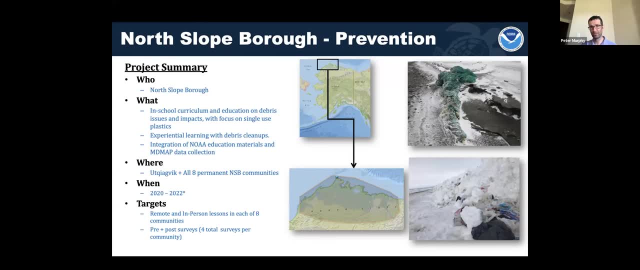 and safety. you know rules as far as how schooling has been done, so this project has been delayed and adapted a bit, but it's one we're really excited about for the opportunities to both engage and also learn that the northslope borough is going to have also the bering sea packing. 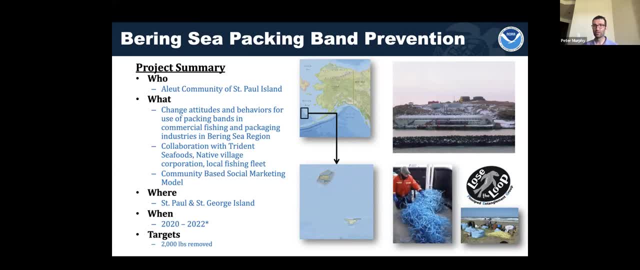 ban prevention project, as we mentioned earlier. you know these are issues. these are unique to different types of debris. that's very important and also potentially damaging, and so there's been a lot of focus in alaska, actually, there's a group called peg pin and pen entanglement group that 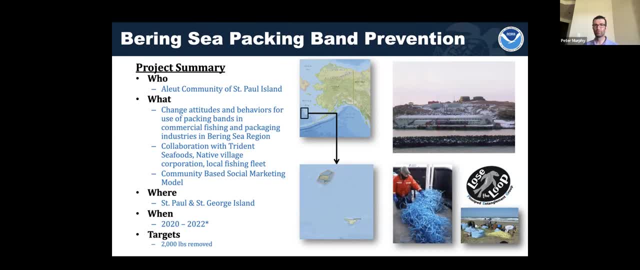 has discussed the issue of packing bans for quite some time, as well as even looking at biodegradable alternatives, but one of the things that we look at this project was through the allied community of saint paul island. what they're doing is they're working on trying to change attitudes and 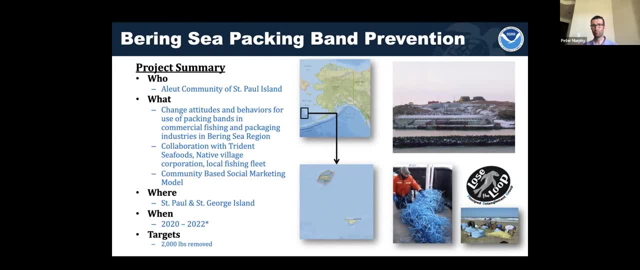 behaviors for packing, bans, use and how they're managed and where they are used, and whether or not in collaboration with Trident Seafoods, a very major seafood company, fishing company, as well as the local community and the local fishing fleet. And so, as I mentioned, I'm giving a very brief summary. 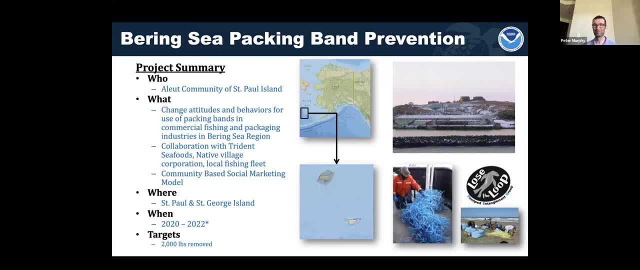 Veronica's online, as I saw, could give a much better one, and I've seen her give very good ones, But I think the credit to this is that I think there's really strong elements of community engagement and also really trying to have a targeted debris type, because the issue can be quite overwhelming. 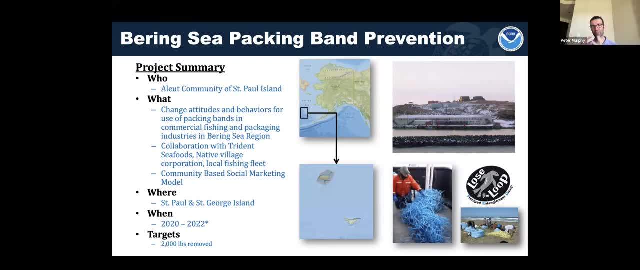 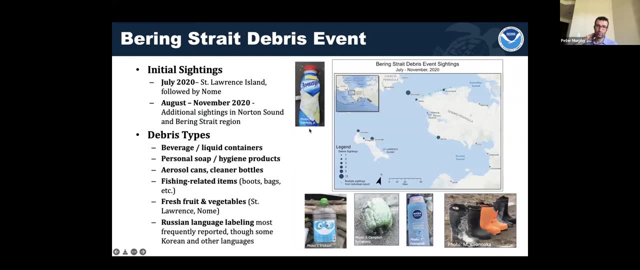 There's so many different types of debris, How do you break it down? So having this intentional model is, I think, a good one for looking forward. I also want to mention a relatively recent- last few years- example of more of a response element. 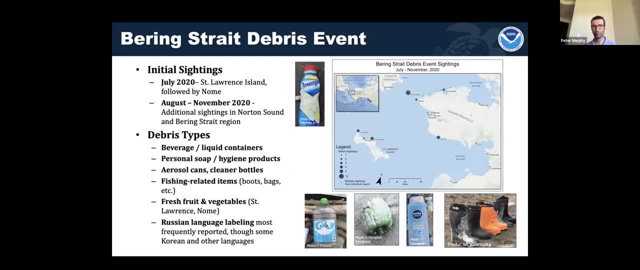 or of an element of acute debris, so debris entering the ocean at a specific point in time. So this is an event that occurred starting in July of 2020 and into the fall of 2020, where there was a significant amount of marine debris. 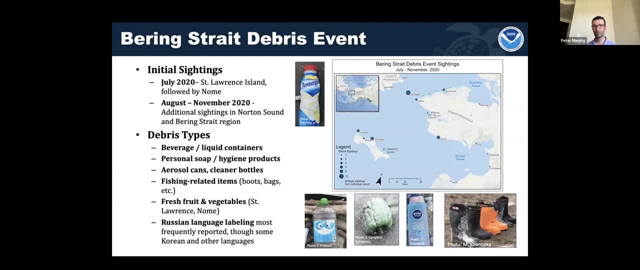 that was unusual, both by quantity and by type, that began arriving on the shorelines. You can see images at right that you know these were all sightings that were reported to Alaska Sea Grant or Coeric out of Nome, And so you can see these images are of debris types that are, you can see these items are relatively fresh. 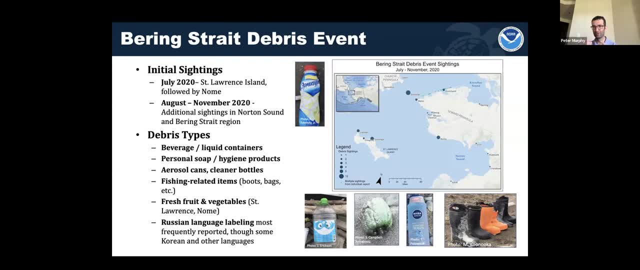 They're new. Oftentimes we've all been on beaches. You see those items that are brittle, They're aged, They look different, They look, you can see, they've been out in the weather, in the ocean for quite some time. 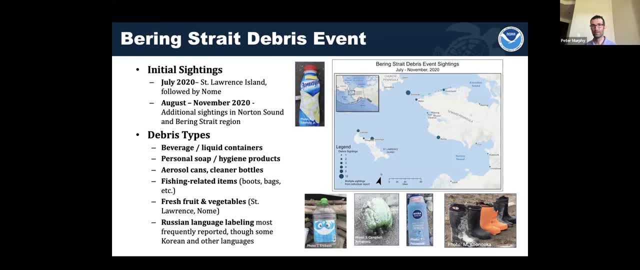 Obviously, these items, some of them look like they could have come off a shelf. you know right then, So it really pointed to. you know a recent introduction of a lot of debris items And so you know you saw beverage and liquid containers, personal soap and hygiene. 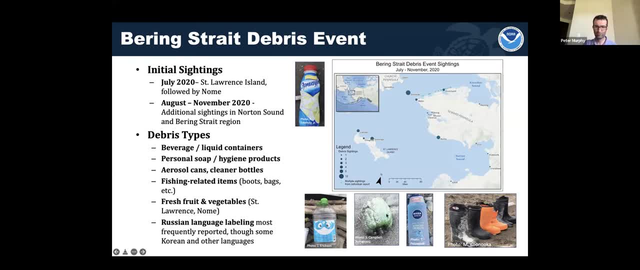 but also fresh fruit and vegetables. You see that image at lower, the lower kind of part here of that. you know what looks like a green bell pepper. Obviously that points to both that not being in the ocean for very long, and you know. 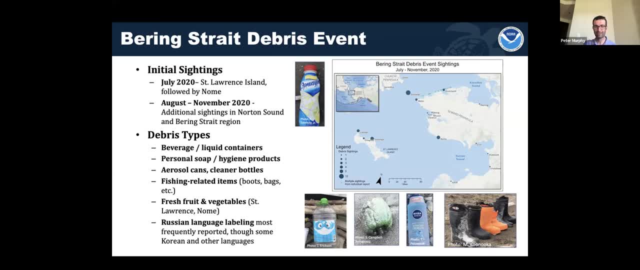 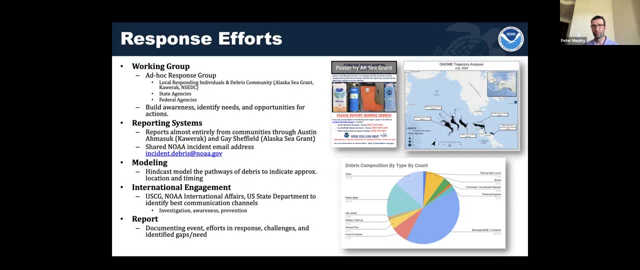 and also an unusual debris type. You really see things like that So working. you know, the alarm was raised by the local groups as I mentioned, Coeric and Alaska Sea Grant, who really, as you know, I think Kay Sheffield's on this call. 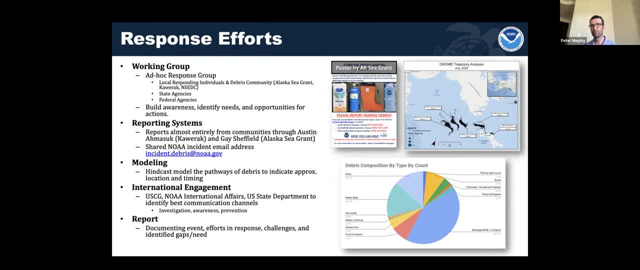 was really instrumental in this project and this effort. But there was a, you know, an awareness of: hey, this is unusual, We need to, an effort needs to be undertaken on this. And so a group was put together, kind of an ad hoc group, of individuals who had connection to 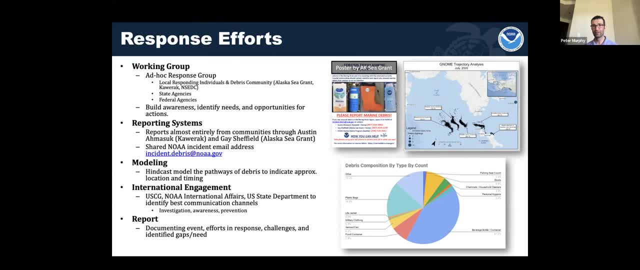 or concern about the issue, to try to build awareness, Identify needs and look for what opportunities for actions and in terms of investigation, communication could be taken. So reporting systems. So, as the slide indicates, you know you saw that graphic in the last one- 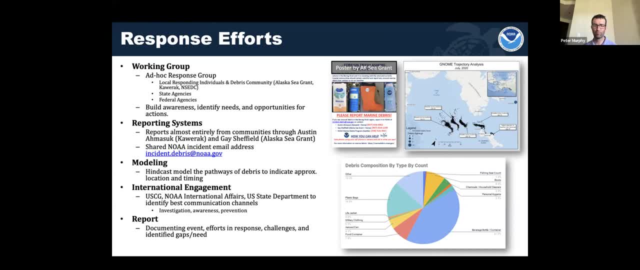 which showed where the debris locations were reported from. The reports came through from the local community members who took time out of their very busy lives to, you know, catalog and raise the alarm of hey, we're seeing these items, and then document those. 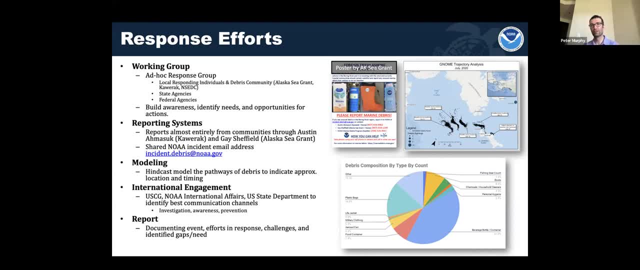 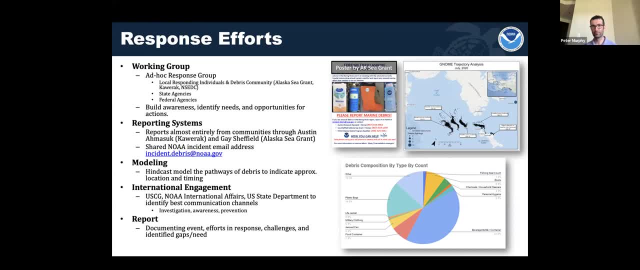 We also set up an email address in case. that was helpful for people. Although the vast majority- almost entirely the items came, the reports came through Austin and Gay, But we were able to use those to try to understand where the debris was and what the timeline was. 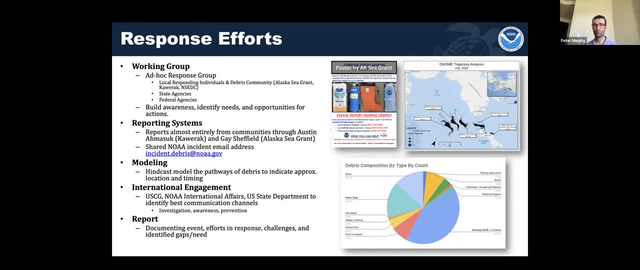 And then using those we were able to conduct some hindcast modeling to look at where the debris may have come from. So using the NOAA Nome model I know this is kind of an oceanography group at Root, So the NOAA Nome model is typically used for oil spill response. 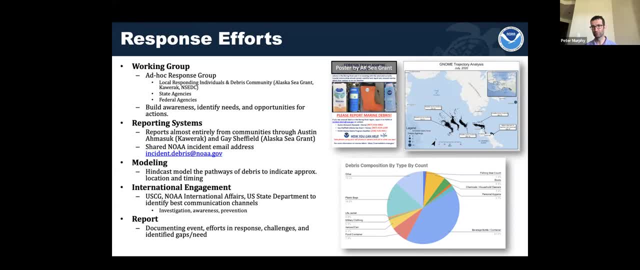 So looking at where debris or where oil may go in the future, pollutants may go in the future, to inform and improve, hopefully, response operational actions. But in this case we were able to use it to look backwards to see where the debris most likely may have come from. 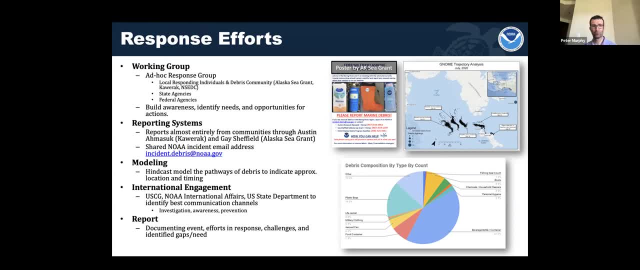 which pointed towards the Gulf of Vanadir, And so we also worked on international engagement, working with Coast Guard international officials. We worked with the National Affairs and State Department to identify communication channels and try to make contact with the Russian Federation government. That was really challenging. identifying who the best point of contact was and remains an area of challenge. 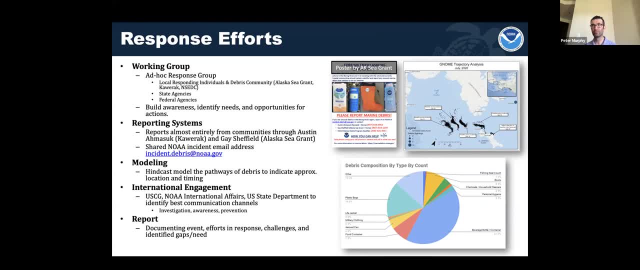 Obviously in the geopolitical climate. now, while that's still, it's been on agendas and meetings. obviously those meetings are not going forward at present And even as points to that was July to November of 2020 was the event. 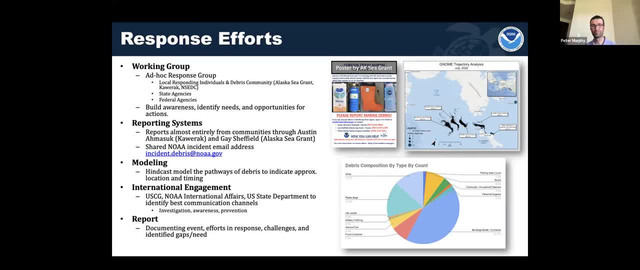 And the fact that it's still an area of contact and the fact that it's still an area of effort points to the challenge of that. And those efforts and challenges were documented in a report that was put together to kind of document. you know, here's what happened, here's what was. you know what was attempted, what was intended. 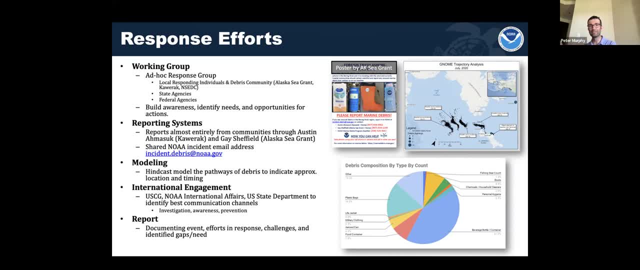 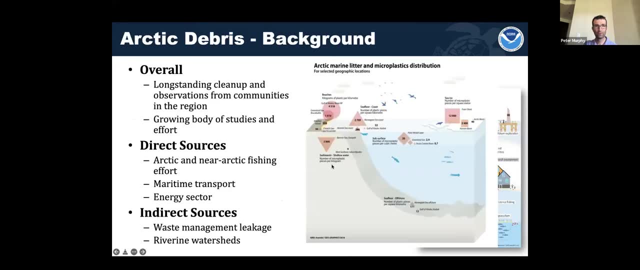 what response actions were taken, but also what the challenges and needs are, so that hopefully, if there's another event, what could be improved. So with that transitioning kind of you know what will we address in the next two or three years. 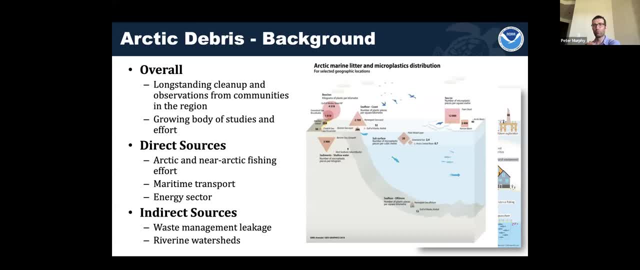 I'll stop with that, but I'll just try to put you guys back, because I think this is a really exciting moment that people have been, sort of you know, taking out organizations that are really working on soft northbound sandstone dioxins going. 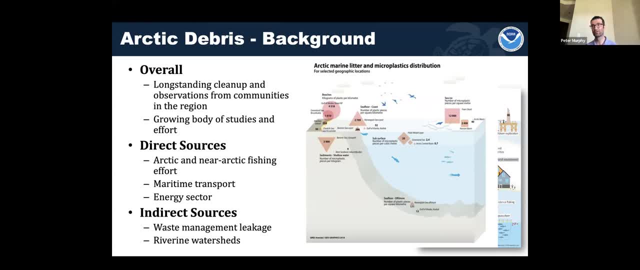 particularly towards global South Podcasts, turning local South Podcasts beyond. over the years- including嗯 For it to have such an impact- evolved within Alaska for over a million pounds of debris they've removed, and so there's been a lot of effort. 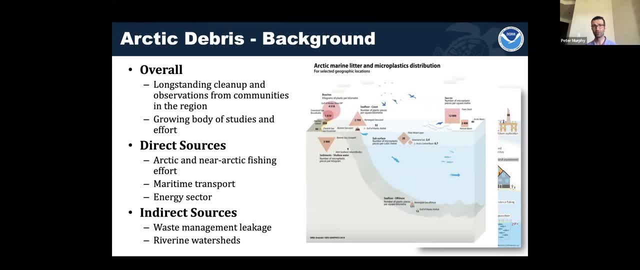 and there's also a growing body of studies and academic and research effort within the region to better understand both the presence and distribution of debris and the potential impacts. I'm sure Jennifer will cover or touch on a lot of those as well, but again pointing to the nature of, 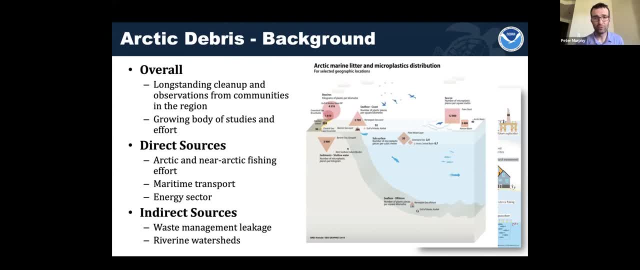 direct and indirect sources that occur. so you have also the arctic and new arctic fishing effort, which can directly introduce marine debris or marine litter into the ocean as or indirectly. so it's kind of belongs in both, but you also have directly into the marine environment, that is to 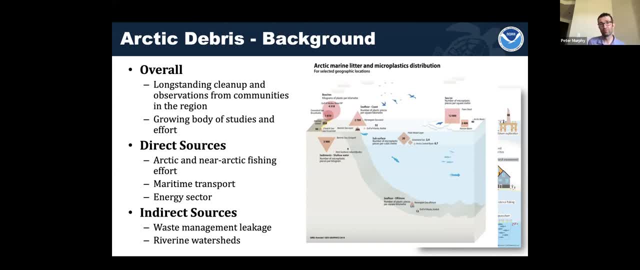 say, but that can also be a distant source. but then you also have the maritime sector with transport, that where you have loss of items or items going overboard, that can certainly introduce debris as well as energy. so oil and gas, that sort of thing, that certainly can. 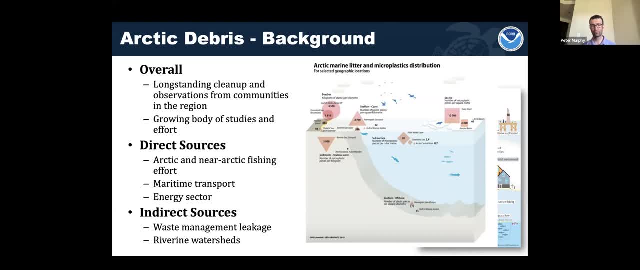 introduce debris as well. the graphic at right is from grid arendal, which, of course, is a primary partner that does a lot of work with the arctic council. that points to just the data of where debris has been found in in different locations within the arctic. so as far as sources go, that 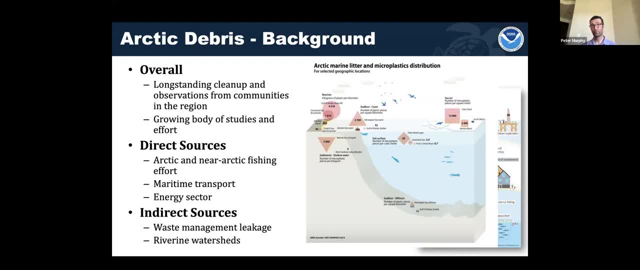 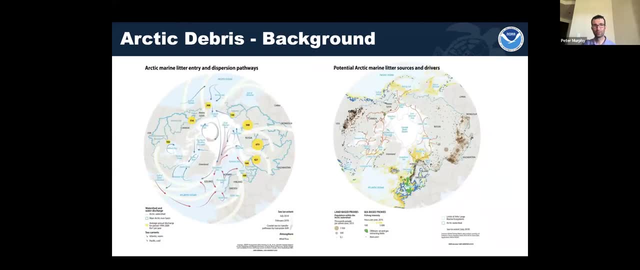 also points to the waste management leakage from within both direct areas within the arctic, but also riverine watersheds that can wash debris out into the arctic, and this graphic is one that i found helpful: um, from the arctic council structure, um, but really points to just the you. 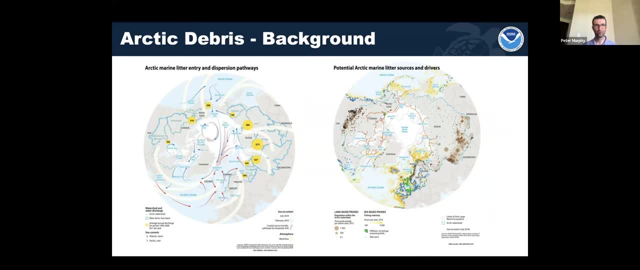 know there's a lot going on, but really i think some of the key things i would draw um, draw attention to is that you know these pathways of debris that can come into the arctic um potentially from um, from the open ocean, from north pacific, north atlantic, um, but also from riverine watersheds. 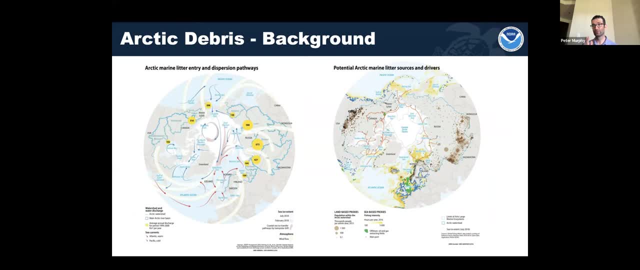 um. so you know, there's a massive river discharges that make terrestrial influences particularly strong and important in the arctic ocean um which, while it holds a lot of weight in the arctic ocean, it holds less than one percent of the global ocean volume. um. the arctic ocean receives more than 10 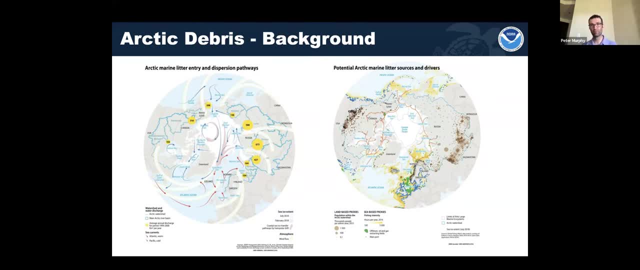 of the global river discharge, which was something i found really interesting when i was starting to dig more into the arctic, and so you also have huge population centers very far upstream within these watersheds, which can point to introduction over time and into the arctic. 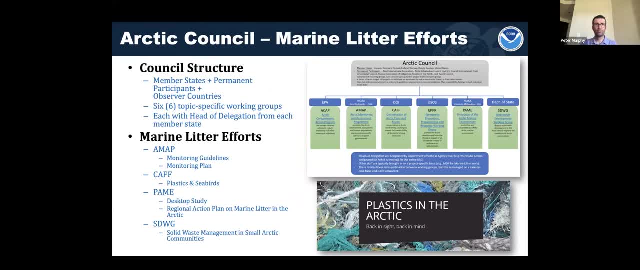 so briefly just to mention that within the arctic council structure growing and increased work on marine litter as a as a focus topic. as icelandic leadership of the arctic council, which just had their two-year term expire, they have made marine litter or plastics in the arctic a focus area. you can see at the bottom right and i'm sure for those 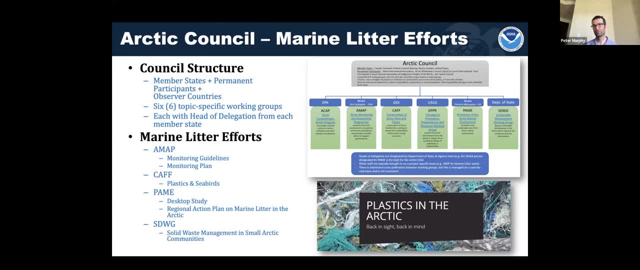 of you all familiar that you know the arctic council has those six persistent long-term working groups and, fully at point at this point, four of those have specific efforts on related to marine litter. so i think it points to the effort that is ongoing um and the and the focus and interest on the issue. 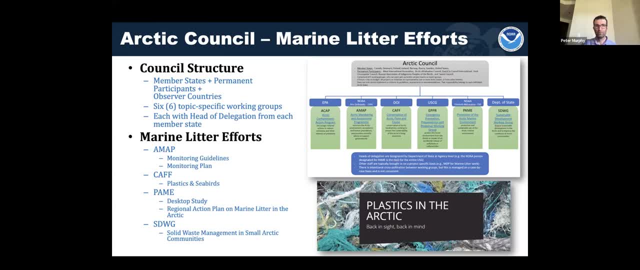 of marine litter within the arctic council, and so two of the ones, i'm sure, um, as i keep on saying that jennifer is really one of the leads on the monitoring guidelines, monitoring plan within the amap structure, um, but, and i'll just briefly touch on it, um, but then there's others that 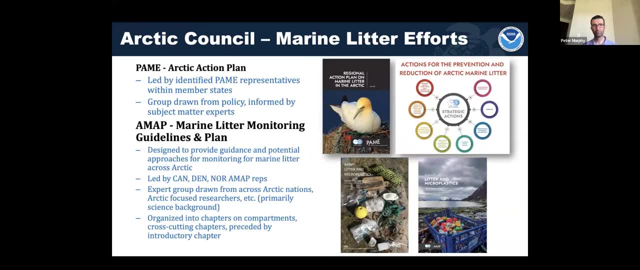 are also ongoing, including um within the protection of the arctic marine environment, um, the or pain um, which is also an important part of the project, and so the the arctic action plan approach that's been put together and includes efforts to kind of catalog and focus on what work can. 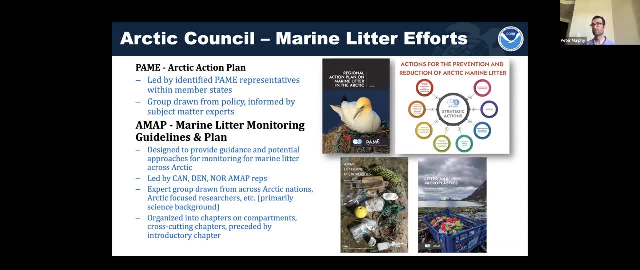 be done and should be done ideally in the arctic to prevent research and, under research, to understand and prevent and also remove, hopefully, marine litter in the arctic as well as, as i mentioned, the amap marine litter monitoring guidelines and plan, which focus more on understanding, which, again, I'll defer more to Jennifer on that. 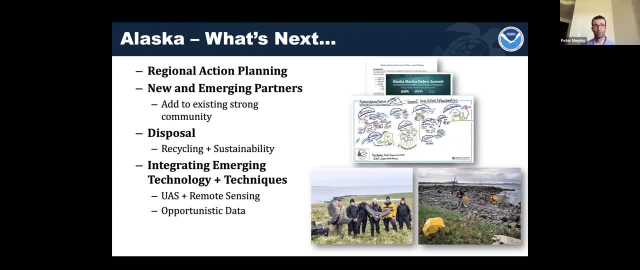 So what's next in Alaska and the Arctic? So regional action planning- that's something that we are focused on in the near term- is actually better putting together documents and efforts to better understand and codify what those efforts that are already happening, what the priorities. 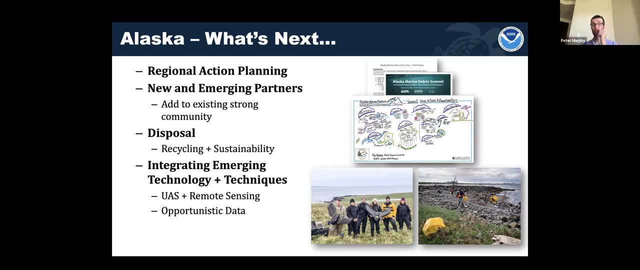 are and also what the gaps, needs and opportunities are in the future in Alaska. That's something that's been done in many other parts of the country and the world as well, but hasn't up until recently, hasn't been a focus area in Alaska. You know the community. 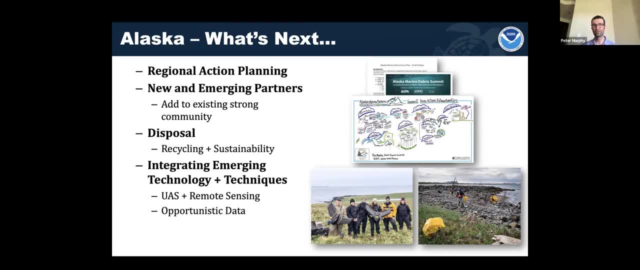 itself didn't necessarily see the value at that point in time, but that started to change and there's groups that are interested And so now, at the time, we're excited to get to launch on that And I think part of that comes from there's new and emerging partners, So there's groups in Alaska. 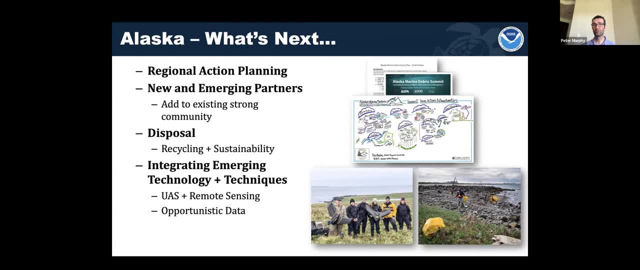 that are, that have historically maybe were more. you know they weren't active in the past, but now they're active in the future, And so I think that's something that has focused on marine debris, but are making it more of a focus of their efforts as well as a long 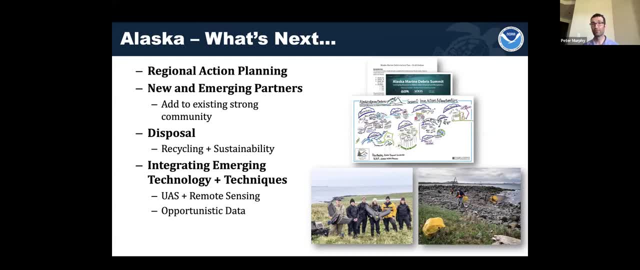 list of groups for whom they have such hard-earned experience and knowledge on the issue And so putting that together, the experience and knowledge of these groups that have been working for a long time with the energy and ideas of the new community, new members of the community, I think. 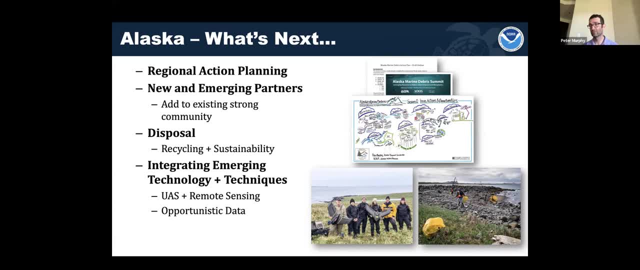 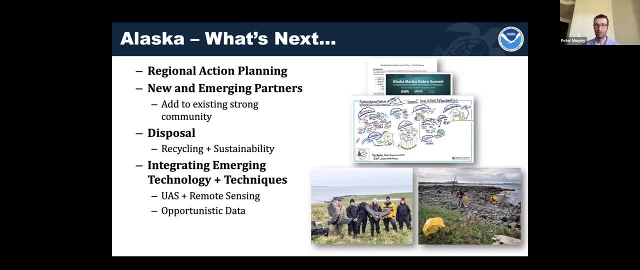 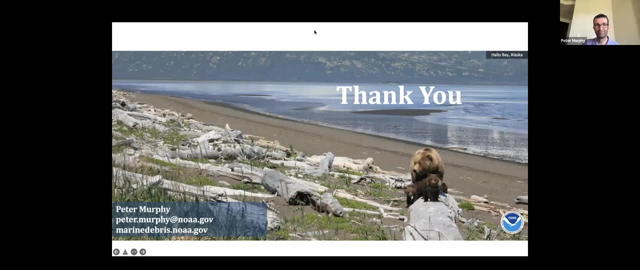 for sustainability and recycling, And then also looking for opportunities to integrate emerging technologies and techniques. So with that, I want to say thank you very much, appreciate your time and look forward to talking further. Awesome Thanks, Murphy, Thanks Peter. This is awesome. It was a really great overview of the. 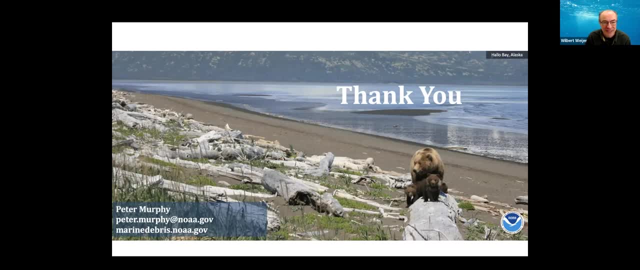 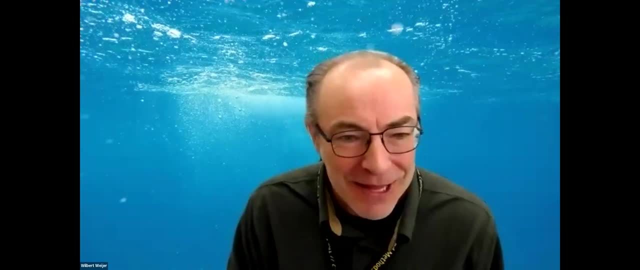 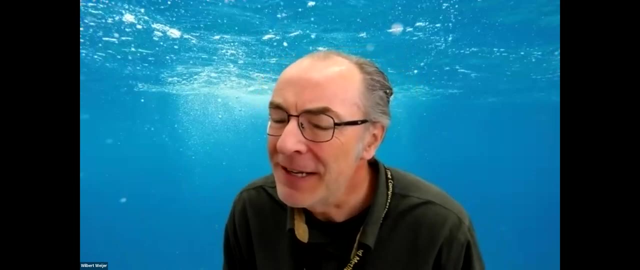 activities that you're involved in and that you're leading, obviously from your position as a NOAA lead on marine debris. Thank you very much. Thank you, I'm sorry. I definitely want to give some time to Veronica to share some of her results. 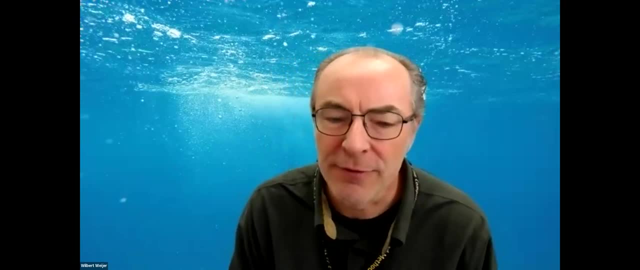 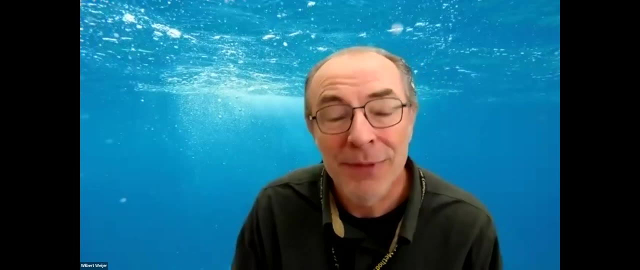 Maybe. why don't we hand it over to Jennifer first, then to make sure we are a little bit behind schedule, to make sure that she has enough time, And hopefully we'll have some time for Veronica to to show a few slides, And then hopefully we'll have some time for discussion And, if you have, 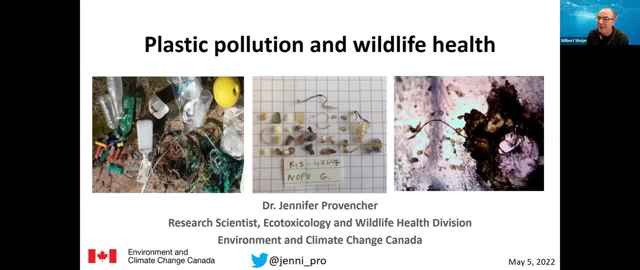 questions for Peter. please put it in the chat and I'm pretty sure he will be happy to answer them. Thank you very much. I'm happy with that. Thank you very much. Thank you very much. Thank you, Thank you very much. 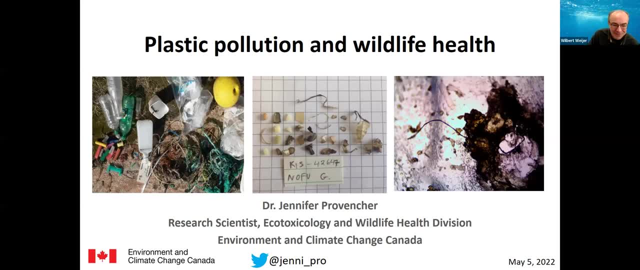 to enter it in there, Jennifer. Awesome, And thanks, Peter, It's always great to talk with you, And so we haven't seen each other in a while. so nice to see you online. So yeah, hi everyone, I'm gonna shift us a little bit. 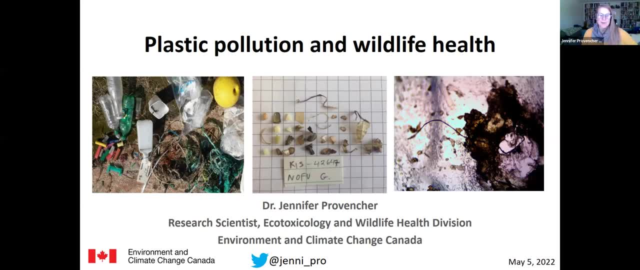 I'm an ecotoxicologist And so I'm gonna kind of shift us from. I always think, you know, Peter talks big scale and then I get really, really tiny, And so my first slide is actually just kind of taking us down there. 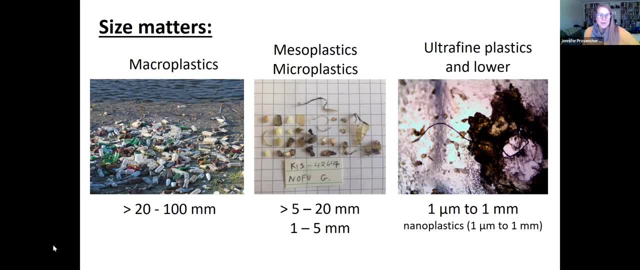 So in the plastics world, size matters And so while you know we just talked a lot about macro plastics, I'm gonna kind of move us down the scale a little bit. And primarily in my work we work on mostly mesoplastics and microplastics. 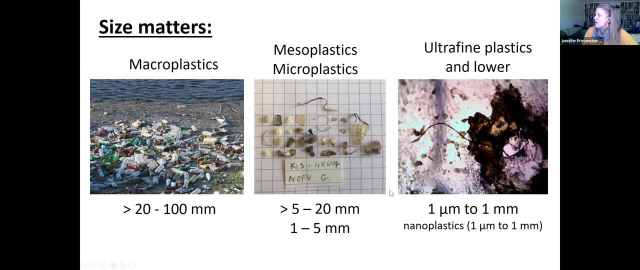 And in some of the work a little bit moving into the ultrafine plastics and lower, And you'll notice that the scales here are kind of messy and that reflects where we are at in kind of defining what some of those sides of plastic sizes are. 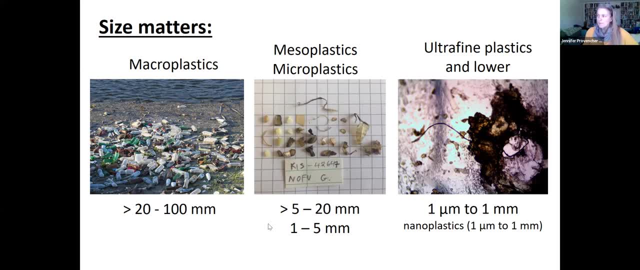 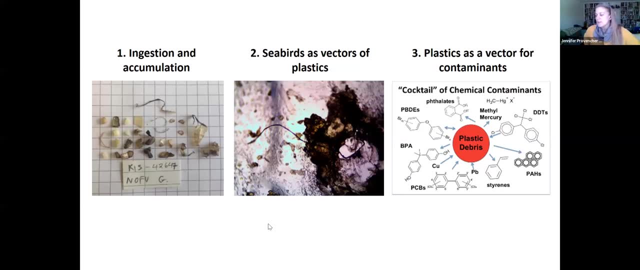 So in my lab- so I worked before Environment and Climate Change Canada And in my lab in particular- we focus on three plastic pollution kind of main questions. We do quite a bit of work on ingestion and accumulation, So this is really about documenting species. 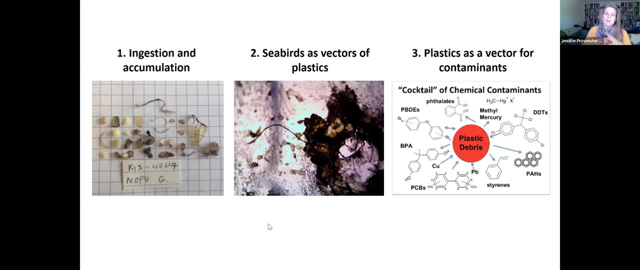 what species are exposed to microplastics, you know, do they actually accumulate them? and then you know potentially have those effects. And in part a part of that is: you know, you know, you know potentially have those effects. 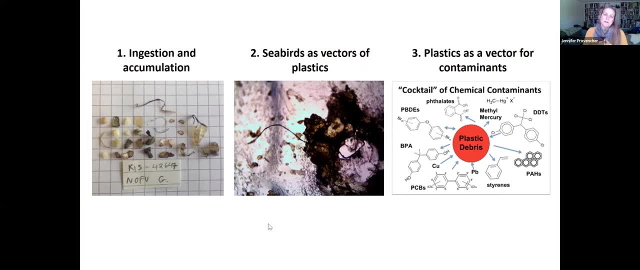 And in part a part of that is, you know, my work here is on the Northern fulmar, which is a species that is listed in the North Sea as an indicator for plastic pollution And as well in Canada we've listed it as one of our 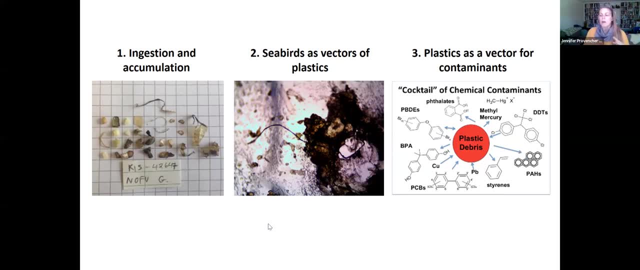 environmental sustainability indicators. And so we kind of have this program where we look at the ingestion of plastics by fulmars over time and space to try to get a signal on what plastic pollution is doing in the environment. Additionally, we do quite a bit of work on seabirds. or actually I should update this more animals. So we do quite a bit of work on seabirds, or actually I should update this- more animals. So we do quite a bit of work on seabirds, or actually I should update this more animals. 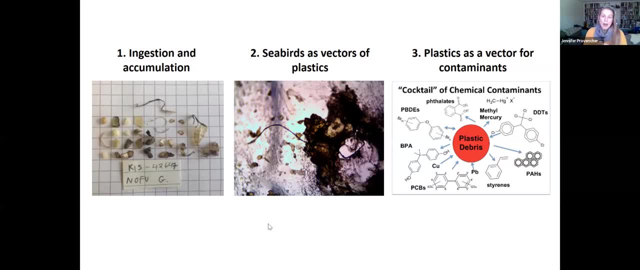 So we do quite a bit of work on seabirds- or actually I should update this more- animals as vectors of plastic. So we know, specifically migratory birds actually move plastics into the Arctic, And so this is comes a little bit later. 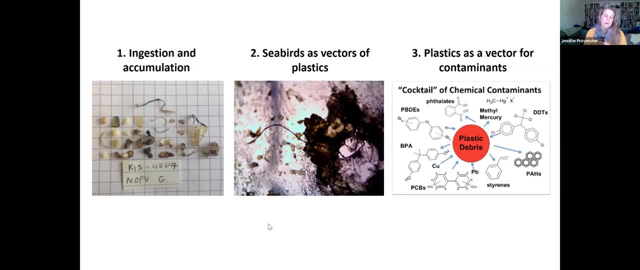 when we start talking about some of the contaminants. but this is an important part of the work that we've been doing And also moving plastics from the marine environment back into the terrestrial environment. So this is something that we're kind of thinking about, from our protected areas and whether birds 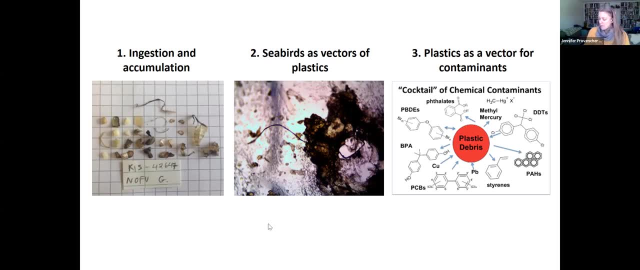 are kind of concentrating plastics around these protected areas, And then the one I'm gonna talk about today and focus on is really this: plastics as a vector for contaminants. And again, Veronica is gonna get some kudos here. This is something that Veronica has worked on as well. 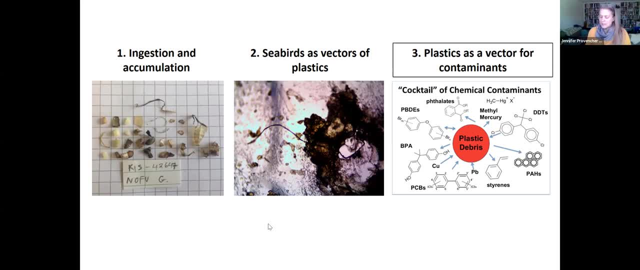 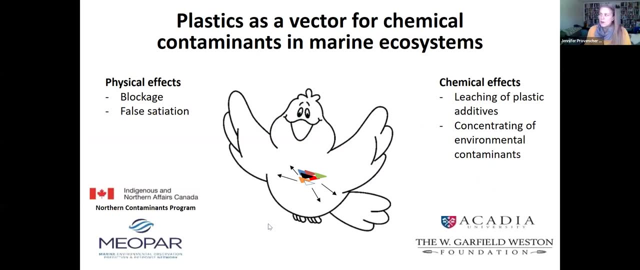 And I'm gonna kind of just run through some of the most recent work that we've done in the Canadian Arctic to kind of think about this idea of plastics as a vector for contaminants. So first of all there's the physical plastic that can sit in the stomach. 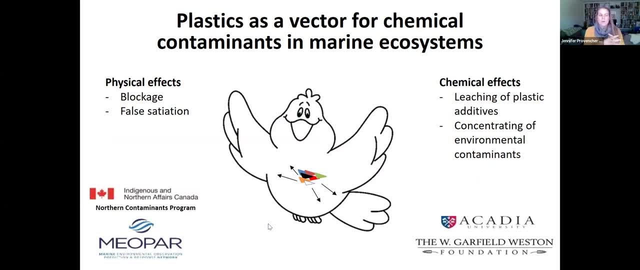 and this can have effects on wildlife, such as blockage. We've seen, you know, kind of ulcers around plastics. We've also seen some plastics actually like perforating the stomach, not so much in the Arctic but certainly in our more Southern sites. 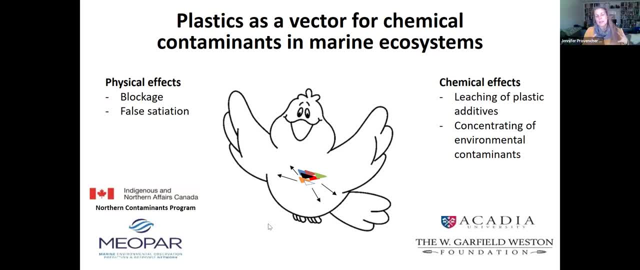 You can have kind of physical effects of plastic pollution in an animal. But what I'm gonna talk about a little bit more is some of these chemical effects, So we the leaching of contaminants into the animals and, of course, the concentrating of environmental contaminants. 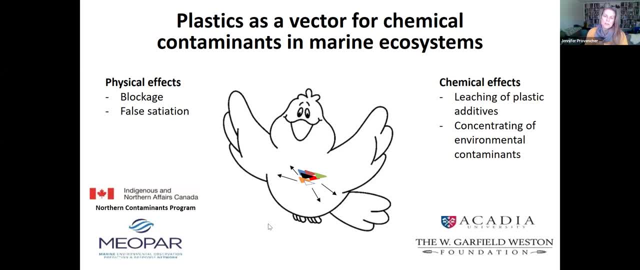 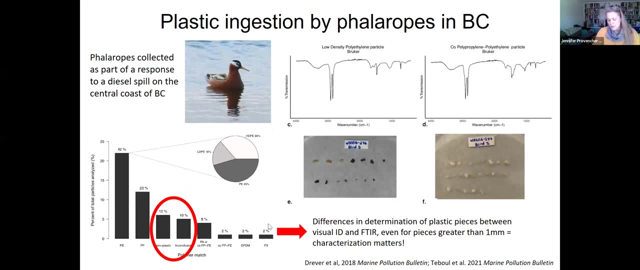 And a lot of this work is supported in our in Canada under the Northern contaminants program, And so this is a kind of a Northern Canada wide program that focuses specifically on contaminants and most often in country foods across the North. So first of all I'm gonna show you this data from: 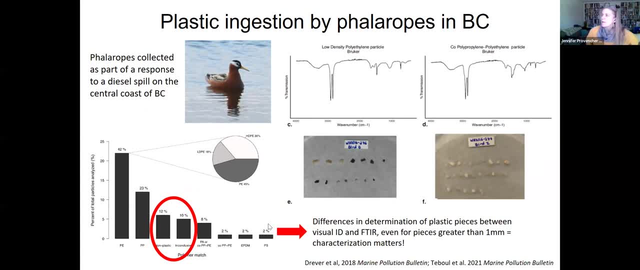 it's not in the Arctic, it's from BC, but some of the plastic ingestion, some of the really good kind of plastic ingestion data we have from phalaropes in BC And this just gives you an idea. So you know these are phalaropes that were collected. 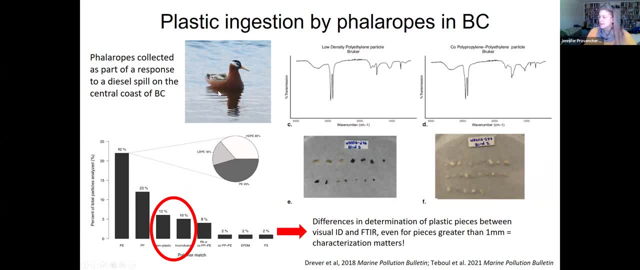 actually after a diesel spill and they weren't oiled or anything, but we found lots of plastics in them And we do plastic identification, primarily in birds, through a visual identification, And so you have these pieces that we can count and look at color and we look at their physical attributes. 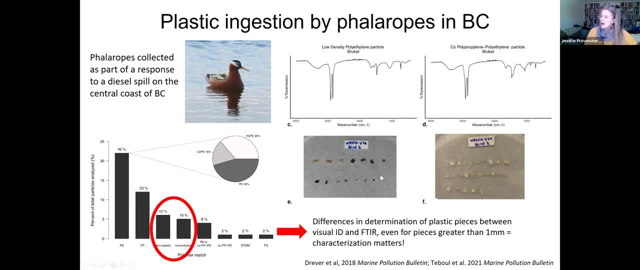 to define their morphology, but we were then able to also take them to polymer identification, And this is something that we're doing more and more And our regulatory partners are really keen as they start to kind of reduce types of plastic in the kind of in the system or on the market. 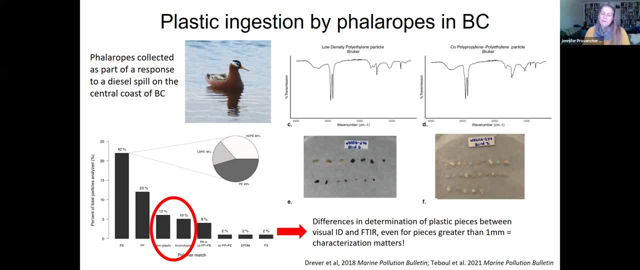 what they're really interested in understanding and how that those levels are reduced in the environment. And so we do FTIR on these particular samples and we get these polymer matches, And so polyethylene is a really big one, polypropylene We get a few other kind of more specific ones. 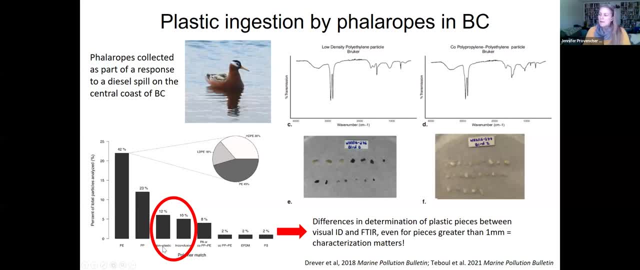 but one of the things that is really interesting from this study is that we also get these non-plastic or inconclusive results, And so for us this is really important, because we can physically see that it's plastic, but it doesn't necessarily come back as a polymer ID. 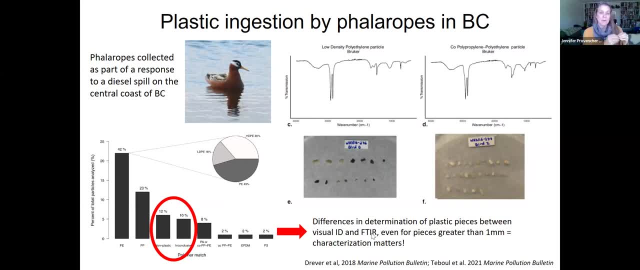 And when you have smaller plastics, that often tells you that it's not plastic. but when you have these bigger plastics, that you know we can see much more detail. it also tells us that you know some of the weathered plastics are not really being done. 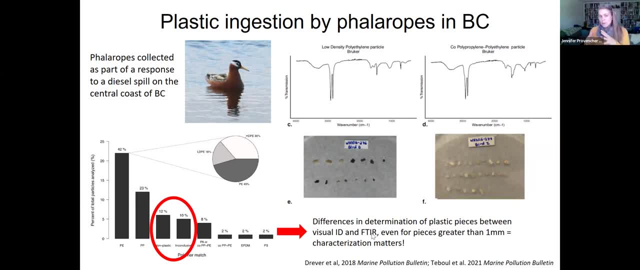 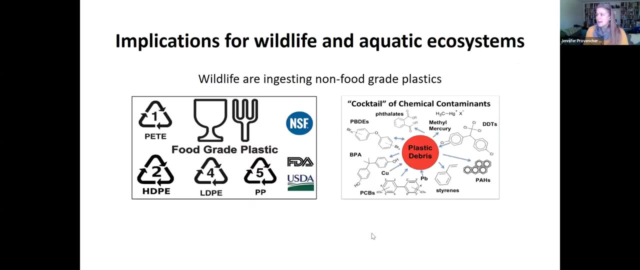 as well by some of the libraries in our spectroscopy work. And so all this is is that the polymer ID of the plastics. it can be really complicated, Okay, But that has implications for the contaminants and for the effects, And so at the end of the day, you know, 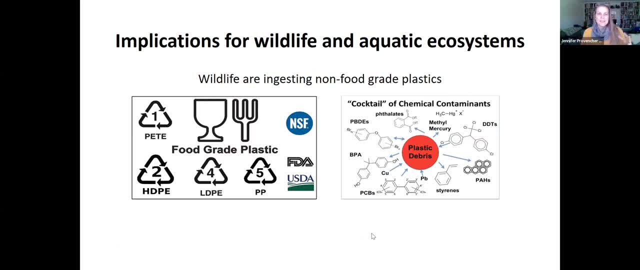 we have probably all eaten- you know things off plastic. today, Much of our food is stored in plastics- certainly at the stores And, but for the most part those are food grade plastics. And what we're seeing from our contaminants data. 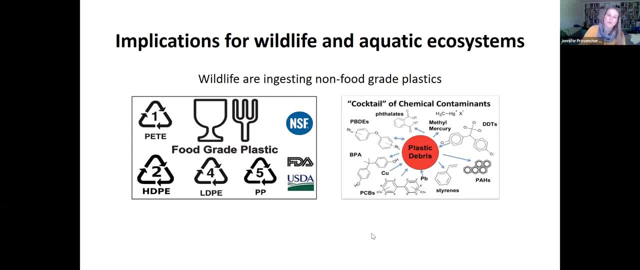 our polymer data is that the birds are actually ingesting a much wider range of plastics, And so they're being exposed to this cocktail of chemical contaminants, and it kind of hitched the ride. Some are part of that plastic and some of them are hitching a ride on those plastics. 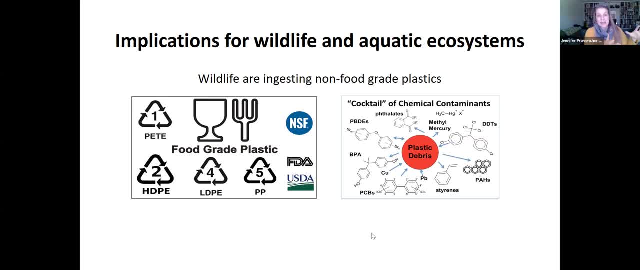 So we're dealing with both what I often refer to as the legacy contaminants, or contaminants that we can have no environmental contaminants, as well as these kind of plastic, additive plastic, derived contaminants. So you've kind of two groups that we're talking about a little bit. 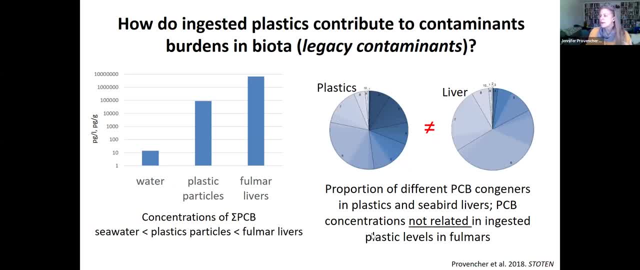 And so we've tried to kind of tease these two things apart. And so one study that we looked at- you know, looked at a few years ago- was PCBs, And so of course this is a legacy contaminant. These are contaminants that have been phased out. 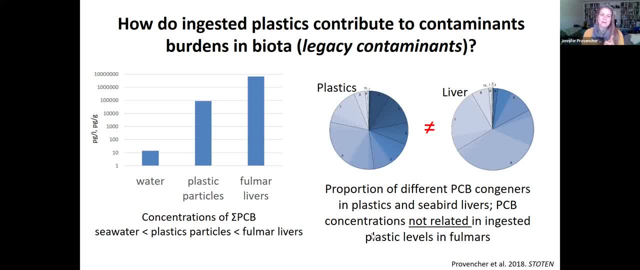 You know there should be no new plastics coming into the world with PCBs a part of them And we were able to look at, you know, PCBs in water and plastic particles, as well as livers, And we were really interested in if these birds had. 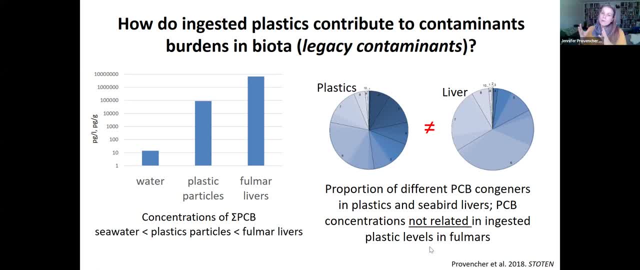 had kind of more plastic ingestion, whether those liver PCBs kind of reflected those same levels or the same congeners, And so what we find is that for the most part they're not related. So there's this paper as well as another one out of Norway. 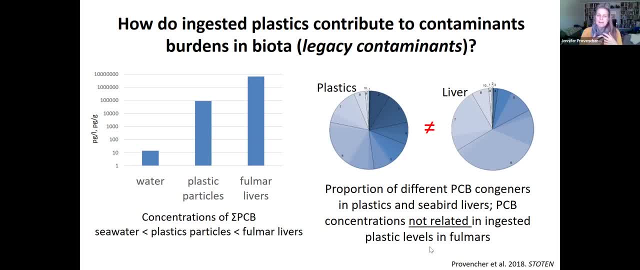 that really kind of shows that for these legacy contaminants, plastics are not a significant route- And that's not saying it's no route- but the PCBs, these environmental contaminants are in the environment, they're in the food chain, And so, while you know, 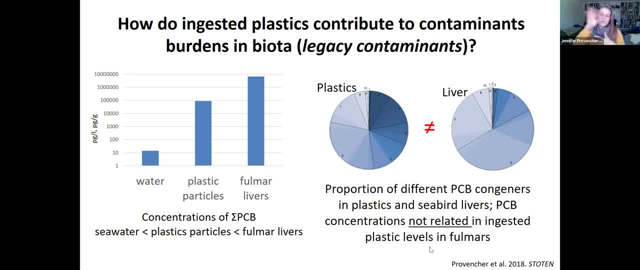 some proportion might be coming on the plastics. that signal is getting swamped out by the environmental signal And that's kind of a signature. So our current thinking on kind of legacy contaminants is that plastics is not like a really big driver, It's not going to be the primary route. 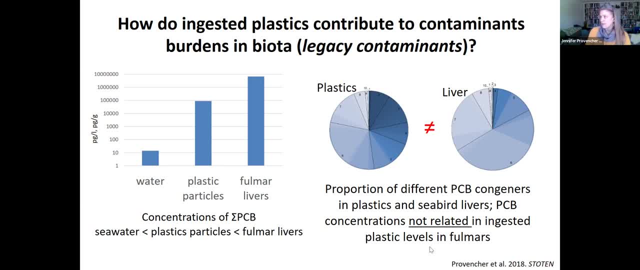 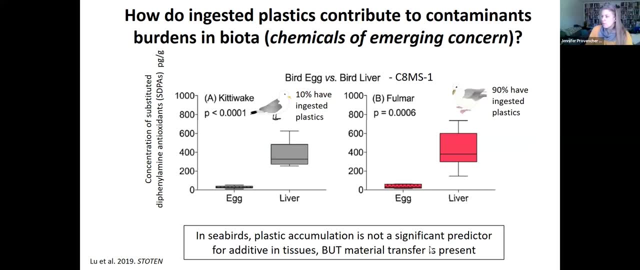 It's not a significant factor into the contaminant burdens for these, these animals. What we've been doing more and more work on in my work- And this is you know where Veronica's work has come into play as well as what about these chemicals of emerging concern? 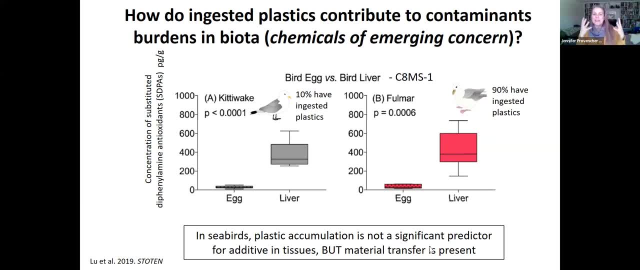 What about these plastic additives? right, These are things that have not been in the environment kind of previously. what do you know? what are the things that are kind of coming along with plastics along the way? And so we've done this now in. 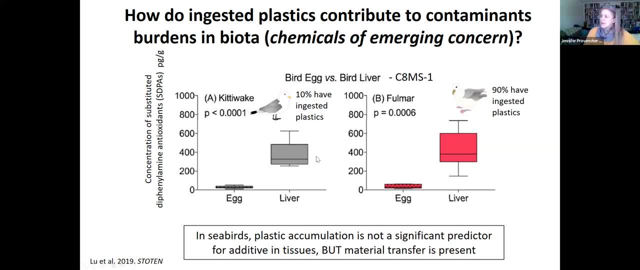 in seabirds and a few different studies. So what we did is we looked at the eggs and we looked at the livers of these two species. So kitty wakes is a gull, you know a species related to the gull. 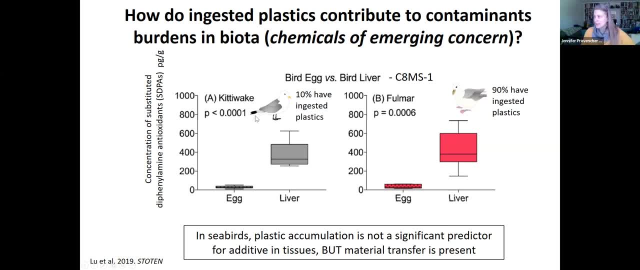 About 10% of the kitty wakes in Canada have ingested plastics in them. We also looked in fulmars and again, fulmars are also- sorry- also breed in Alaska. So many of you familiar, but they're more related to albatross- about 90% of the birds. 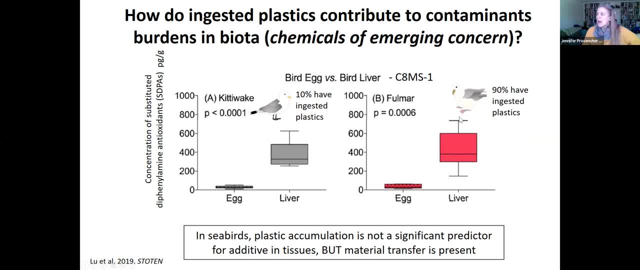 in Canada, breathing in Canada, have plastic pollution in them And I expected that the fulmars are going to have much higher levels of these antioxidants, which are plastic derived contaminants, And what we see is it's very little different. So the the the liver values for these antioxidants. 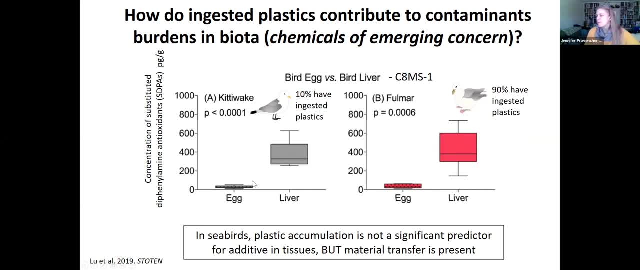 these plastic additives are are, you know, very similar. We see similar levels In the eggs, But I think the most important part that we take away from this is that we're finding them in the eggs, And so not only are these- 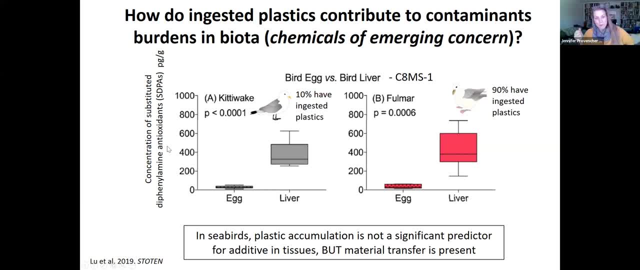 these plastic derived contaminants kind of ending up in the bird at detectable level levels in the liver. we also see from this that they're being maternally transferred, And this is where that effects question really comes into play, because a few of these are endocrine disruptors. 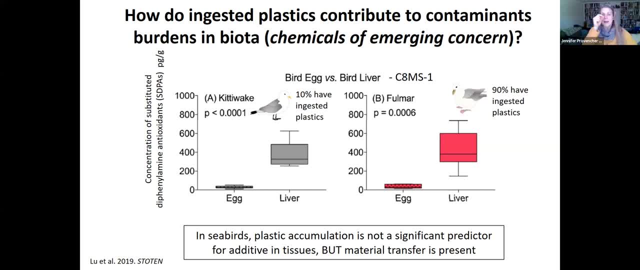 We know that it takes very small levels to actually have an effect on a developing embryo or or a developing bird, And so this is where it's. you know, this is our first kind of tweak that something might it might be happening here. 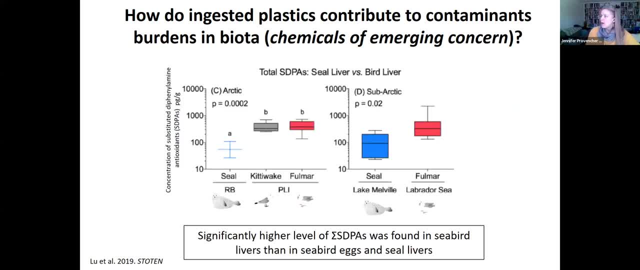 So we know that that maternal transfer is happening. We we've also done this same study in seals And so we use ring sales in in. there's two kind of locations: repulse, sorry, resolute Bay, and then Lake Melville. So we've got, you know, birds and seals from you know. 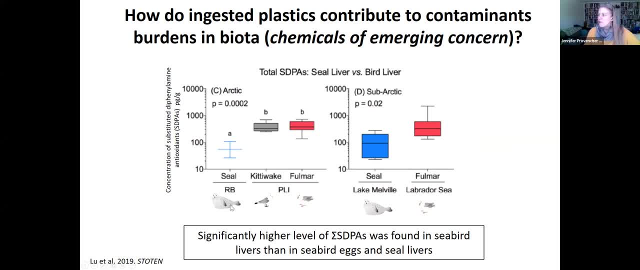 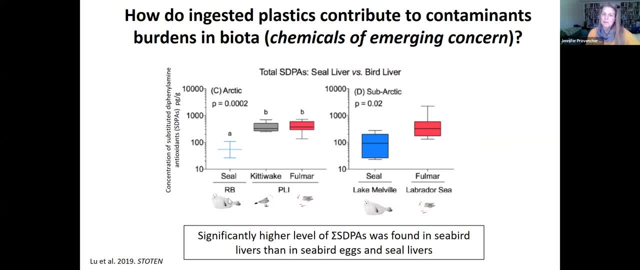 It's known to have a very joined. look on them again for April This year. These are two drilled animals And what we see is that, you know, interestingly, the seals have much lower levels. They do have some levels of these antioxidants. 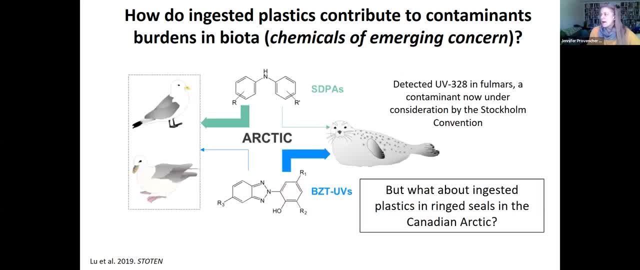 but they're actually consistently lower than the bird. So, really, pointed, the CB birds are having a higher exposure to these antioxidants or these plastic derived chemicals Then what we see in the seals, but it doesn't hold true for every contaminant, which is one of the things that we're we're learning. 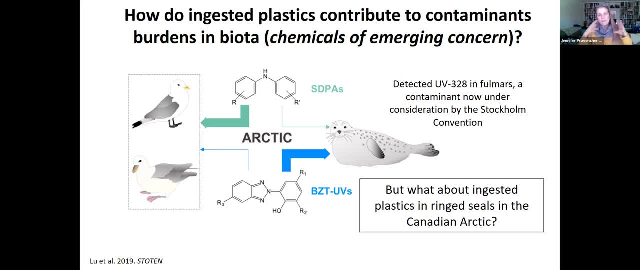 or in some ways receive. these all had kind of different behavior in different animals and different food webs, and so you know there's been a lot of work on some of those contaminants and now we're seeing that same pattern again in our plastic additive contaminants, and so we see our antioxidants. 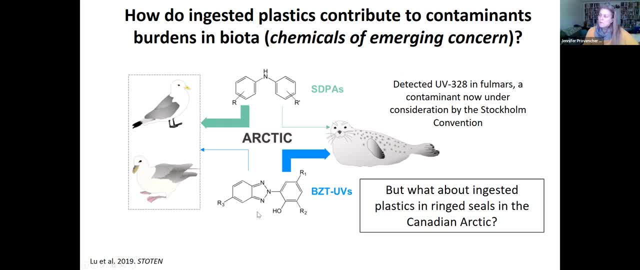 were much higher in these two bird tissues. but then when we look at the uv stabilizers that you know, a different family of plastic additives, we see much higher levels of these in the in the seals. and so two things i just want to kind of add is that uv 328 in particular is one of the 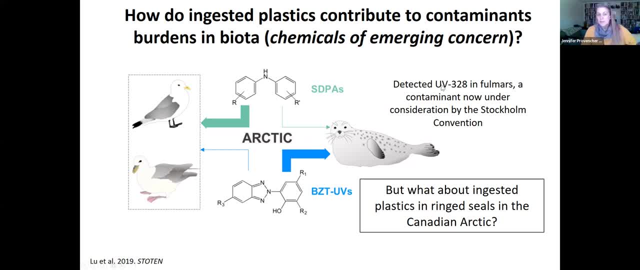 things that we've measured and this is now under consideration by the stockholm convention, so they are moving through their assessment, and one of the things that you have to kind of be, you have to have under the stockholm, is you actually have to have long range transport, and so one of the 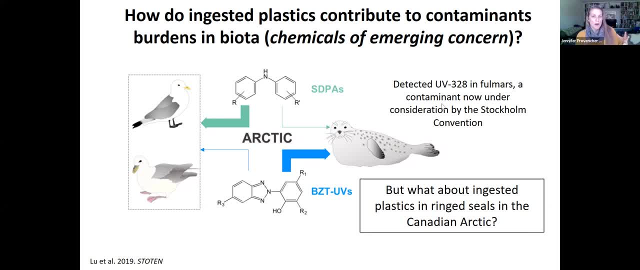 ways that the stockholm convention is kind of invoking this. long range transport is via seabirds, and so it's the birds moving the litter, moving the plastics that are actually kind of getting to the arctic and invoking that long range transport. um, but of course you know, this then begs the question about seal. so we, you know, 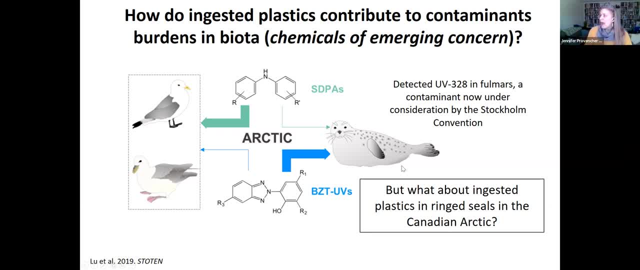 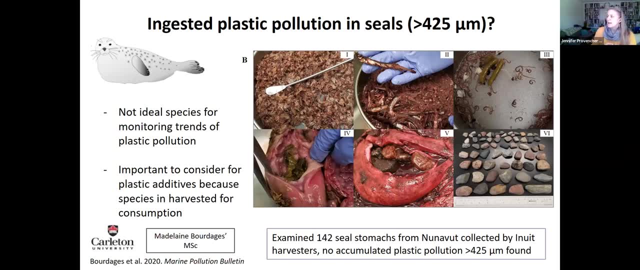 we hadn't really looked in seals but we were finding these plastic additives and so we we put out a call. we worked with five inuit communities across nunavut and we looked at a student of mine more, madeline borday. she looked at 142 steel stomachs. we put out a call. i thought no, maybe. 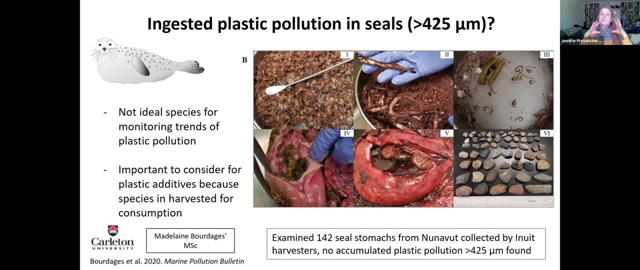 we'll get like 40, maybe we'll get 50. you know, poor madeline 100. you know poor madeline 100, 42 steel stomachs. later, um you know, she looked through it all, saved it all kind of at a one millimeter size fraction. um, sorry, it was 425 size fraction and she didn't find a single piece of. 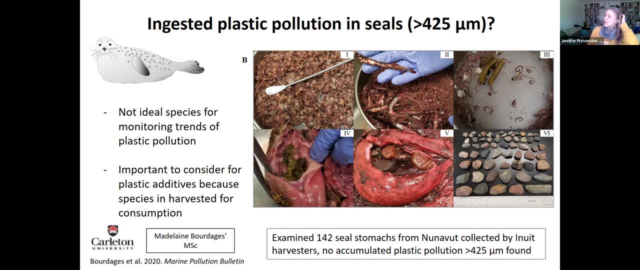 plastics. um, which is really interesting, um, you know, because we, we they have plastic additives, so we fully expected them to have some type of plastics in them. she found a lot of things, you know, a lot of ephazids. all of these rocks are all from one one steel. i don't know what's happening. 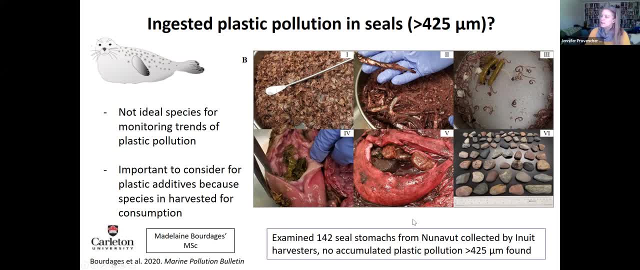 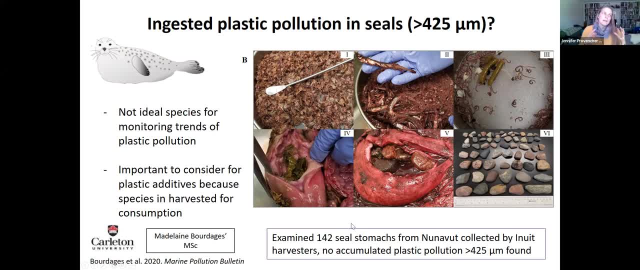 and so i think that this is really demonstrates that these animals can have these chemicals without having the accumulated plastics, and so either they're eating things that kind of have plastic additives in them, or they're consuming plastics again, probably through prey that are so small they're just kind of really moving through the digestive system so they're exposed. 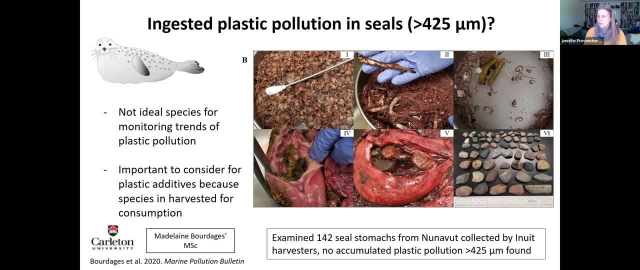 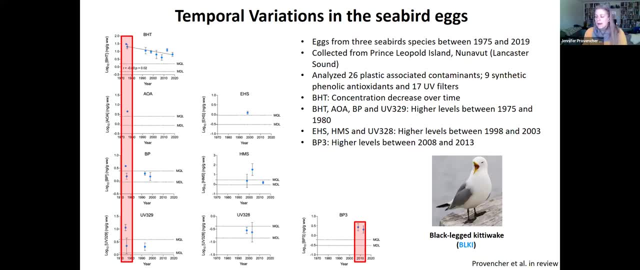 for a short amount of time, constantly, but nothing's accumulating, like we said, and so it's really interesting to see what we see in the bird's stomachs. we've also looked at more recently at some of these temporal variations. so in canada, my predecessor in my position, dr 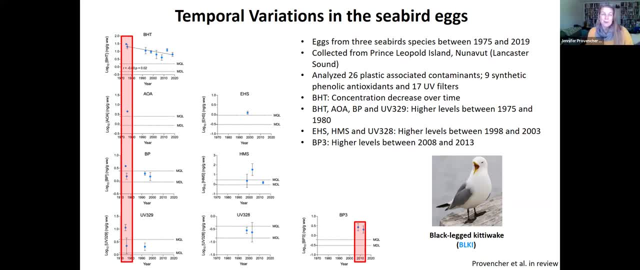 burgett braun. she worked with environment and climate change up until about two years ago when she retired, and she was in charge of this long-term monitoring program for contaminants in seabird eggs, and so we have eggs in our in our archive that date back to 1975, and so that 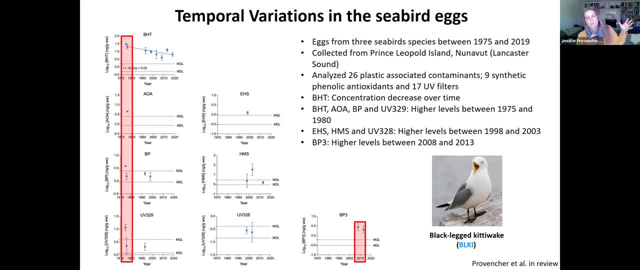 actually allows us to go back and look retrospectively and look at what's happening in the wild that we're seeing and we see how the, the other species that we've identified are relatively Effectively for the emerging contaminants. and this is the the whole reason for the specimen bank that we have at the national wildlife research center, and so we're 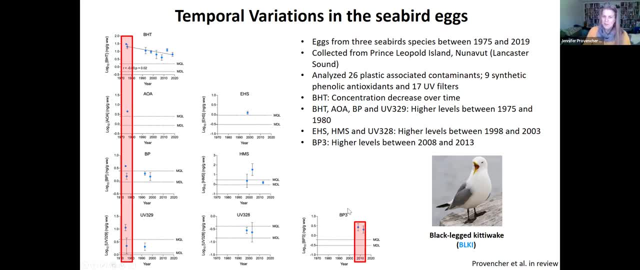 able to go back to 1975 for for a couple of species. I'm just showing the kitty wake data here and and we were able to kind of look at what these trends are over time and we actually do see that some of these additives are are popping up even in the samples from. 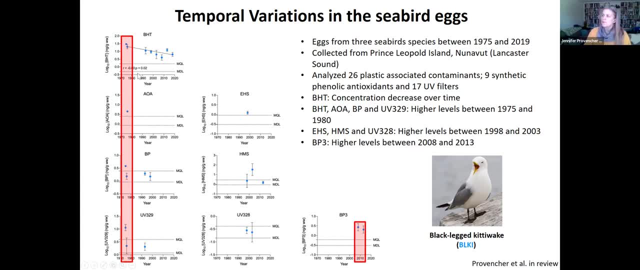 the 1970s. there there's no kind of real trend. we see a trend that we might see an adelphi and as we go the neon. we see that the more the more seen and as we go to the new species trend here with bht, but this is the only one that we see, um, you know, some of them have higher levels. 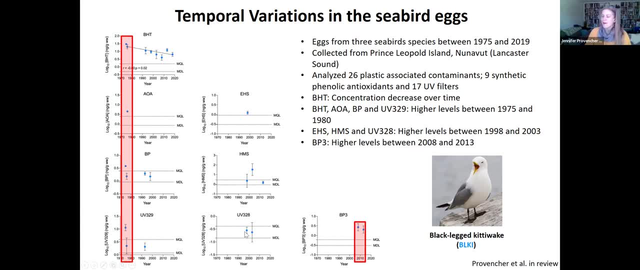 kind of looking at the 90s and the 2000s, it's kind of difficult to tell there's only a few spots. everything else that's not on these. uh, you know, below these um graphs are basically levels of non-detect, so they were so low that we couldn't detect them. but it is interesting that we see. 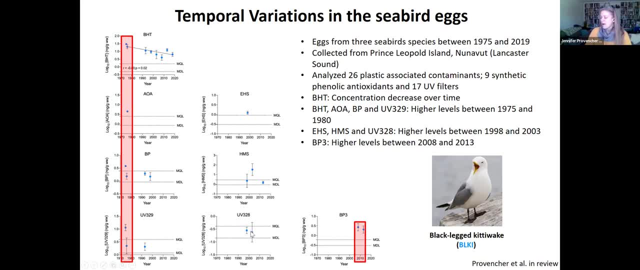 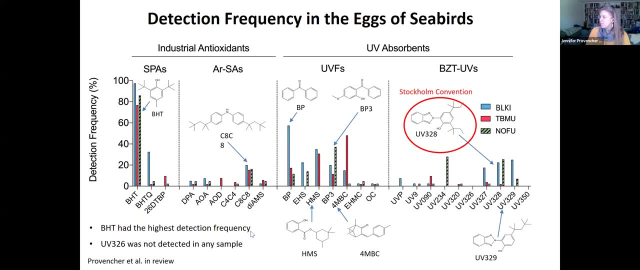 this uv 328 um pop up and we do see the higher, higher levels kind of previously. so this is something that we're working on and we're continuing to work on and track uh trends in, just kind of to zoom out a bit. um, so we do. we did look for a wide range of of contaminants. 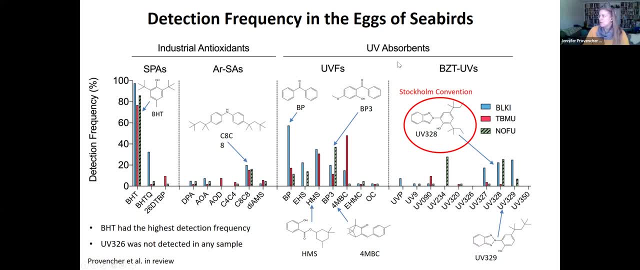 and we looked again at these industrial antioxidants and the uv absorbers, and again i'll point out this, uv 328- this is the one under consideration by the stockholm convention currently, and we did detect it in all three species of eggs, and so you know lab studies. 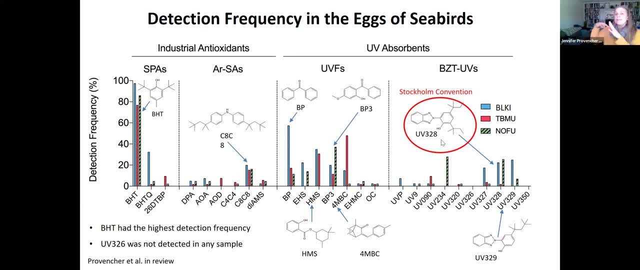 are kind of confirming and kind of um kind of examining the toxicity of this contaminant and the the role that our program plays is, you know, what are the actual exposure in the wild and what does it look like at these hierarchic sites? so this particular site is in, is in um, is in lancaster sound. so prince leopold island and 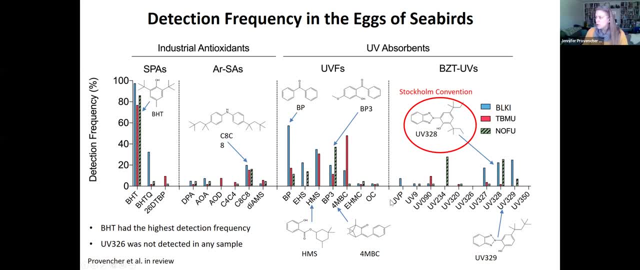 this is where we have a long-term, a long-term site. there are very few uh contaminants that are not detected in any of the samples, and so uv 326 was one of them, but again we're. you know we're getting hit that for at least um in most species. 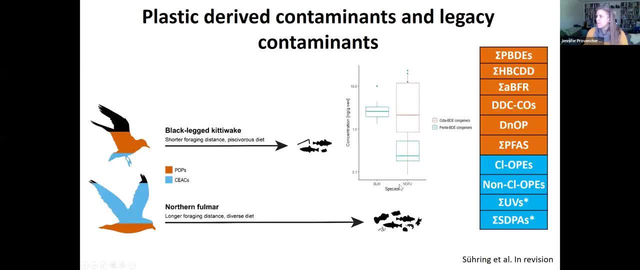 for for these um contaminants that we've looked at um again in this kind of idea of like well what you know, what does the emerging chemicals look like? in relation to these legacy contaminants, we have done a recent study where we looked at a whole suite of these contaminants and for those, 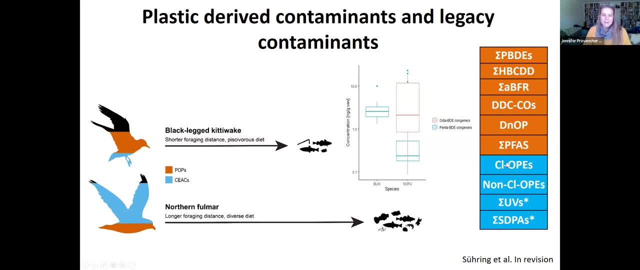 of you who are, you know, not kind of a toxicologist aside. um, you know, each one of these, this is the thumb of pvdes. each one of these has multiple things that are being added together. so these are, these are families of contaminants that are not infected, and then you know what's happening when. they start to become industry-level contaminants. and then you know what's happening: when they're getting more and more as you're getting more of these, the transfer of contaminants, and oftentimes they will get more contaminants that will be added, but we don't know exactly what's going on between. 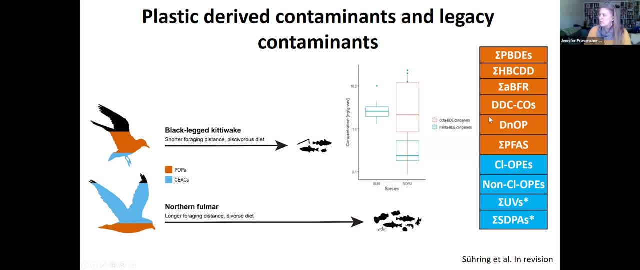 these contaminants and we're hoping to see if there's a chance of a potential nutrient that we can analyze and group them together. these orange ones are kind of these pops. these are more of the legacy contaminants, the persistent organic pollutants the blue here are. these are um are more. 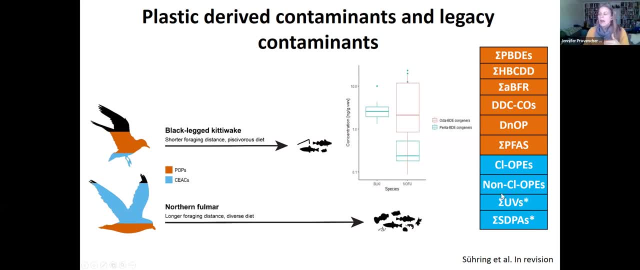 kind of um chemicals of emerging arctic concern. uh, they're listed in some of the amap reports on um emerging- sorry, chemicals of emerging arctic concern and often are related to plastic pollution or can be used in plastics, and so we see that um. you know, when we kind of sum it all up like this: 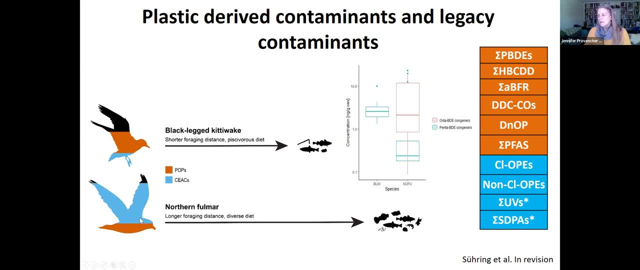 what we actually start to see is that these northern fulmers, these long distance foragers, this is the species that have higher levels of plastic. we actually see higher levels of these chemicals of emerging arctic concern. these are the plastic additives and when we look at the kittywigs you know they've got some, but they actually primarily 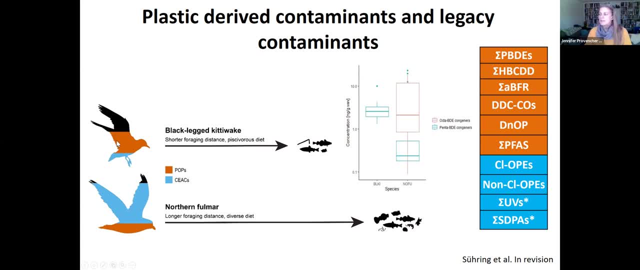 mostly have these legacy pops and so there is a difference kind of between these two species. but it can't be done at kind of a contaminant by contaminant by contaminant um perspective. you know, we're trying to think about it like a more holistic perspective. 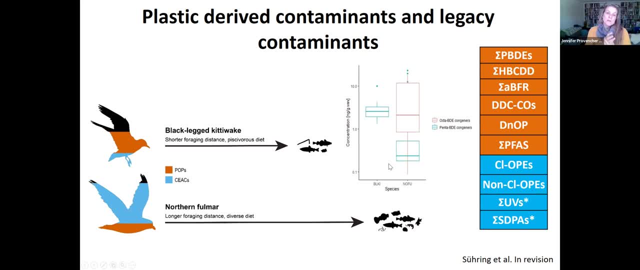 and and the one contaminant that we actually found- an association between those birds that had kind of plastics and not plastics- was actually um organophosphate esters, and so again we're we're still kind of trying to think about what are the contaminants that are found with plastics. 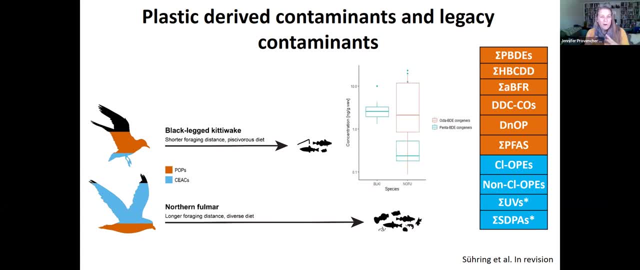 and what are those contaminants that we can use as a, as a marker or an indicator kind of exposure to plastics? and it's not necessarily always, always straightforward, um, but we kind of are trying these different um, different contaminants to see kind of where we land and what can be used for for that um use. i will put out there that i think might be of interest in. 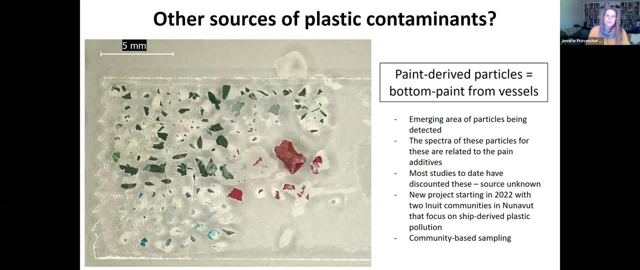 this particular group is that we are thinking about other sources of plastic contaminants as well. um, and this is where some of the work that we we started a couple years ago and actually just got funding for three years is looking at these paint particles, and so we're finding these in our, in our water samples. um, we have several communities. 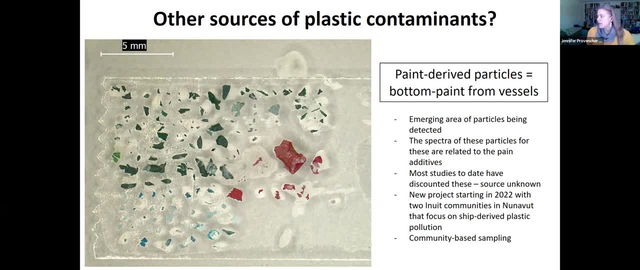 that we work with pond inlet kikitarjiwak and akviat um and they're finding finding these paint related plastic particles in their in the water samples in the national wildlife areas, and so we're going to do further work on thinking about what are the ship derived plastics that are 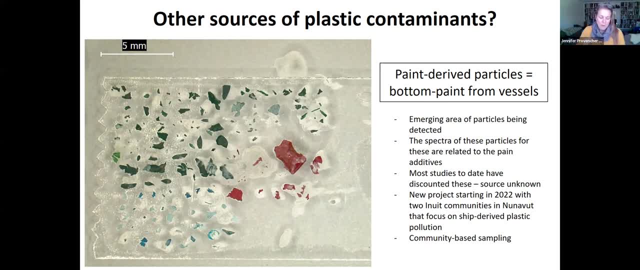 actually coming to the arctic and, of course, for those of you you know who know about bottom paint blades, it's sloughs off and the whole point of it is so that the invasive species are not kind of being moved around on the bottom of the paint. but what we're finding is these chips, these paint chips. 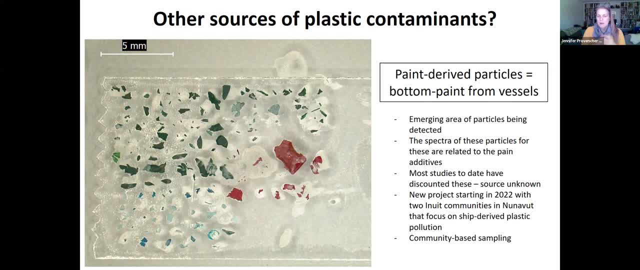 are ending up in the, in the water column and, of course, being exposed, or the bio are exposed to it and uh, from, uh, from a, and i'm happy to talk more about it, but i i will kind of get into it here, but from a, from a, a chemical or toxicology perspective, these are toxic to invertebrates. 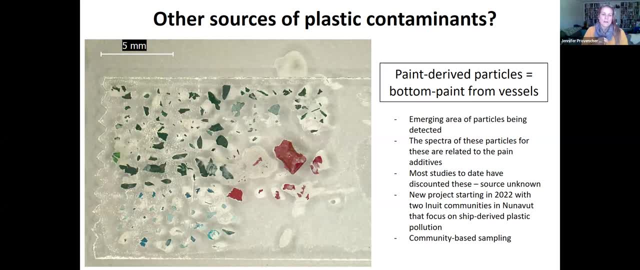 by design, and so there's that kind of aspect to the arctic and the arctic and the arctic and the that we're trying to thinking a little bit more again as we unpack the toxicity. So I will plug that we are 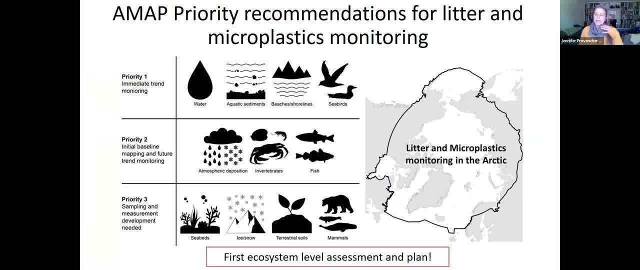 we have done this activity where we put forth an ecosystem level assessment and plan under the Arctic Monitoring Assessment Program, under the Arctic Council. This, I believe it's online. We're doing a special issue currently, So there is a special issue of about 10 papers. 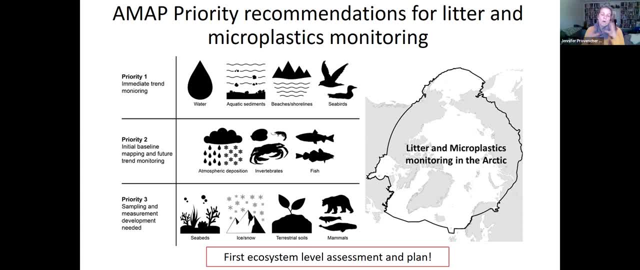 that are coming out and talking about kind of a monitoring plan and the compartments in kind of a couple of different formats, And so this is actually coming online as we speak in Arctic Science, And so I'm happy to share the link to those that are available online. 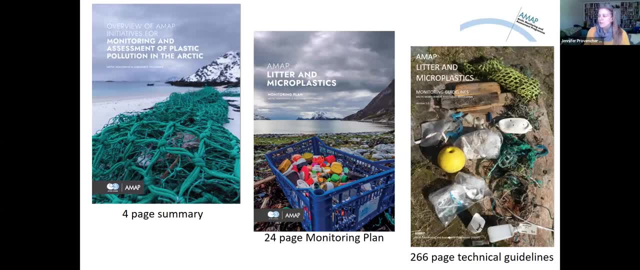 And again, if you want the long version, I can point you in the right directions. There's the four page summary for the quick read And then, for those if you really wanna get into the details, there's the 266 page technical document. 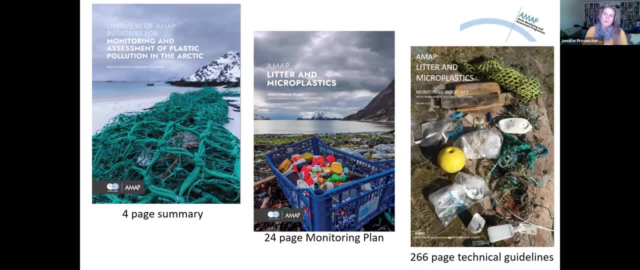 that we can point you to. But the goal is is that for those people who are either very deep into plastic pollution, as you know, Peter, I'm sure you've heard of it. Peter talked about the community or kind of. you know, coming in for a little bit. 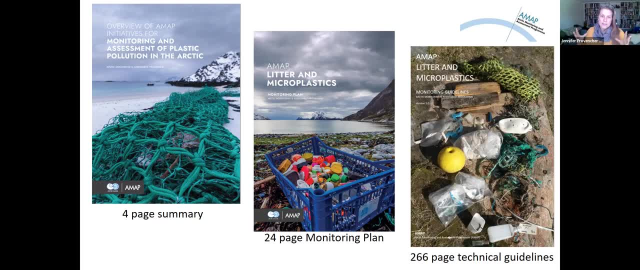 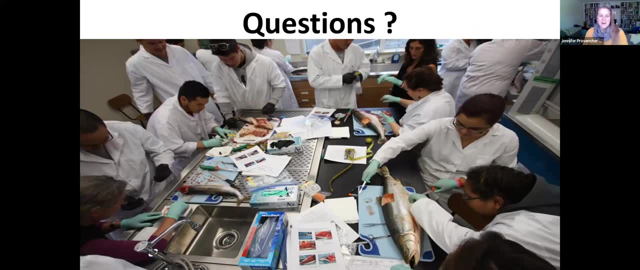 and then kind of coming out again. the idea is to get us all on the same page, collecting data so that we can actually start to look at, you know, spatial and temporal trends, And that is it. Thanks for listening and I'm happy to take any questions. 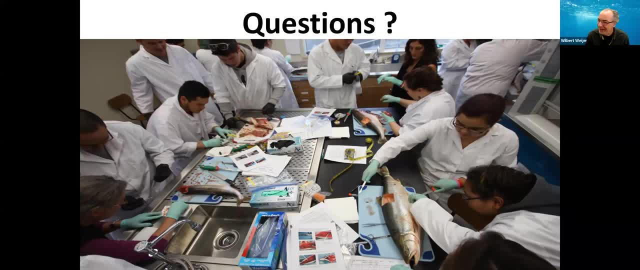 Awesome thanks, Jennifer. It's very, very complex topic, obviously Wonderful way, wonderful for you to present it in such a clear way, even to you know, non-specialists- physical oceanographers, for instance. excellent. So we're running a little bit late. 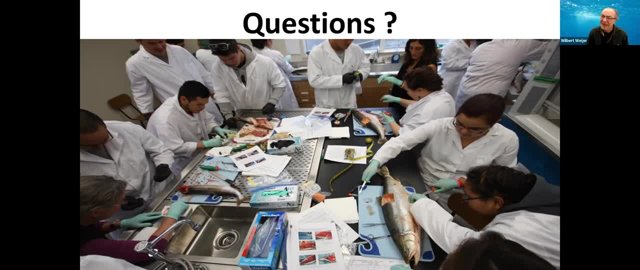 We got 10 minutes on the clock. Meredith tells me that we have a little bit of time. We can go a little bit over time. So I wonder if we hand it over to Veronica a little bit and ask her to present a couple of slides. 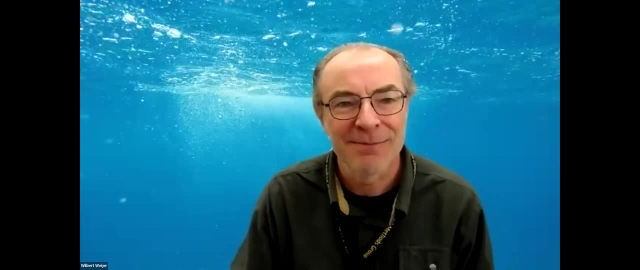 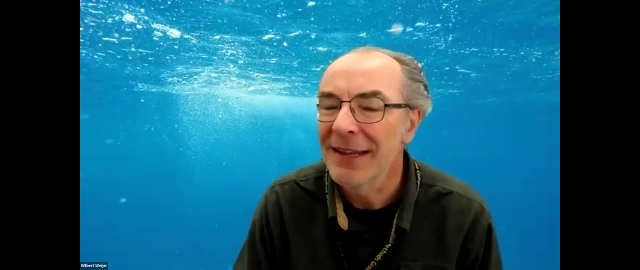 on the projects that she's working on and then opening up for discussion. And again, please feel free to ask questions to Jennifer and to Peter in the Q&A. Veronica, Hi, so I'm almost at my office. I decided to walk out this morning. 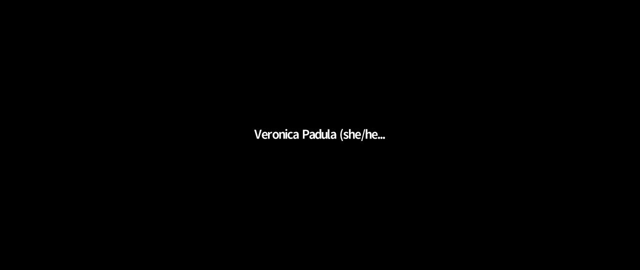 So once I do get them I will throw them up or else I will share them in an email later. But I can do sort of a quick overview of some of the work we've been doing regarding the plastic band issue on St Paul. 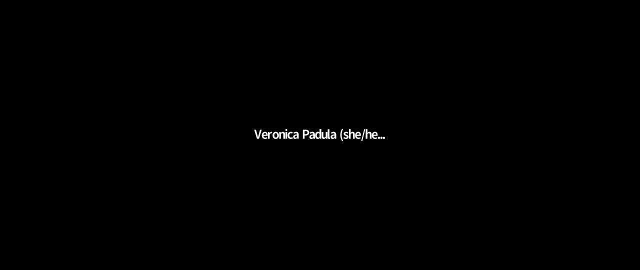 For St Paul Island itself. it has a large population of northern fur seals which are both culturally and sort of like resource important for the community, and they are very, very at very high risk of entanglement both in nets and in plastic packing bands, and so our idea was around trying to like, like peter said, 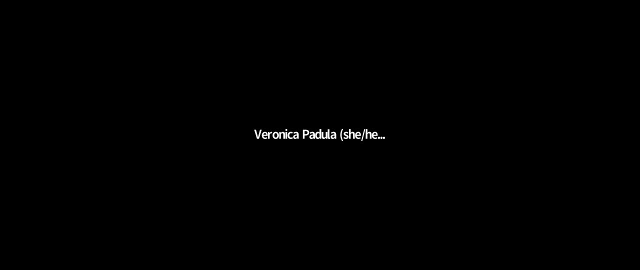 target something very specific and target a very specific behavior to at least prevent um so much entanglement from the plastic packing bands. and so our initial thought was to work with the community and sort of investigate what their behaviors were around disposing packing bands, because, you know, in some cases you could just rip off the loop off the box and then just throw it. 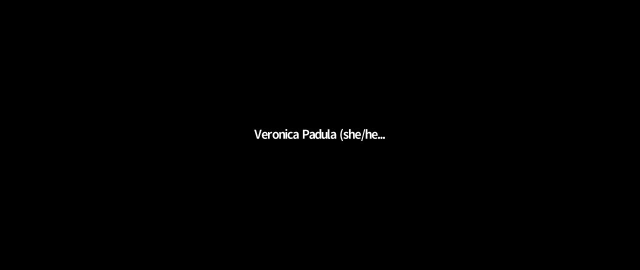 away and not necessarily cut it before you dispose of it. and what we found in our focus groups was that, um, you know almost everybody we talked to they already do that, and so we're like, well, okay, so we have to think a little bit bigger. and so our next: 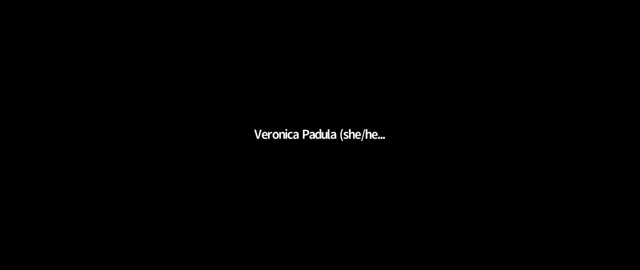 steps are really thinking about, um, the sources of the packing bands, which the community provided some examples to us and we figured that would be a great starting point for us in order to reach out and have conversations with people and think about how folks might consider using either fewer, 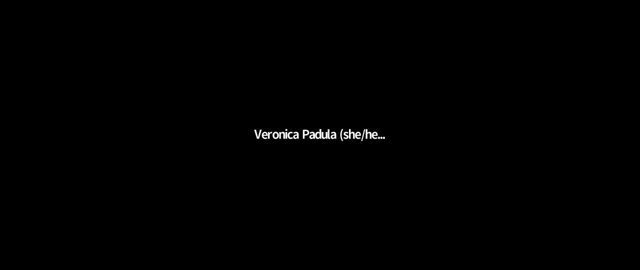 packing bands, no, packing bands replacing the type material, and we definitely stand on the shoulders of giants in terms of um, kim ramsurian and the peg group to have these ideas and sort of have this network already started? um, and we just kind of want to take it a step further and see what we can do, because 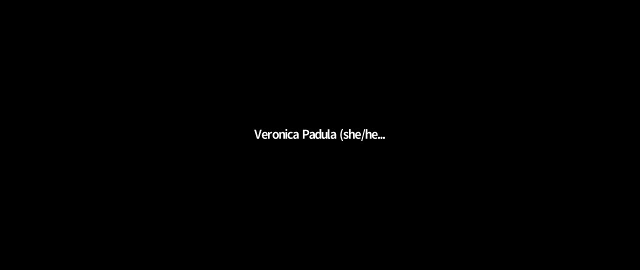 saint paul, you know, is a. it's a small island in the middle of the bering sea but is also a major spot for commercial fishing. we have a lot of crab boats come through, we have halibut, we have a lot of fish processed directly on island and fish boxes um are wrapped in the plastic packing bands. 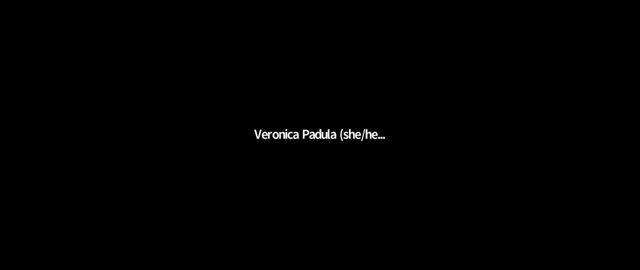 and so you know it is a community-wide effort to sort of change the story a little bit and see if we can really tackle this um, this one particular issue of plastic packing bans, in hopes that we can also sort of have a ripple effect. and you know these companies that are: 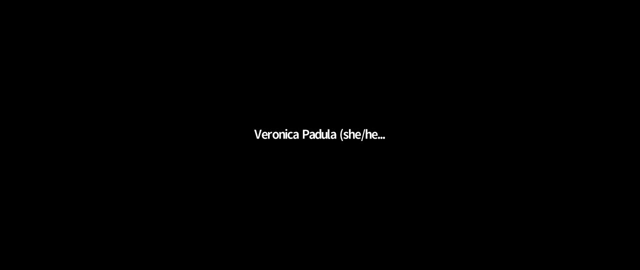 sending packages to saint paul aren't just sending packages to saint paul. there are other communities in alaska that receive packages from these companies and maybe we can sort of have broader impact as we reach out to more stakeholders and more participants in the work. so, um, you know that's. 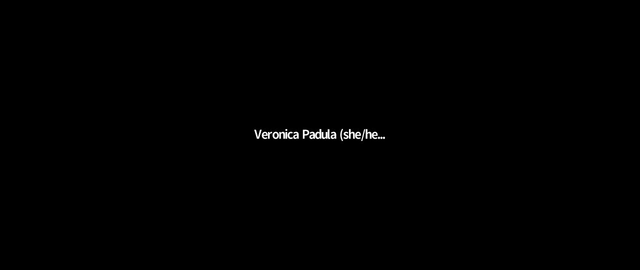 kind of the gist of it. um, it's a lot of a lot of boots on the ground just chatting with folks and and building relationships and sort of communicating properly. you know what the impacts of the plastic packing bands are and how we can make a change. um, so if anybody has 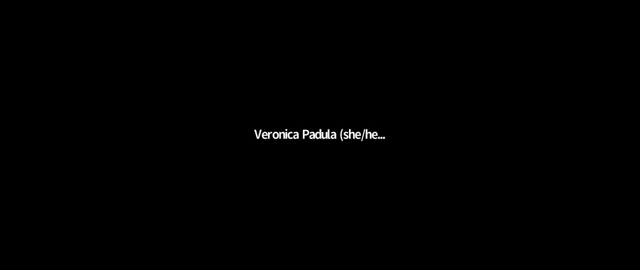 any questions about that. i'm happy to take them um, and i will. i'm almost at my, i'm almost at my desk, so i can share some slides very soon. i can also talk about the sea, the seabirds and the illusions and their plastic ingestion and contaminants as well, because, um, a lot of what. 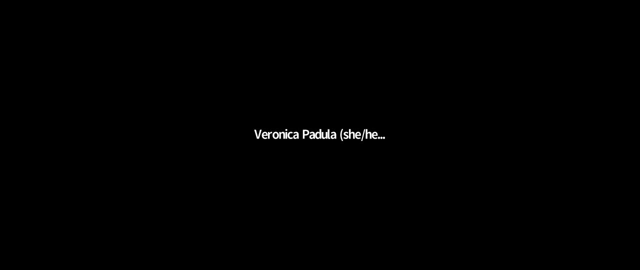 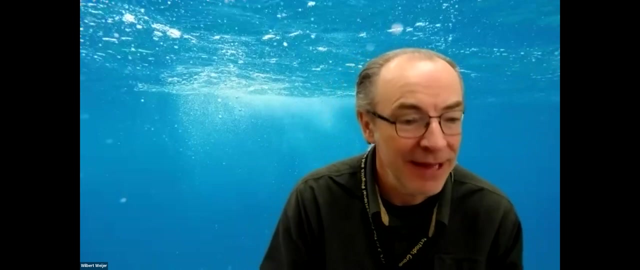 jennifer discussed is, um, you know, mirrored in what's happening with illusion, island seabird populations as well. all right, why don't we hold that thought for a little and maybe open up the floor for questions to, uh, to peter and jennifer, and, if there are any questions for you, for alika, um, so if you have a question, please, um. 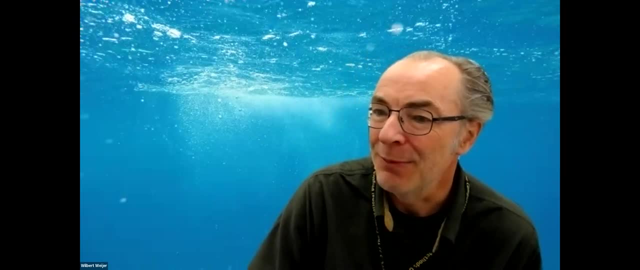 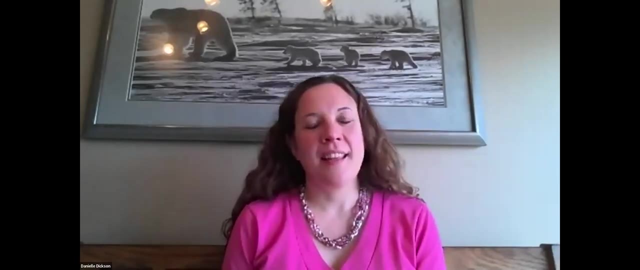 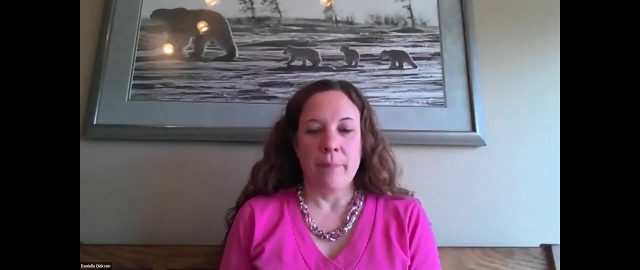 you can raise your hand or maybe um mute yourself too, i think. thank you, uh, both peter and jennifer, for your wonderful presentations. we really appreciate you spending your time with us today. um, i've got a ton of questions, but i'll just start with one, um, because we don't have very much time, and we'll see. 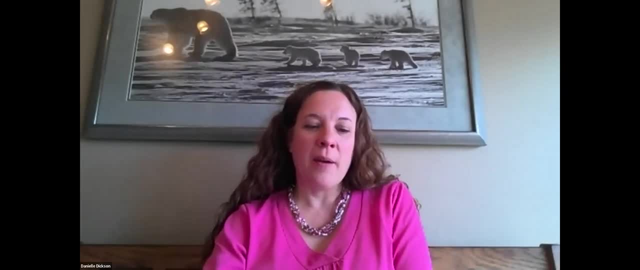 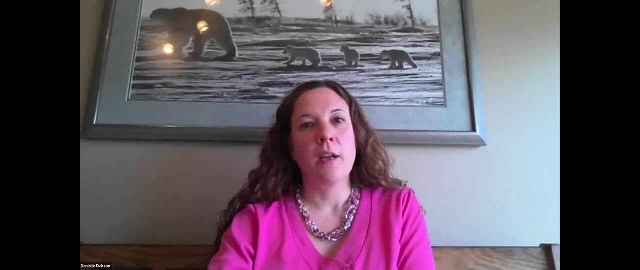 many other people want to add to the conversation. Peter, I wondered what sources of funding may be through your program at NOAA for people who may want to get involved and provide a little bit of money or some sort of incentive for either people's time or money to pay for the disposal of. 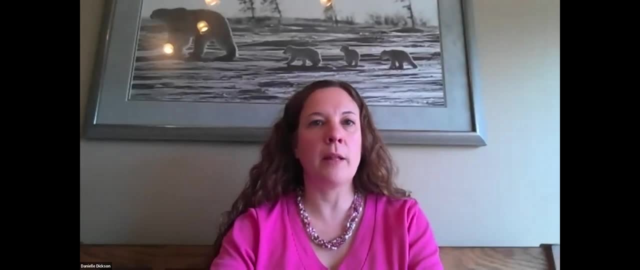 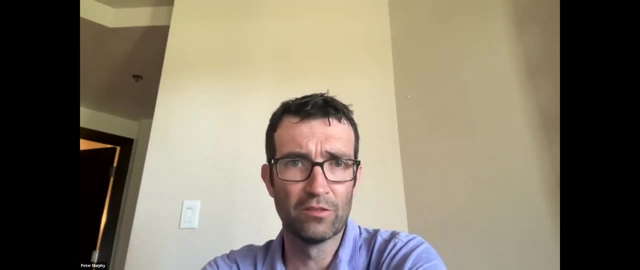 marine debris. Do you have a grants program and what might those opportunities be to let people know about? Yeah, of course. So there's a few different funding mechanisms or grants that the marine program typically provides every year, And you can find those on our web page. I'll 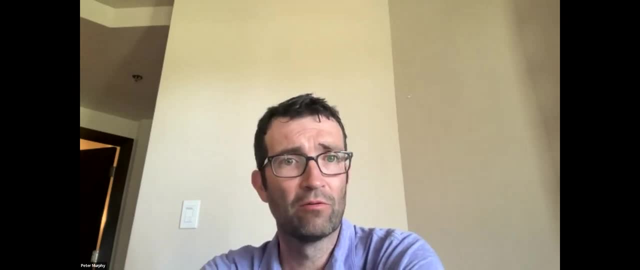 find a link in the chat in just a moment. But primarily they're around removal and then every year, and then research and prevention alternate years. Research is around typically a few focused research questions, whereas prevention is around kind of specific debris types or topics. 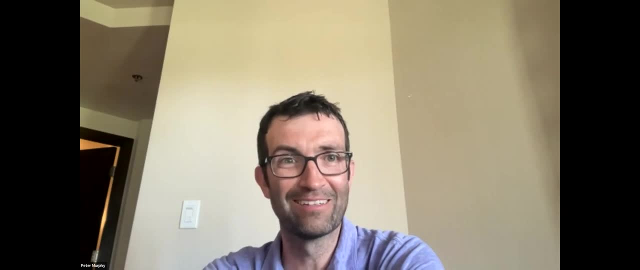 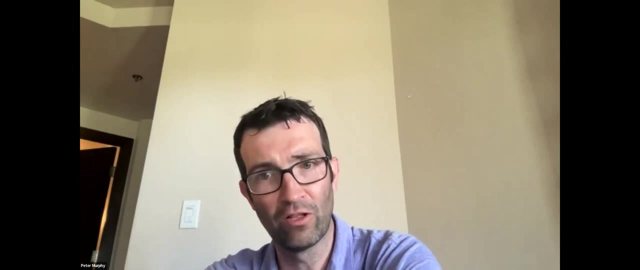 Of course, as we all understand- unfortunately, I mean the federal grant- timing is challenging And so those are long lead times to applications in the fall for award the following summer, And so that can be challenging, for, as an example, in the Bering Strait, Debris. 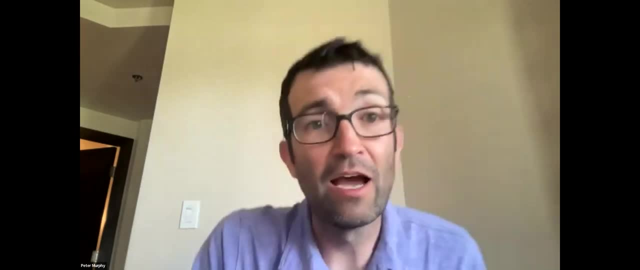 event, when you have something that's happening, right then. But generally, yeah, those are the things that are out there. There are competitive, So we get a lot more interest than there is funding, But that is the nature of things. There's a lot more good work to be done than there is. 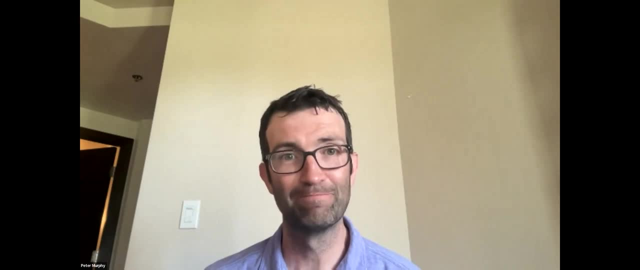 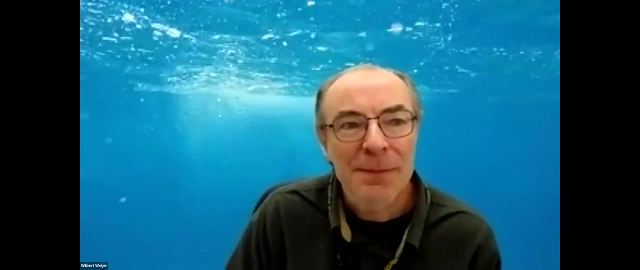 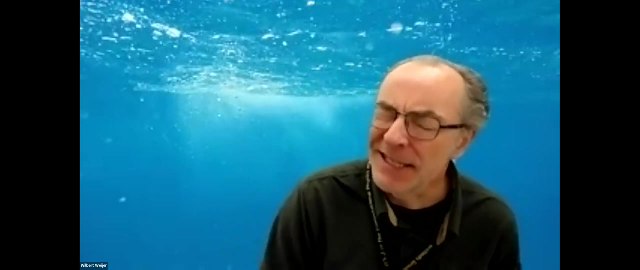 funding to support it. So those are things to keep an eye on. But yeah, Great Thanks. And any other questions, I guess I'll put one in myself. So you touched a little bit on the collaborations you have with other agencies. So do you see opportunities for expanding collaborations with other agencies? 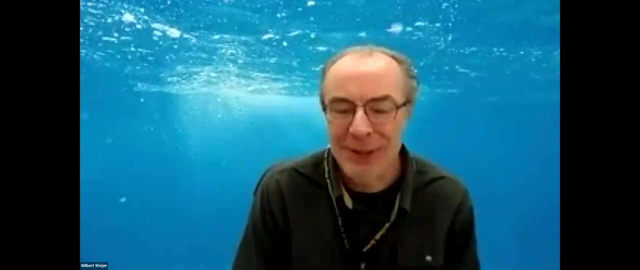 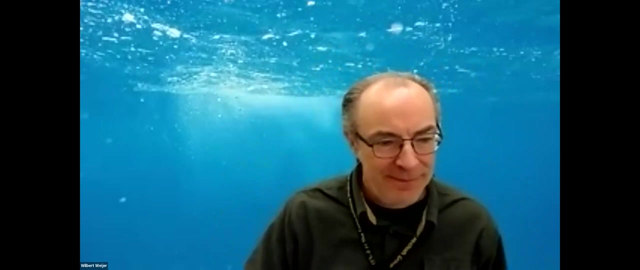 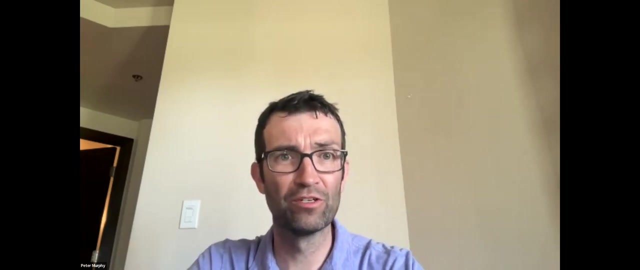 And maybe what role? is there a role that you could see IARPC playing in that? I'll take a quick stab at it. I think that, generally, collaboration is a good thing And I think that, especially now, there's more interest in more and more and growing interest. 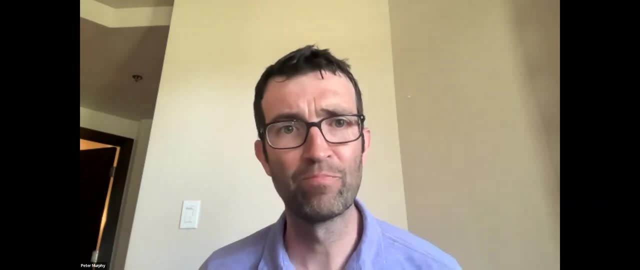 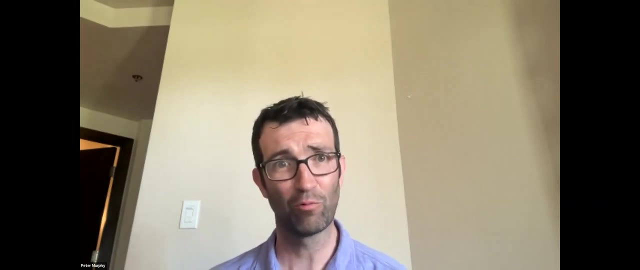 in the issue. I guess there's groups that have been working on this for a long time, But I certainly could see there being value in sharing information and people reaching out as they see connections between what they're working on or their interest areas and marine debris, because there may be connections that can be made, even if it's not for me. 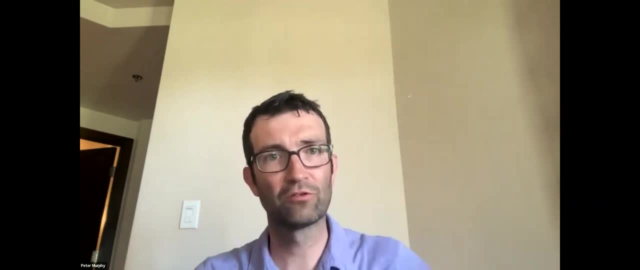 personally. So I'm interested in working out that as well. But then I think there's a lot of value: what rain reprogram is working on, but connections to- oh, there's this other group that's working on something that may have- um, may have overlap, especially, as you know, as many efforts are. 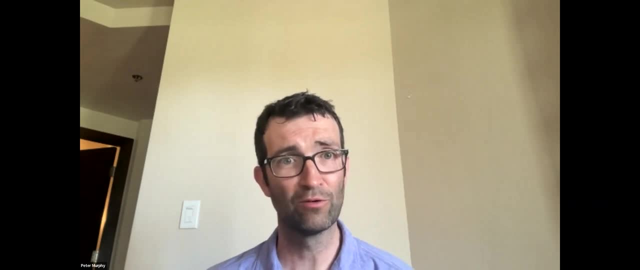 resource constrained um opportunities to collaborate and share information and insights. um can provide better outcomes as well. so i know it's kind of a general answer, but i think that um you know the short version. i think that there's the. there are certainly opportunities for continued information sharing, especially around specific areas of interest. 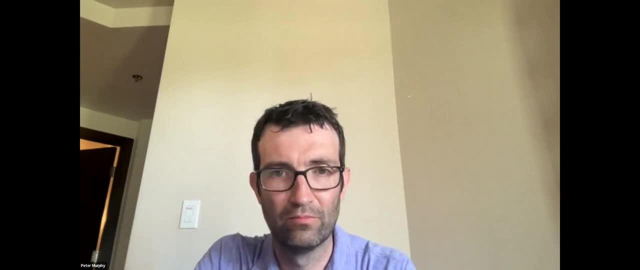 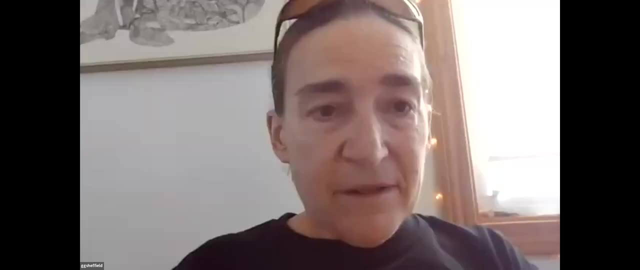 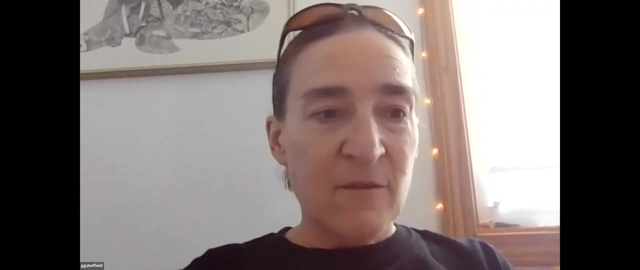 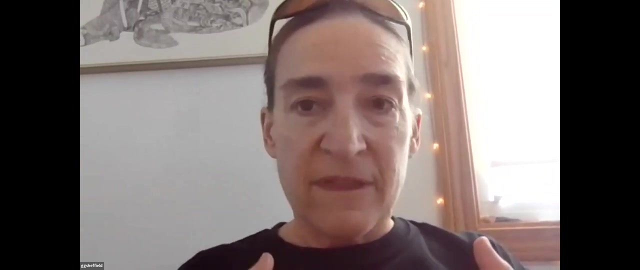 thanks and gg sheffield. thank you, gay sheffield. uaf alaska sea grant out in nom um wilbert your question. i guess i would say thank you, peter, and i would say you guys are international. we have the the something like the foreign marine debris event. one of the things with the arctic is that, as at least in our 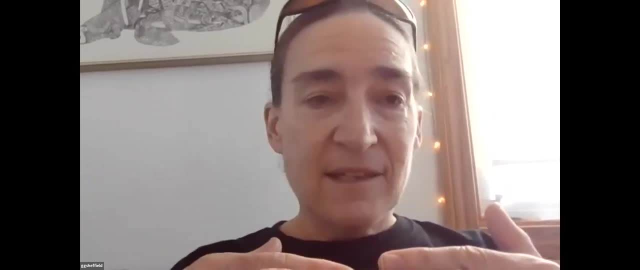 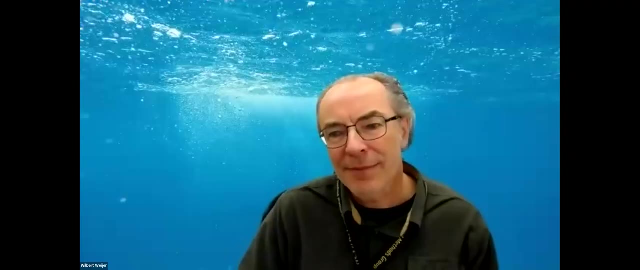 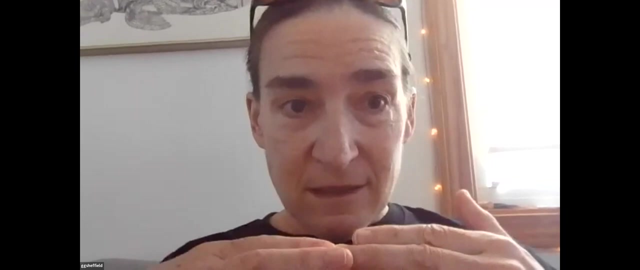 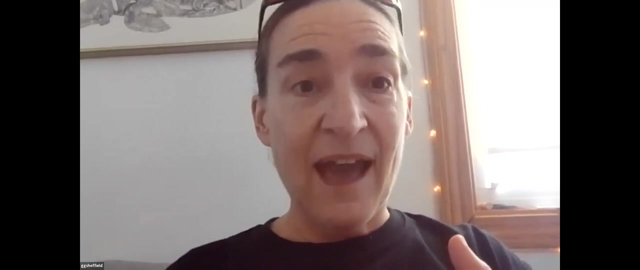 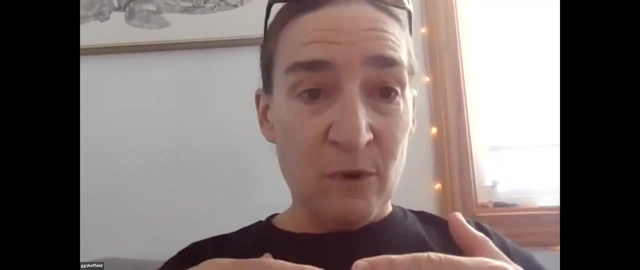 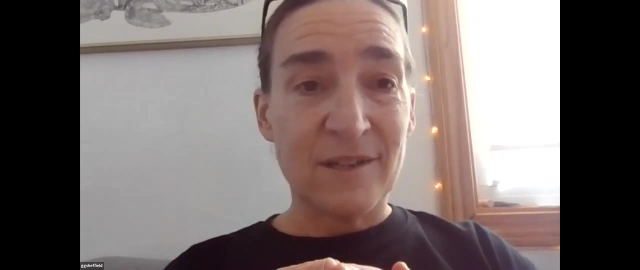 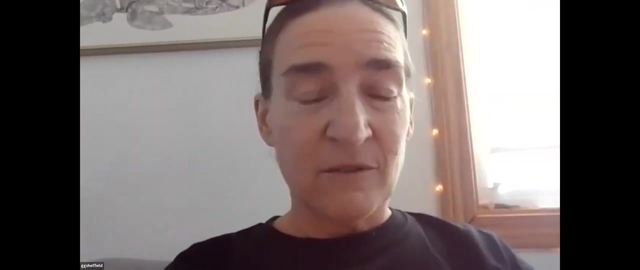 grow, and by that i mean the commercial fisheries are moving north and we're in a trans boundary area, the bering strait, with a very narrow entry and exit into the arctic, and we have the northern sea route and we have the uh developing the northern sea route across the top of russia for lng tankers and other oil tankers and all. 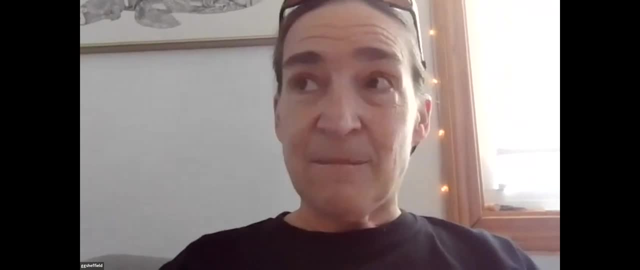 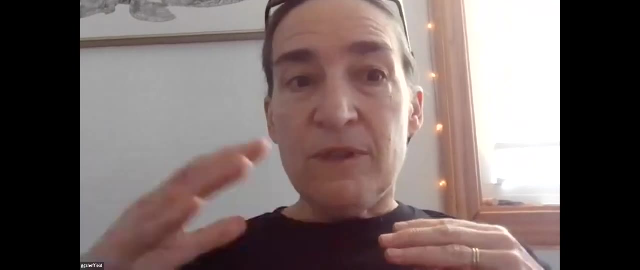 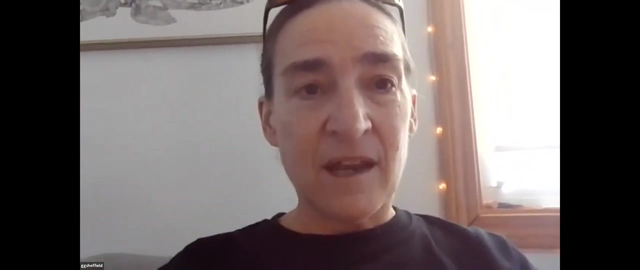 kinds of freight and fuel. we have the northeast passage developing through the canadian archipelago regarding cruise tourism and things like that. these are pressures um mouth. recipe technology and advance beta equipped systems has these kind of the uh uh, but i don't think uh uh, but i don't really think we're a Penny company. 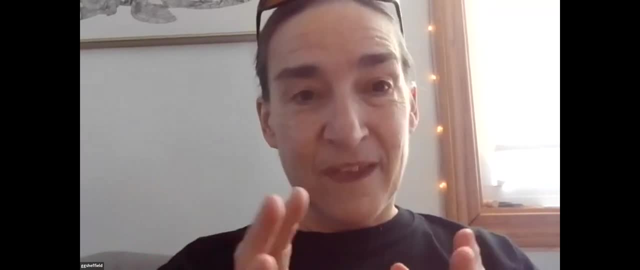 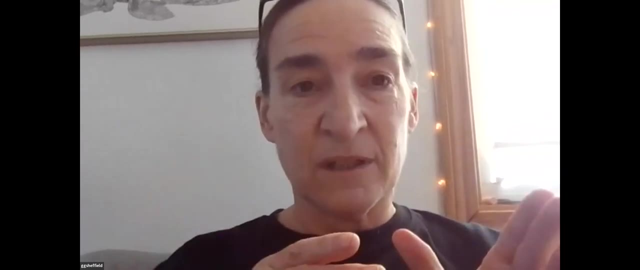 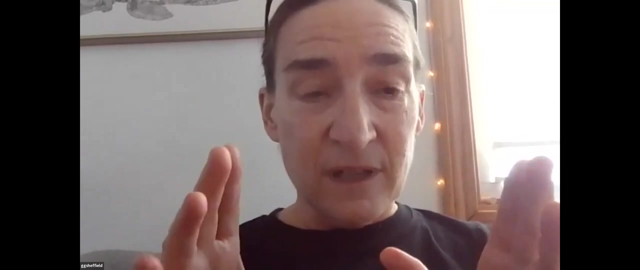 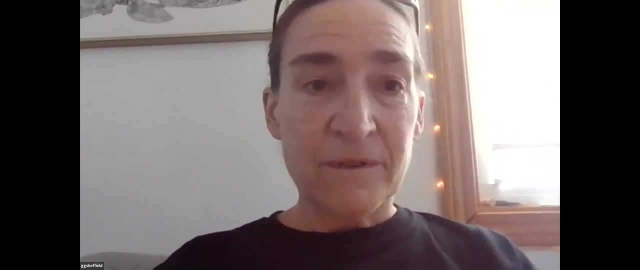 and we really don't think we can go the enormous down down. well, between anything like country ofでき, atakgga area, are really feeling all kinds of pressure And trash, marine debris is going to be, you know, if it's not. 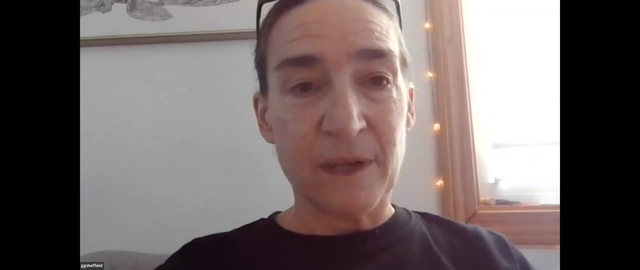 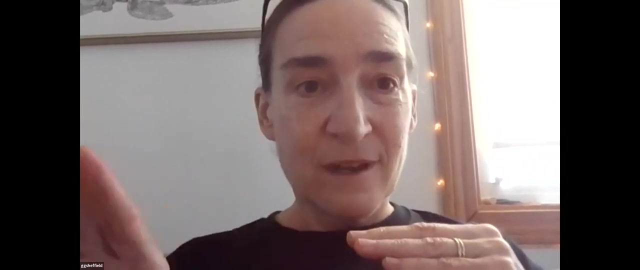 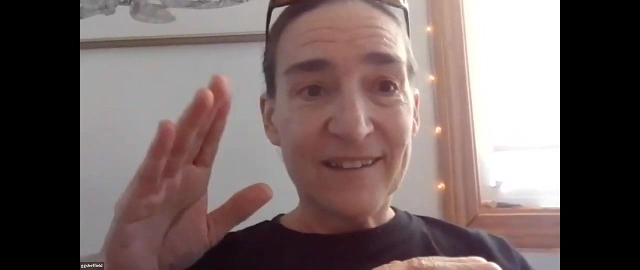 addressed internationally. it seems like we will just end up more And we're going from a time of really low trash, not fisheries so much, but foreign debris and the types of debris from low to high. So, anyway, that's how I would answer your question. 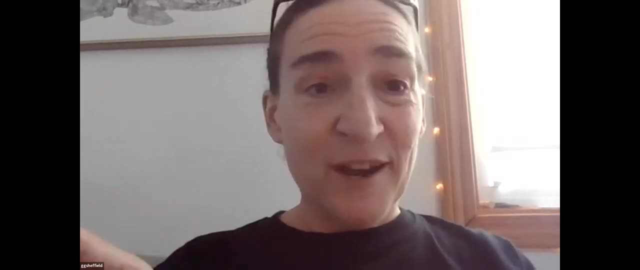 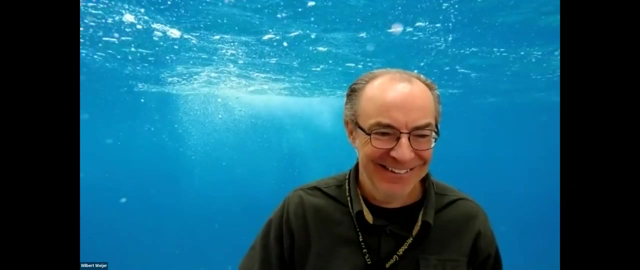 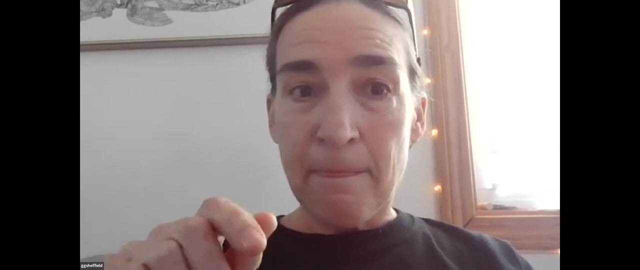 And I do have a question for Jennifer. Can I do that? Can I just switch and ask: Go ahead, Go ahead. Thank you so much about microplastics. Is there any work being done in Alaska? You're doing a great job in Canada and Nunavut. Yeah, I was going to say Veronica. 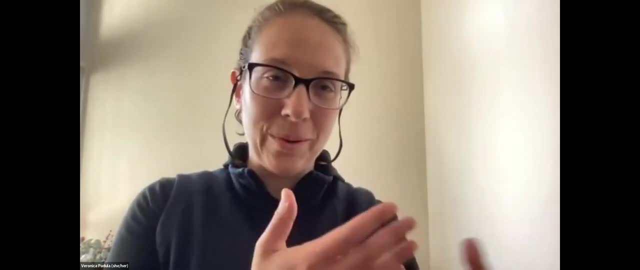 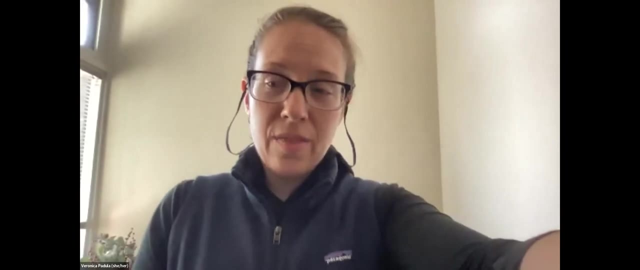 My PhD project's kind of coupled, looking at microplastics in seabirds in the Aleutian Islands, along with the sea birds in the Aleutian Islands. So I'm going to ask you a question, Along with some work on St Paul And there are other folks working on microplastics, kind of. 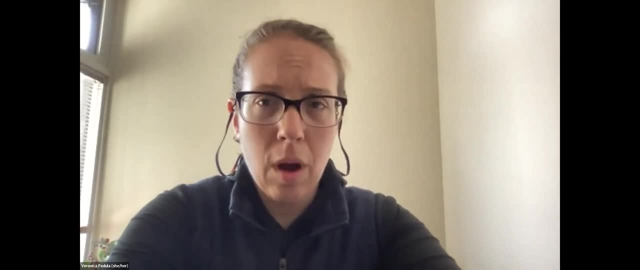 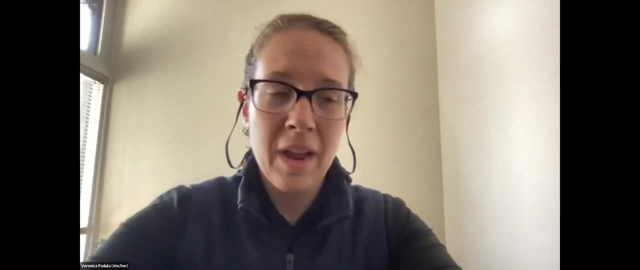 mostly out of the university, And so I could sort of- and Peter and I have been talking about this a little bit- of who's doing the research on this sort of stuff, But it is my intention to put together a list of who's doing the work. There's someone out of Juneau, which Peter, 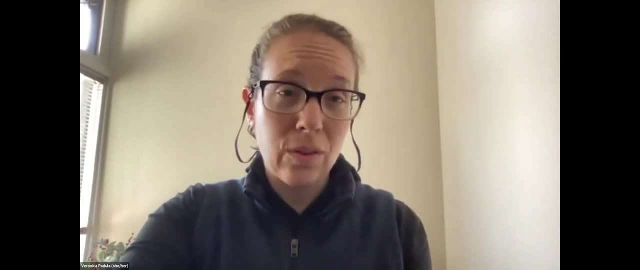 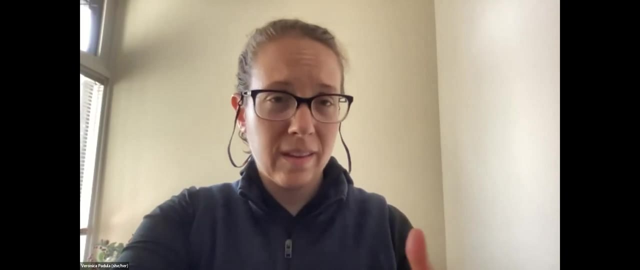 I don't know if you remember their name, but I can't remember their name. But there are folks doing it and working on it, Little bits and pieces. There was some work in national parks looking at microplastics and sediments. Also, I can put together a bit of a reading list for you if you want it and send it. 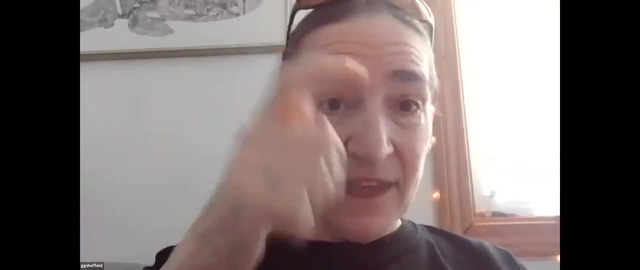 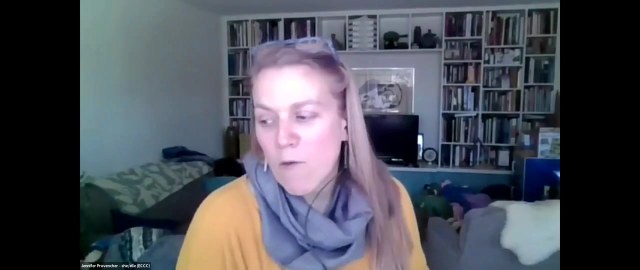 your way. Yes, please, That's awesome And thank you. Yeah, I would say, you know, I'm just going to plug this a little bit And it's not anything that most people haven't heard me say before. You know Europe, we've got, you know, the North Sea indicator In Canada. we've gone ahead and 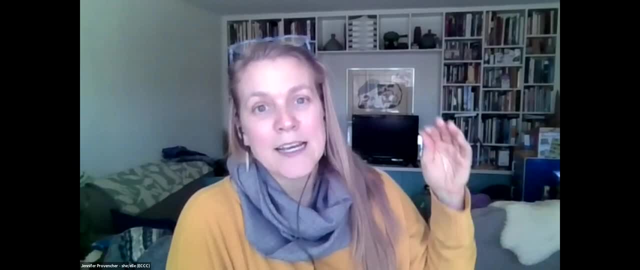 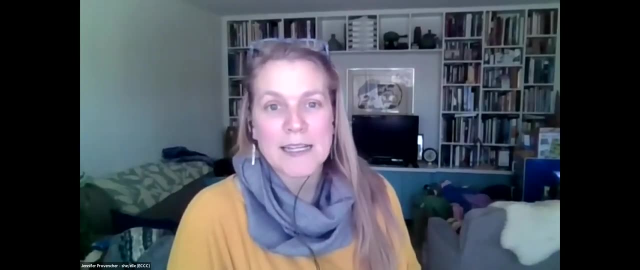 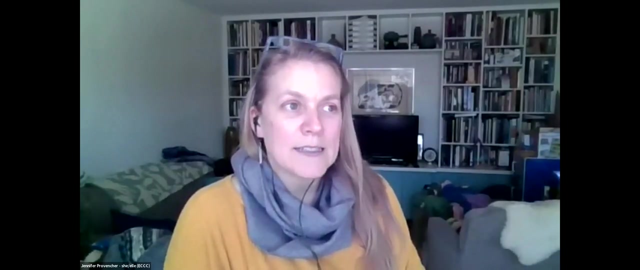 put the FOMARS as our Canadian Environmental Sustainability Index. The US is lacking on that. You know we don't have the. you know we don't have the partner data that we'd like to out of the Pacific And we've done a few reviews now on where that data sits. 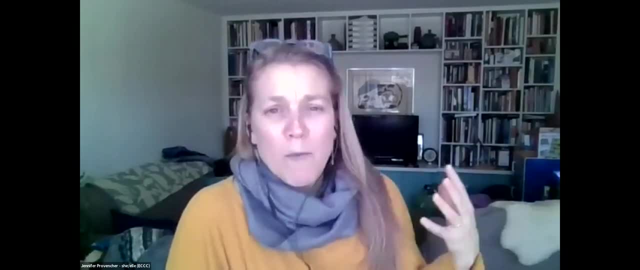 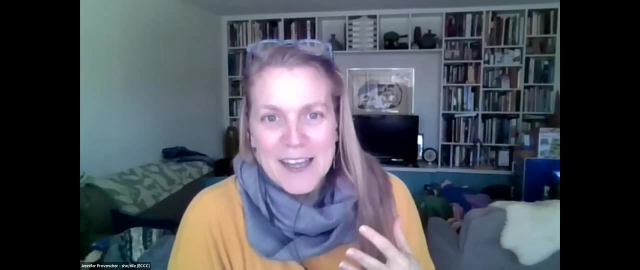 And you know from my perspective. you know there's a lot more mammal data, which is great, but the data says that they're not super susceptible, And so we're lacking data on species that are probably the most susceptible to the FOMARS. 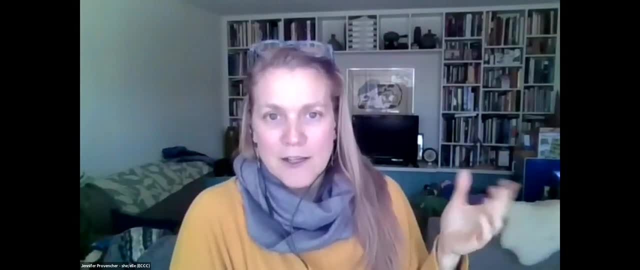 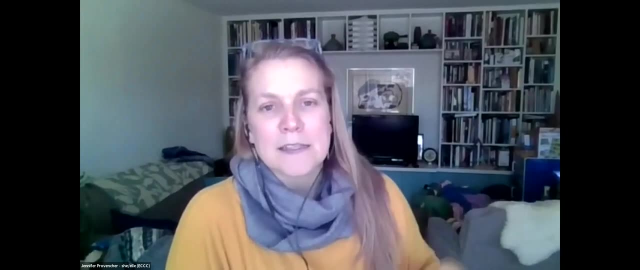 Physical plastics, chemicals- different story, ongoing discussion. But you know that from our. you know we've got Europe on board, we've got Canada on board and the US doesn't have that strong presence. I would say That's an outside perspective. All right, Well, thank you And your. 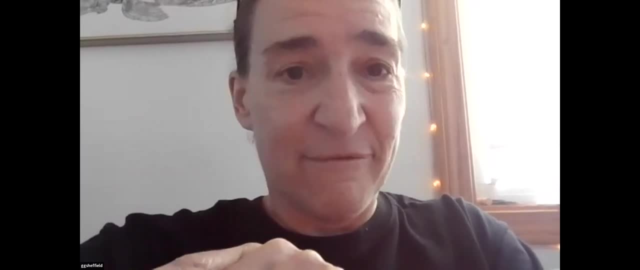 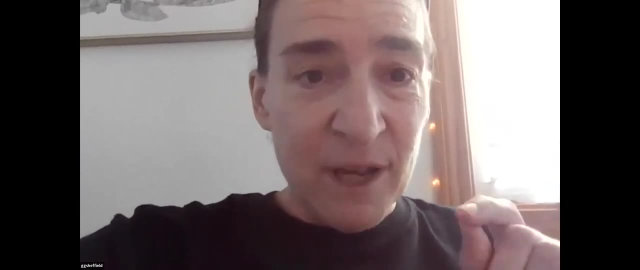 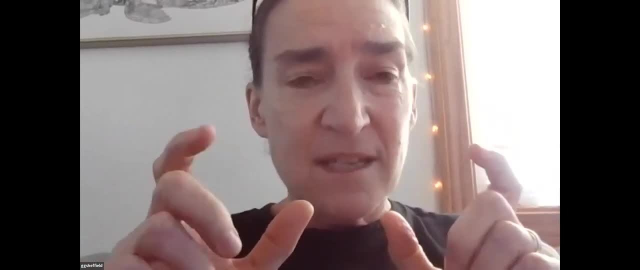 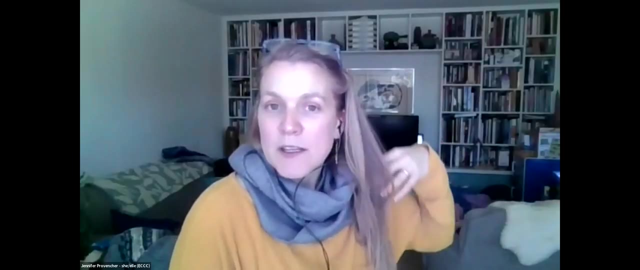 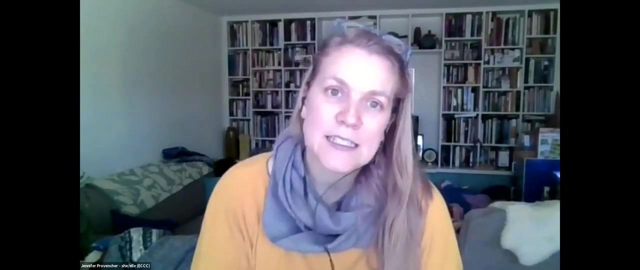 Seals the amount of contaminants. does that have anything to do with the body size? It's corrected for mass. I think it has to do with the accumulation, I think the seal. So we have another project that I didn't include here on walrus. We've just looked at 60 walrus over. 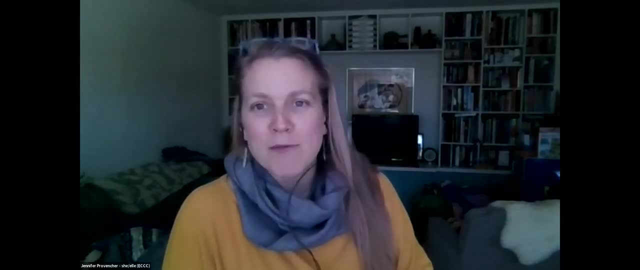 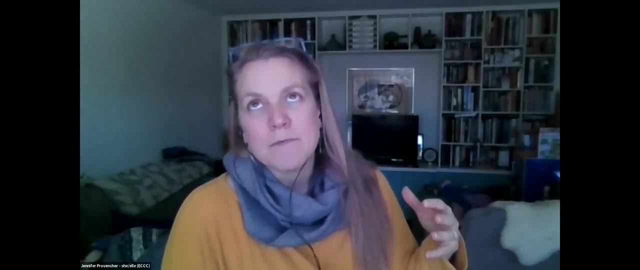 five communities in Nunavut And same story: no plastics but plastic additives. So the walrus and the seals are telling the same story. You know kind of over and over. But one thing I would put out there is: you know, Peter put up that map that. 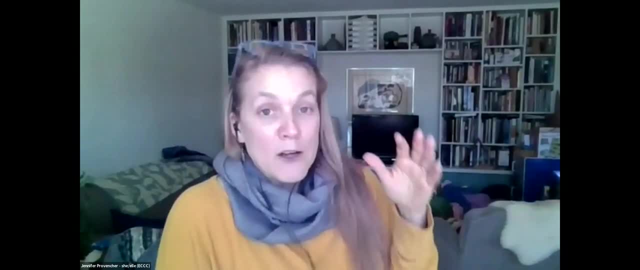 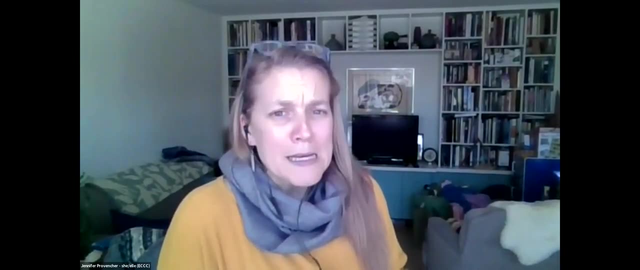 has all the freshwater inputs. We also have a project that's looking at the freshwater inputs of plastics. So we're looking at plastics along the McKenzie And I think that's another piece that you know is really understudied. What's this freshwater? you know input, And so I have 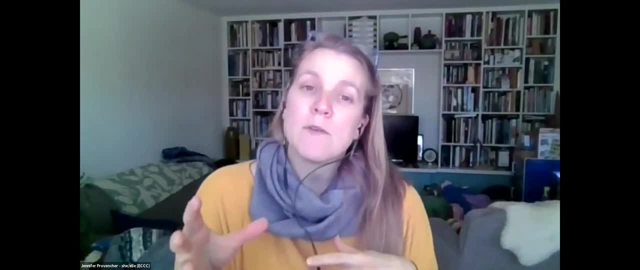 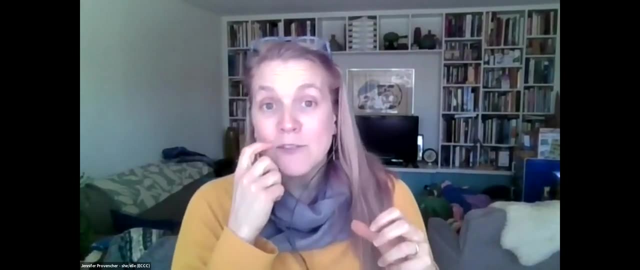 a student looking at freshwater and I have a student actually working on arctic char And we think again: those are two big pieces that you know communities are interested in knowing And has that you know management implication right? Is it coming down the rivers or is it? 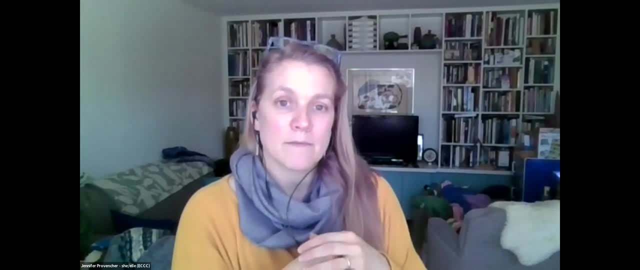 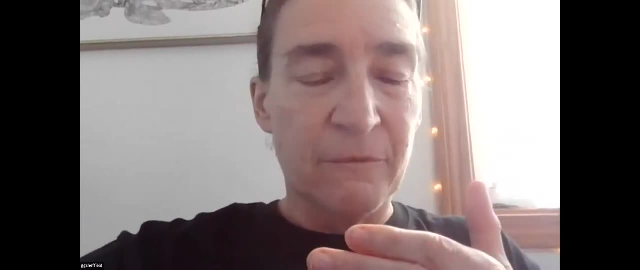 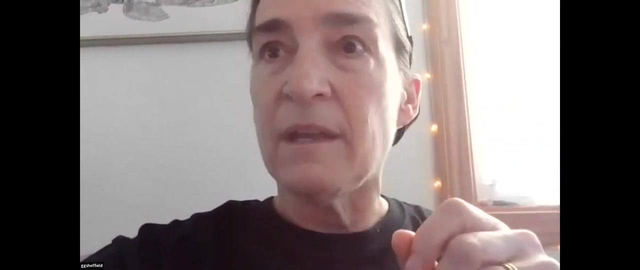 coming across the current And we don't really know the answer. Last thing, in that foreign marine debris event, because you're not seeing the plastics but you're seeing contaminants. We had bottles that had toilet bowl cleaner that had you know WD-40, Korean, We had you know. so there's. 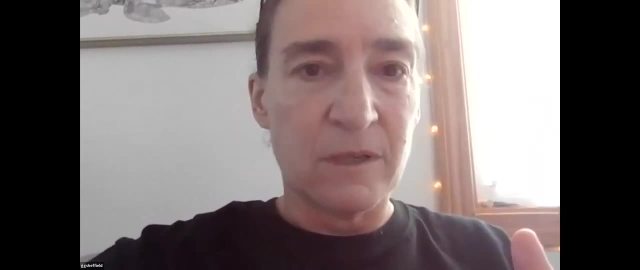 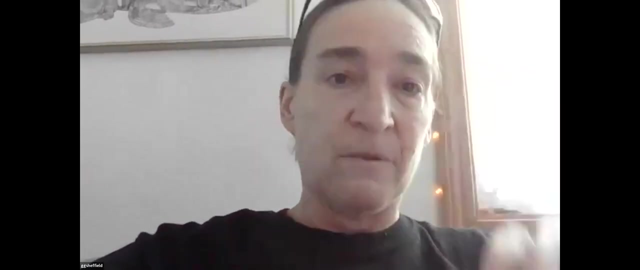 plastics. but then there was just hazmat. You know, there was roach, insecticide aerosol cans, spray paint cans, still with material in them that you could squirt out. So anyway, I'll leave it there, but something to think about It was. 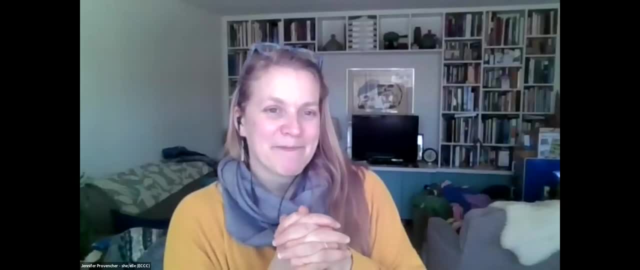 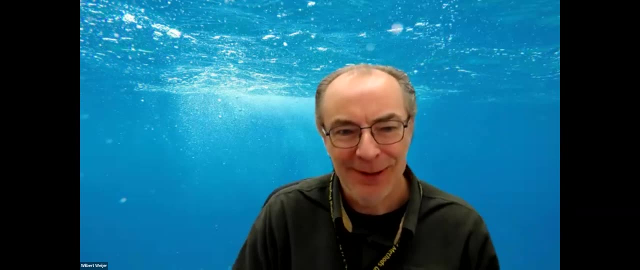 not nice. Yeah, So thank you for what you're doing. Oh, thank you all. How about one more question from Danielle And then we'll close up shop? Sorry, just real quickly, and I think we could go forever with this conversation. It's been. 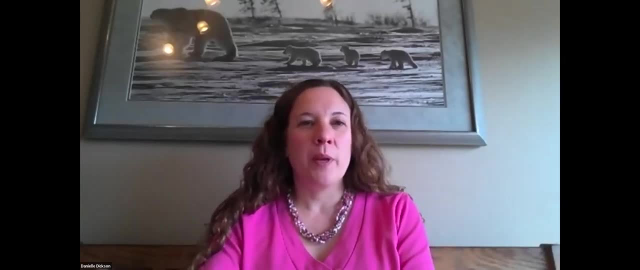 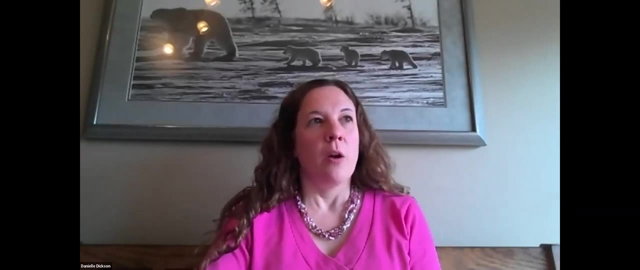 really wonderful. So many interesting facets of it. Because this, this webinar, was mostly organized by the physical oceanography team. I just wondered. you know we've talked a lot before our teams about opportunities to validate physical oceanographic models And I wonder for the physical oceanographers on the line whether folks are 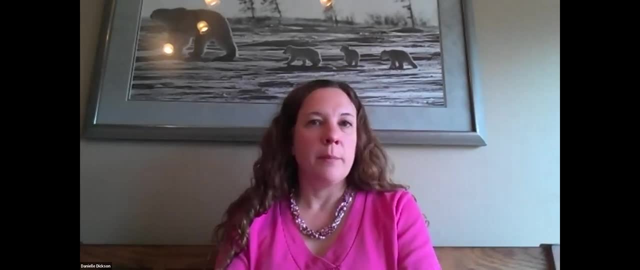 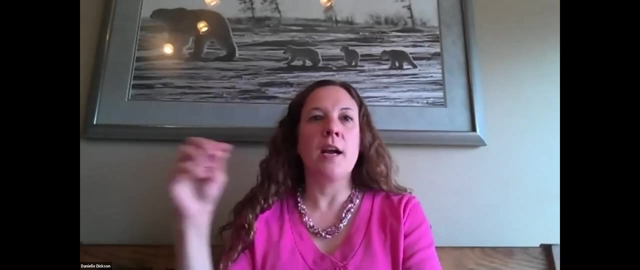 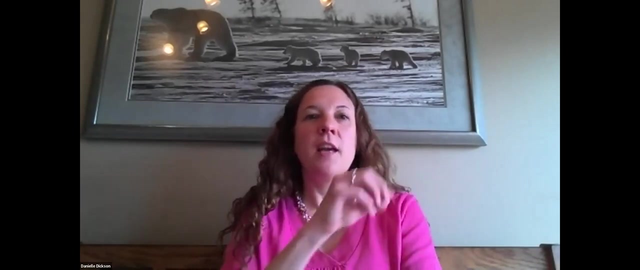 have thought about using the satellite imagery potentially of identifiable marine debris to look at, tracking it over time and use that to validate surface current physical oceanographic models, Because they, you know, if you could, I know satellite imagery in the Arctic can be quite, quite. 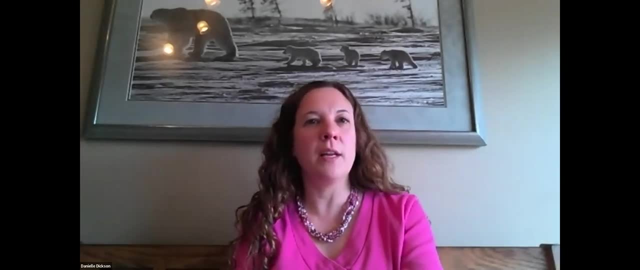 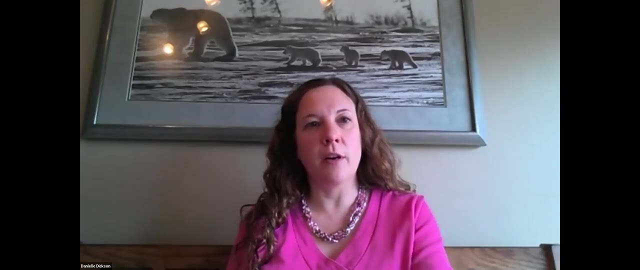 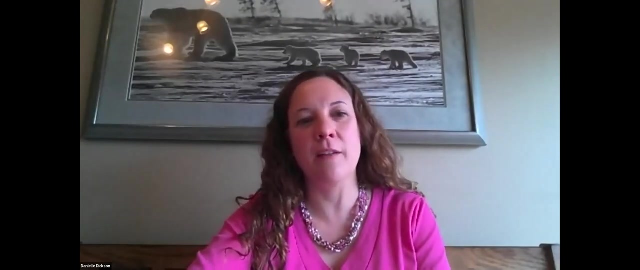 challenging And you'd probably need some pretty unique collection of debris to you know, identify it and track it over time, But that there might be an opportunity there for a semi-natural tracer to validate models. I just wonder if folks are doing that and whether the satellite folks at NOAA 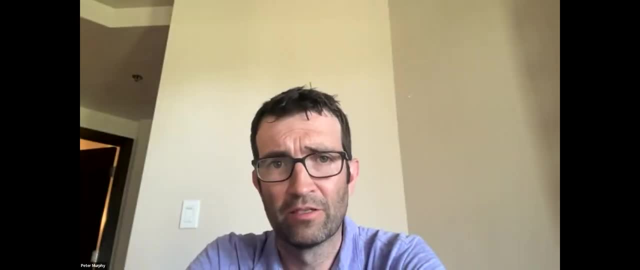 might be able to help with that data. Yeah, I can take a stab at that, I think So. actually, that's one of my other. we're a relatively small team And so each of us wear a few different hats, So one of my other. 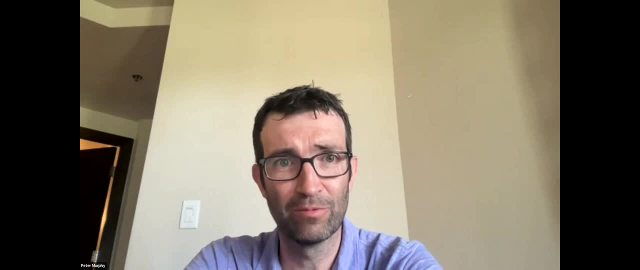 areas I work on is remote sensing. I'm not a remote sensing expert but I try to keep an eye on kind of where the technology is. It's kind of one of my topic areas. Anyway, short answer is: I think that there's been a lot of work. there's a lot of ongoing work around the use of satellite. 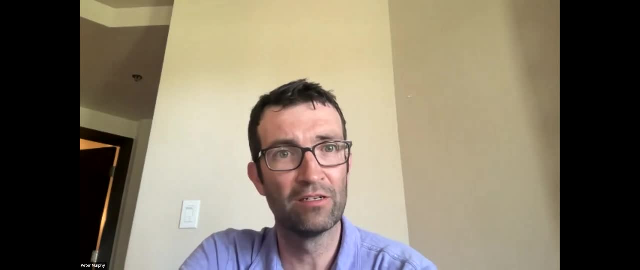 data. Oftentimes, marine debris is just too small and doesn't present a clear enough target in when it's in the marine environment to assess it, So I think it's important to look at that as well. Yeah, I think it's important to look at that as well, So I think it's important to look at that as well. 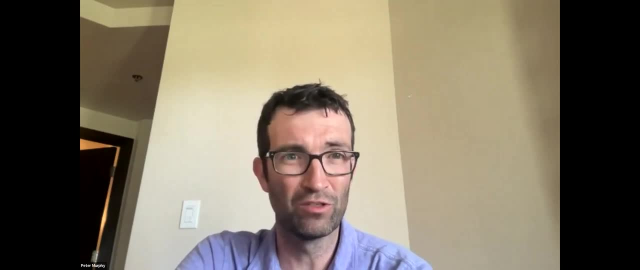 So I think it's important to look at that as well. So I think it's important to look at that as well- To a satellite sensor to be picked up or to be. also one of the big issues within remote sensing, of course, is the difference between detecting like is something there and then identifying. 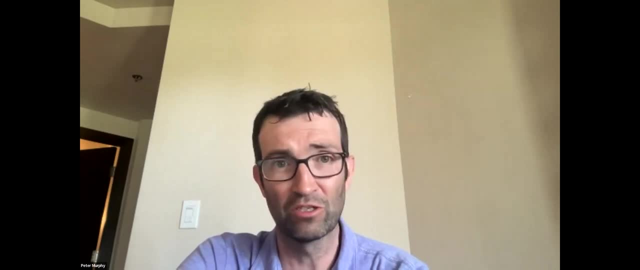 Are you able to differentiate that item from other potentially naturally occurring phenomena or items that aren't marine debris, So anyway? so I think the short answer is not. it's an area of effort, but there hasn't necessarily been a success in the Arctic yet, But there's emerging. 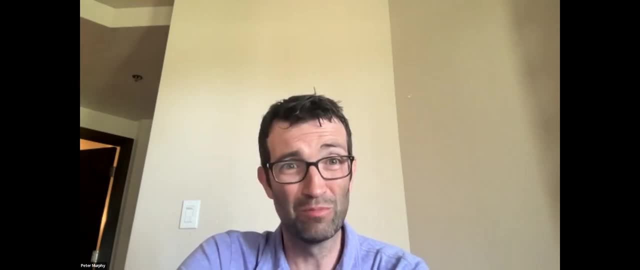 effort. there's been works out of Europe. there's been work with NOAA, certainly, So it's actually a group that meets weekly. So I think it's important to look at that as well. So I think it's important to look at that as well. So I think it's important to look at that as well. So I think it's important. 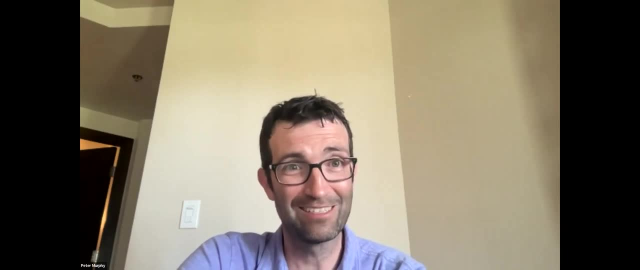 still continues to talk about this topic of using satellites to look for marine debris, And so I mean there's an active area of focus, but no one has found that solution or that answer or to be able to do it reliably for ground truthing at scale yet. But I'm optimistic. 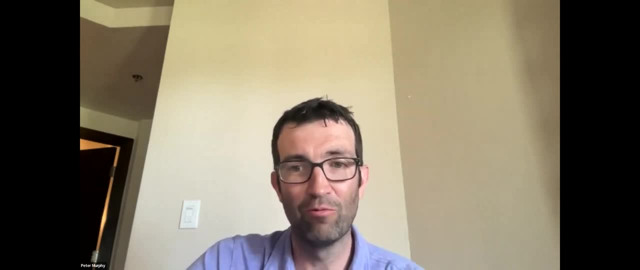 that someday that will occur. It's just a question of figuring out how that will, what that will look like And you know what that may be, And I think that, as people are providing links in the chat, I think it's a lot of it is looking at. 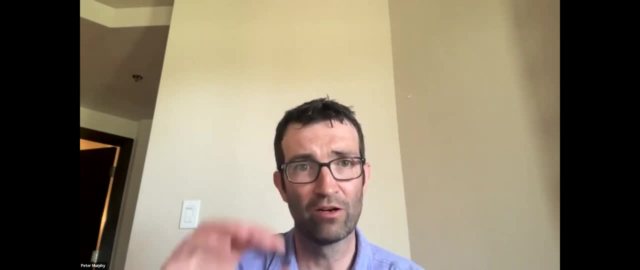 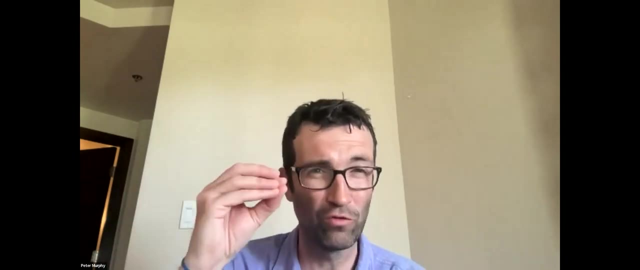 the detection, using algorithms to and other methods to try to tune machine learning to try to find debris, and also, because that's one of the big issues- is post-processing, the time it takes to try to look for and tease out these items. i think the short answer is: area focus definitely. 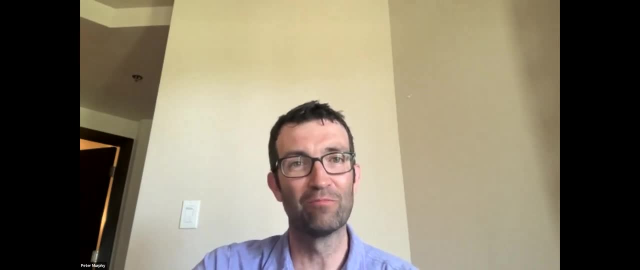 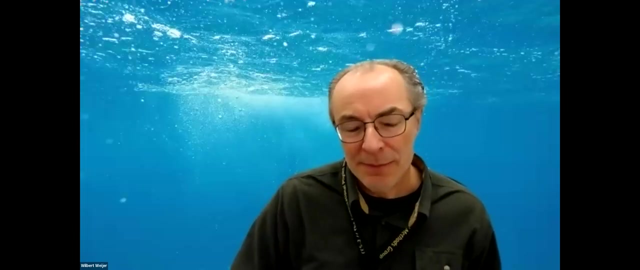 people working on it, um, but it's. but we don't have a satellites, aren't yet at a place where they can replace um in situ data collection, um from you know an aircraft or other other sources. yeah, i would just back up peter on that one. it's exactly what i say. people are working on it. so if 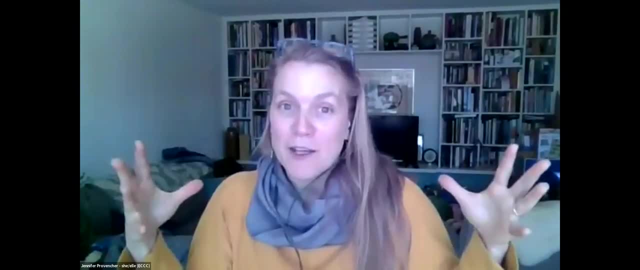 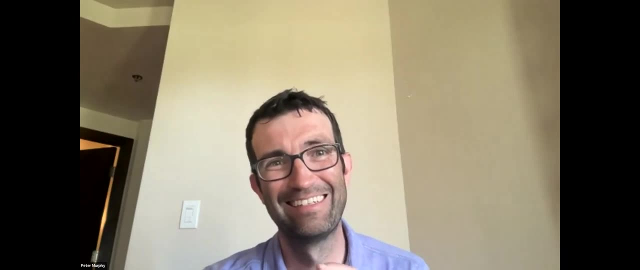 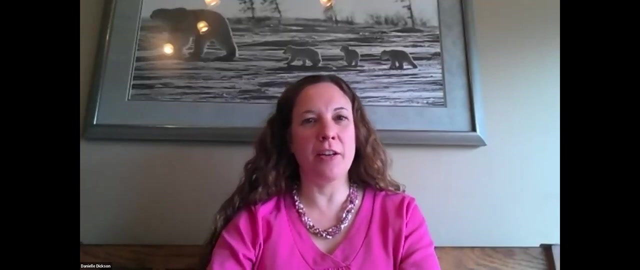 you've got you, if you've got kind of um expertise in that field, like come, come play in the plastic seems like maybe, uh, you know, a dual use case for some like dod groups, like office of naval research that are interested in verifying what currents are doing in the arctic, and you know. 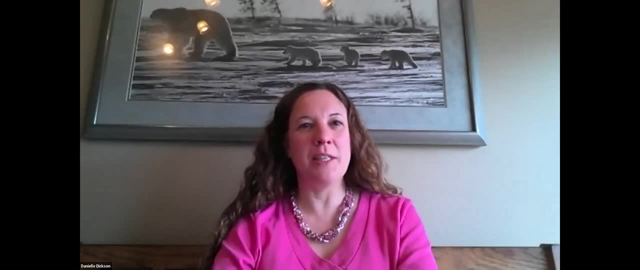 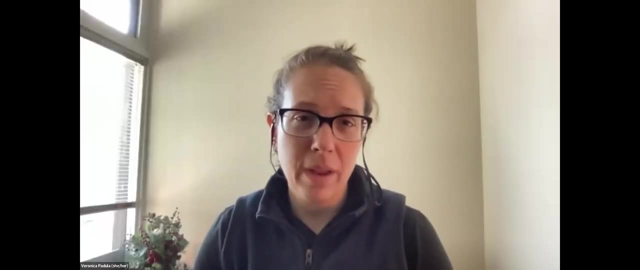 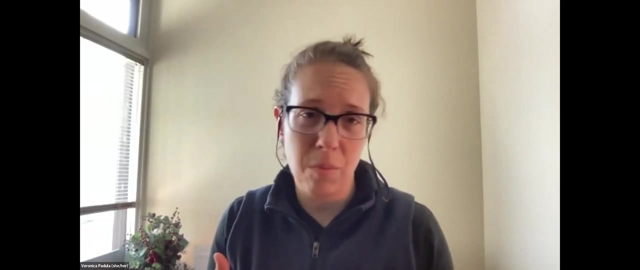 connections to high-res satellites data. maybe we can pull dod. yeah, i would also say coast sorry, oh, go ahead. oh no, we had some luck with working with coast guard out on st paul ii. there are definitely champions within the space that like care really deeply about marine debris and like we had a team of 15 folks when the, when their. 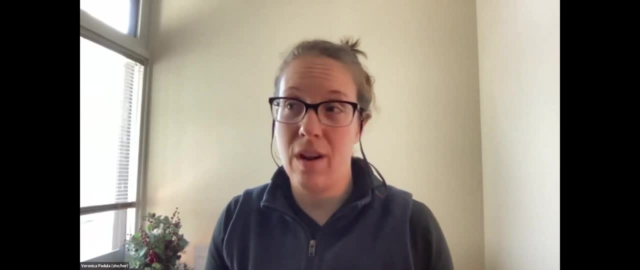 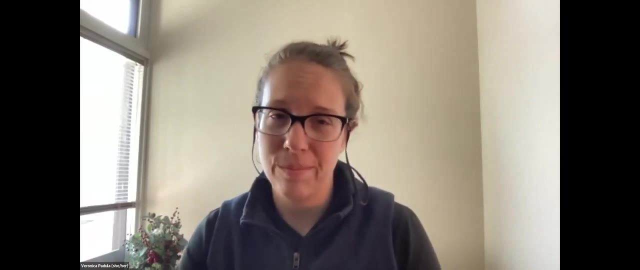 uh vessel was in our harbor that came on island and helped us remove like a several thousand pound net because we just couldn't do it with our own resources. so, um, just putting it out there to think about like coasties as well, because they can be very helpful. 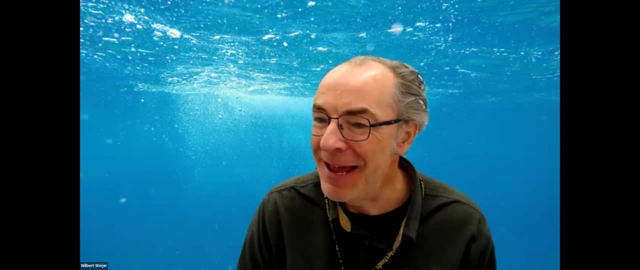 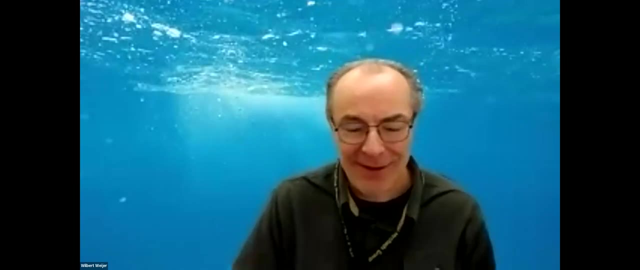 awesome. very nice discussion everybody um. so maybe we should um stop here and thank you very much, jennifer and peter. very insightful uh presentations. it opened a new world- for me at least- um into all the issues that are involved with uh, with marine debris, um and and their and their impacts. it's pretty staggering um so. the physical oceanography team. 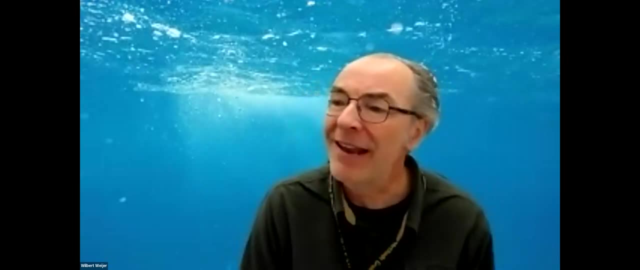 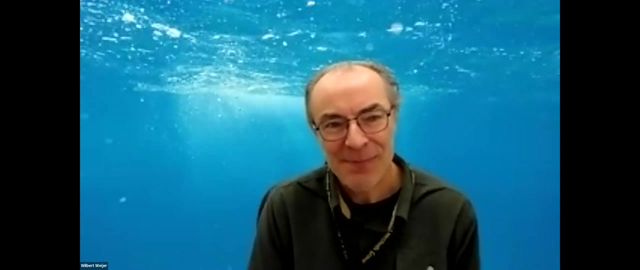 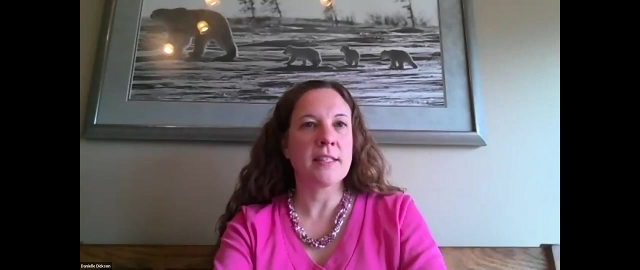 has a next meeting at june 2nd. we're still working on that. i don't know if the marine ecosystems team has anything planned in the near future that they want to advertise. we're- uh, we usually meet the um second tuesday of every month at 10 am alaska time. 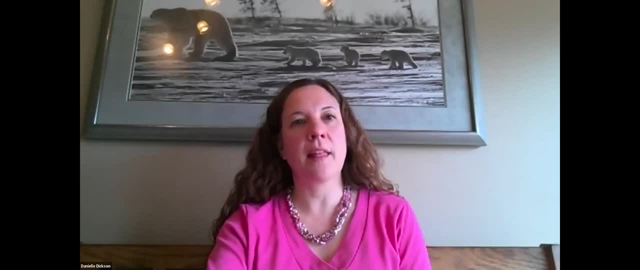 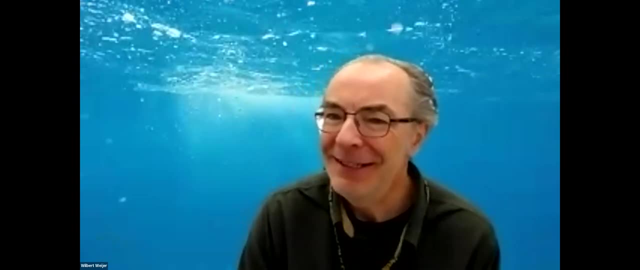 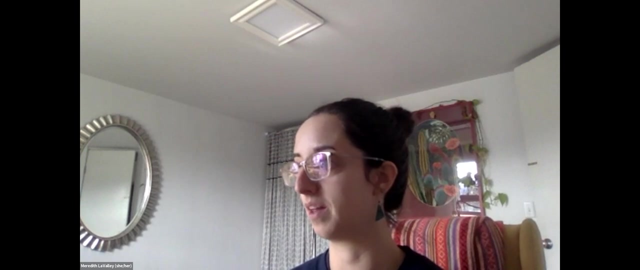 um, so keep an eye out for our agenda for june. i think we're still firming that up. thanks, great thanks, um, meredith. anything else for you too? um, just that. this recording will probably be posted by the end of the day today. um, as well as, uh, the, i will post um some brief notes and the resources that have been dropped.